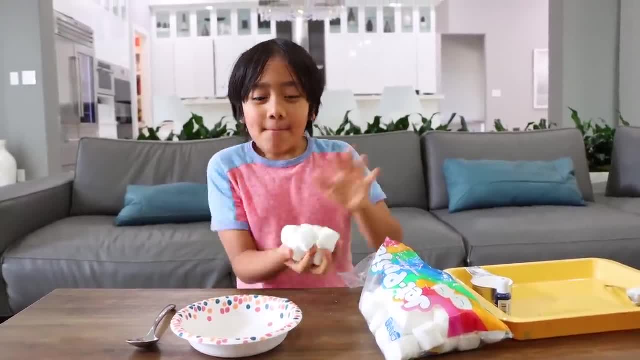 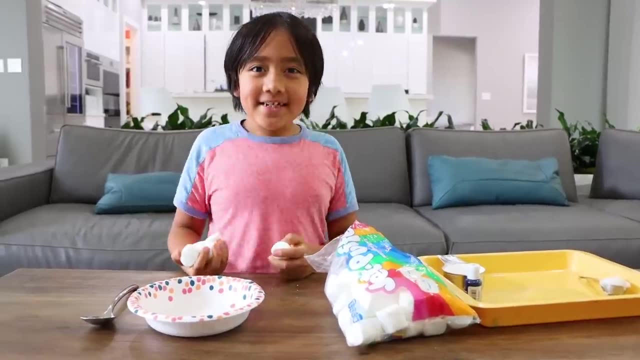 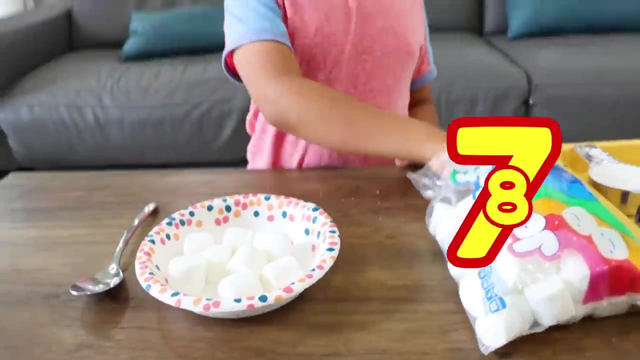 Hey guys, today I'm going to make a homemade play-doh with marshmallows. First thing you're going to need is marshmallows. Here I'm going to use 10 marshmallows- Five already- six, seven, eight, nine and ten. 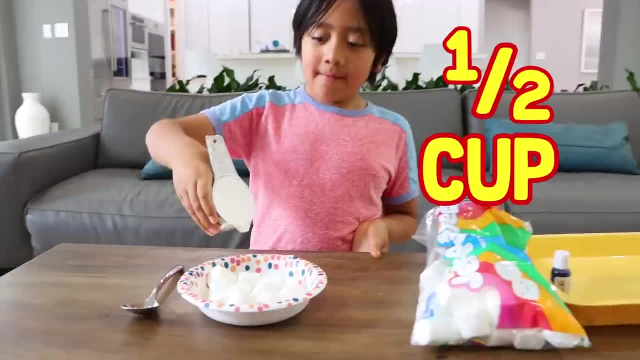 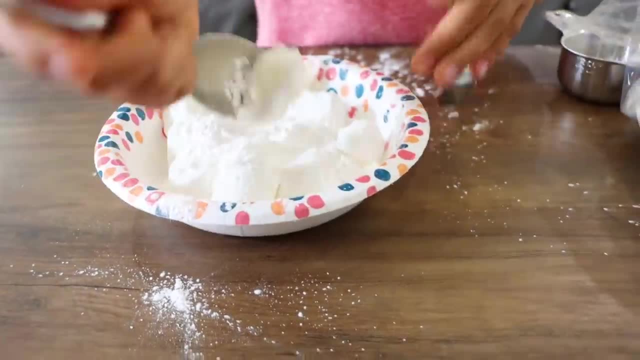 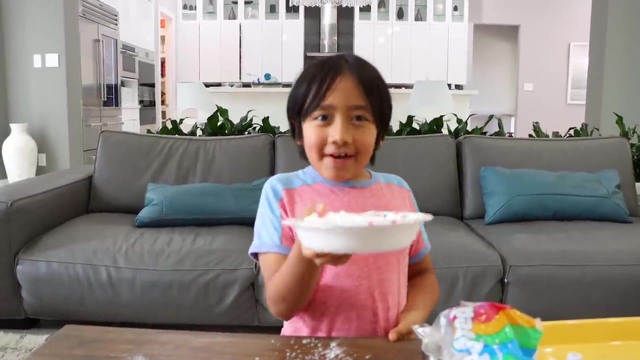 Next thing you need is half a cup of cornstarch. Next is one tablespoon of coconut oil And there, Next thing, ask a grown-up to microwave this for 30 seconds. Mommy, can you microwave this for 30 seconds? Of course, Ryan, I'm right here. 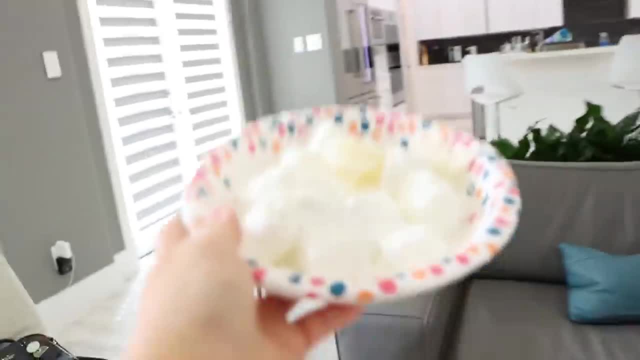 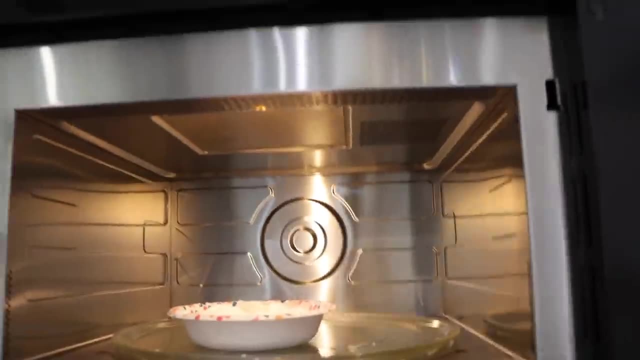 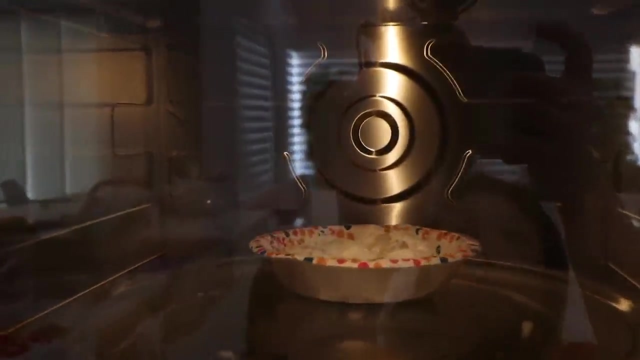 Thank you, Be right back. Okay, taking this to the microwave: Okay, Microwave 30 seconds, Okay. And if you look here, notice what happened to the marshmallows when you microwave it, The magic's gonna happen. Oh, I noticed what's happening. 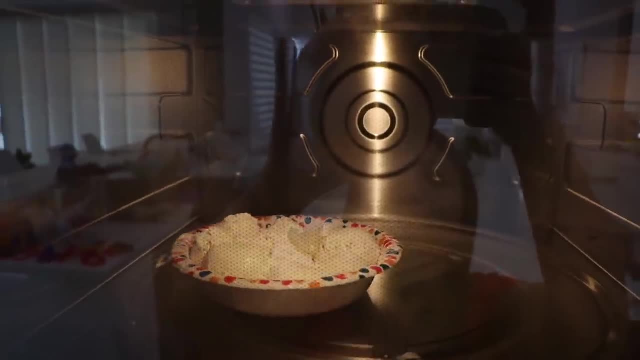 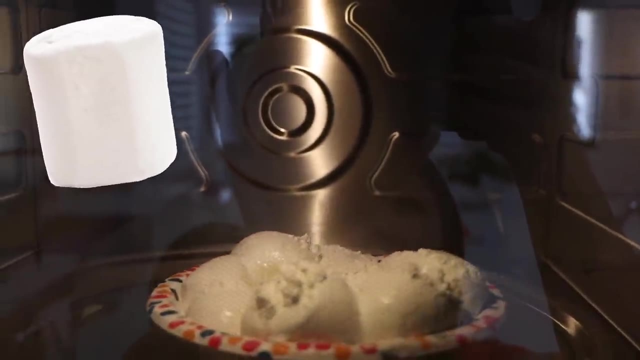 What It's spinning. But what's happening to the marshmallows? Did you notice it got bigger or smaller? It looks bigger, Do you see it? It's a giant-sized marshmallow. Oh, that's 30 seconds, Okay. 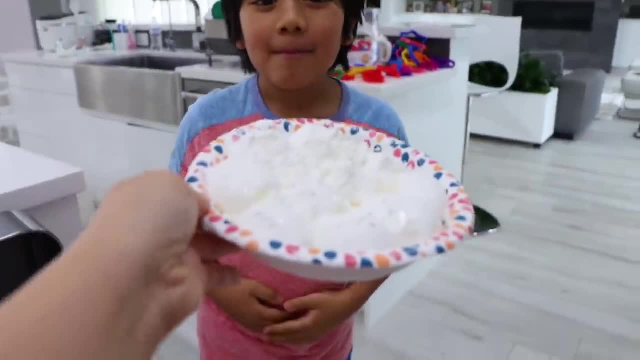 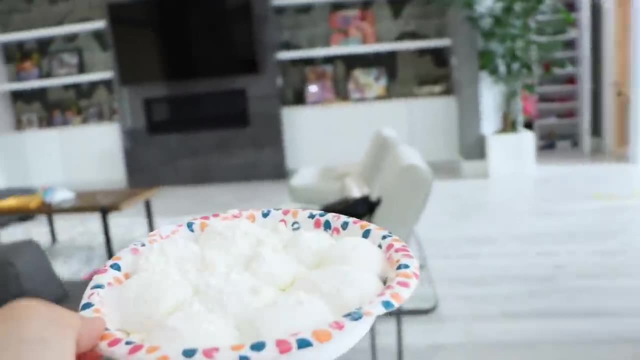 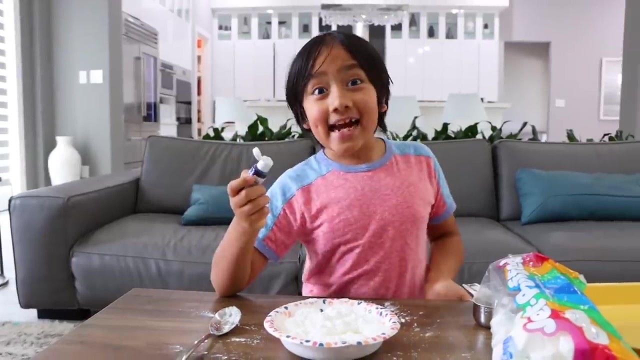 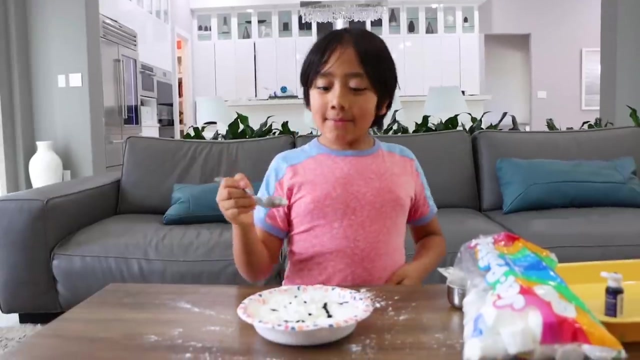 Yeah, Okay, Look, Whoa, Do you see it? Okay, Let's bring it over. It smells like, uh, s'mores. It smells like s'mores. Yeah, Next, add some food coloring. Now I'm going to agitate the blue food coloring with the blue food coloring. 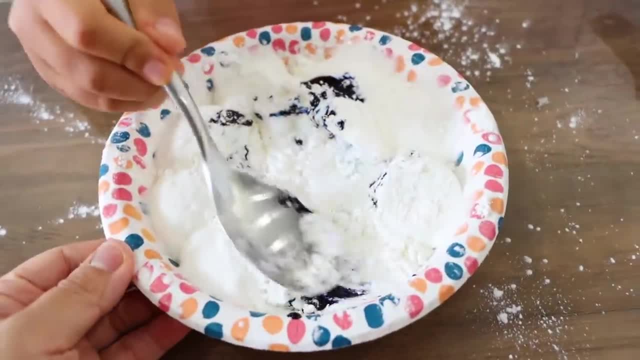 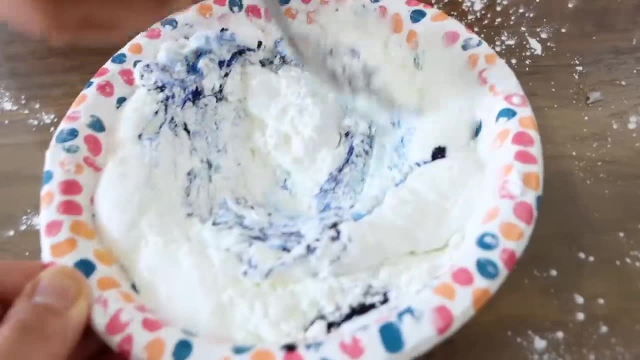 The marshmallows? Okay, I'll hold it for you. Whoa, Okay, Exactly like mixing s'mores It does. huh, It looks kind of cool. Mix it all up, Mix it all up, Agitate, Agitate. 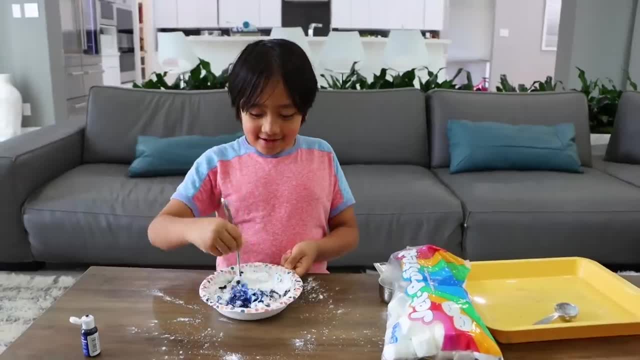 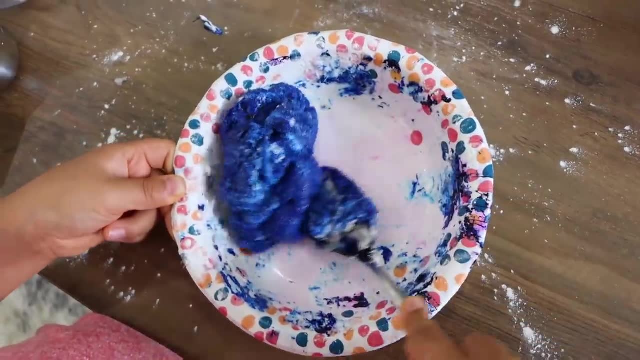 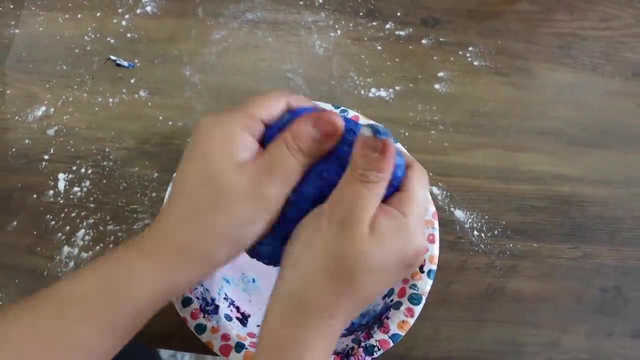 What's another word for agitate? Mix Or stir? Good, Okay, Mixing, Almost there. Good job, Get almost fully blue. All right, Now it's a little warm, so mommy's going to take over, But all you do is just smush it together like so. 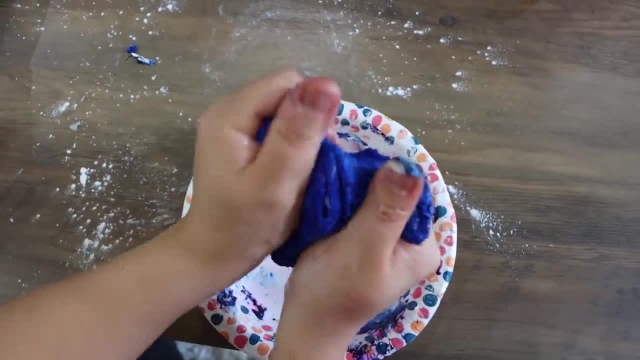 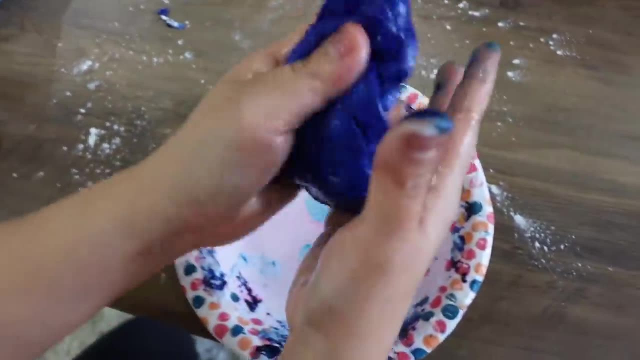 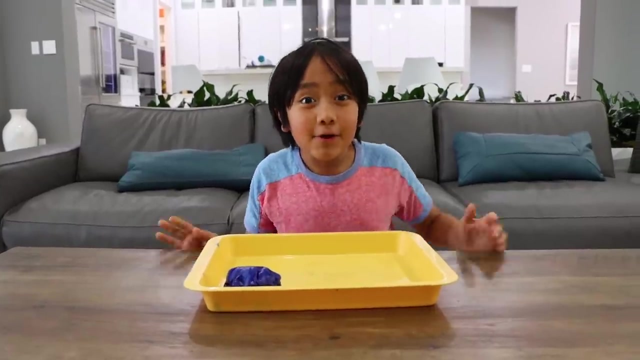 Whee, Looks like it's starting to look like Play-Doh. Look, Ooh, And then just, you can even roll it and twist it. See Woo-hoo, Now that we have our blue Play-Doh, let's make the other colors. 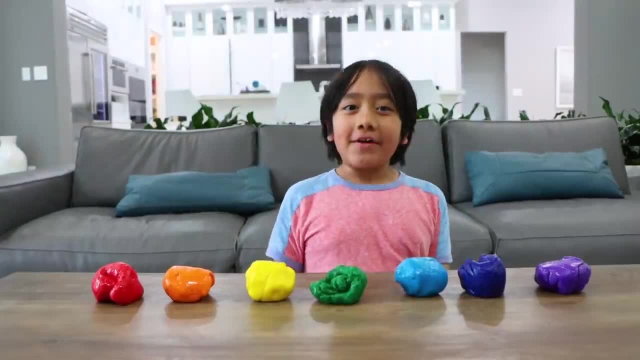 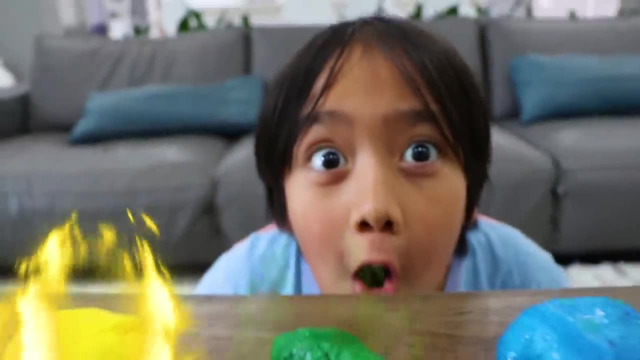 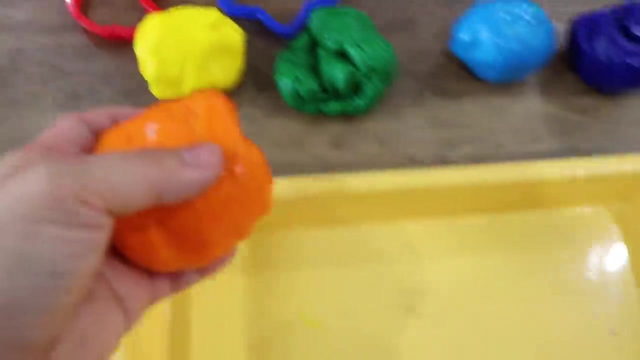 Okay, Okay, Yay, We have all the colors of the rainbow of Play-Doh Marshmallow. Now let's test it out, Okay, So first we're going to just use orange. You just press it down, Okay. 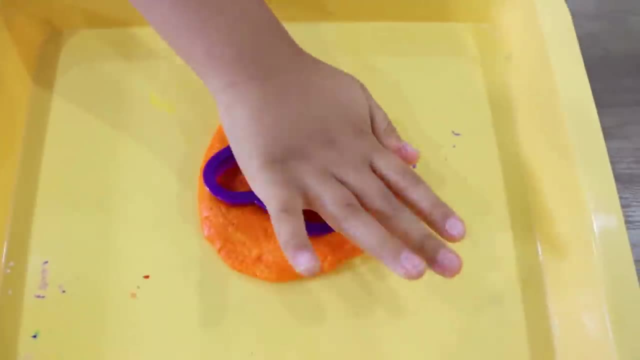 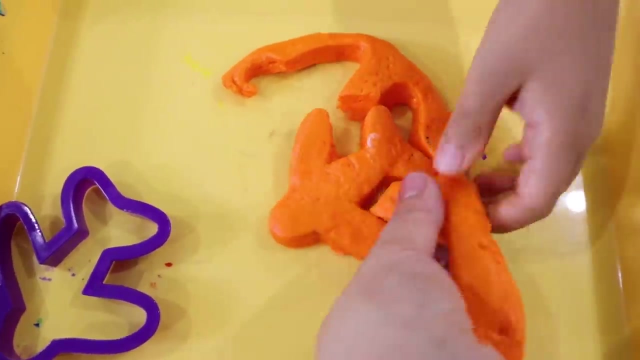 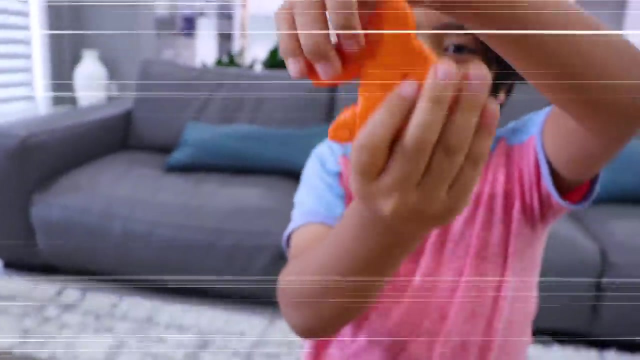 And then you put it in: Okay, And now we're going to take out the sides. Okay, Yay, Now we have an orange Play-Doh. Where are you going? Where are you going? Whoa, Whoa, Watch out. 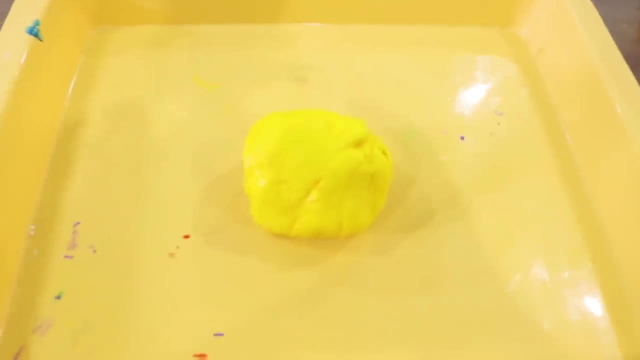 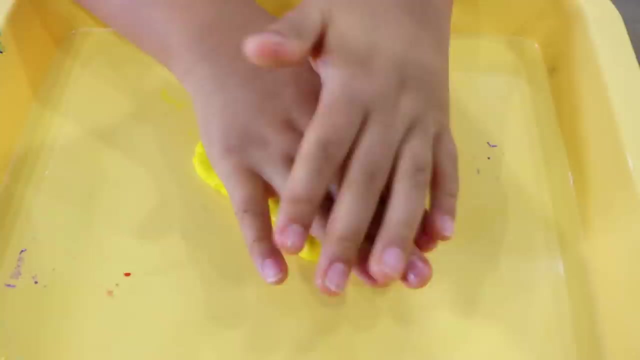 Okay, Now let's see if we can make a star. Okay, Let's see if that fits, Okay, And a yellow star: Okay, Push it in. Okay, Push it in. Okay, Nice, Nice And teamwork. 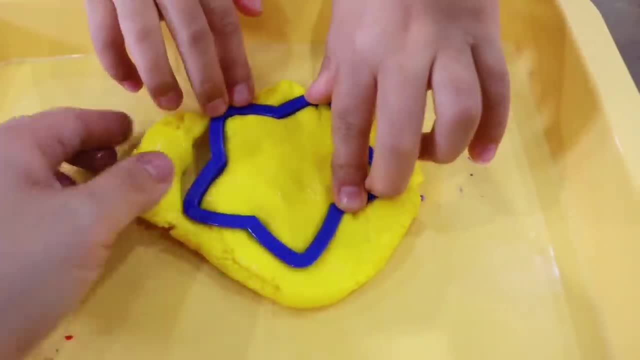 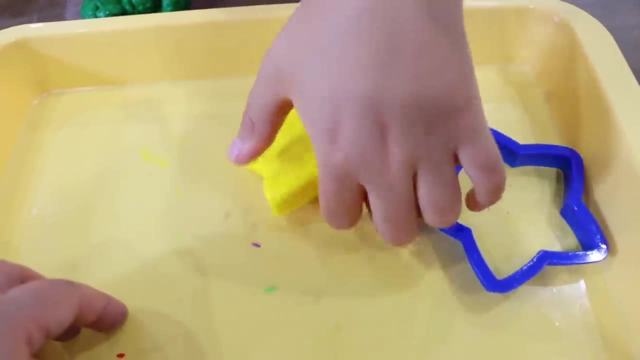 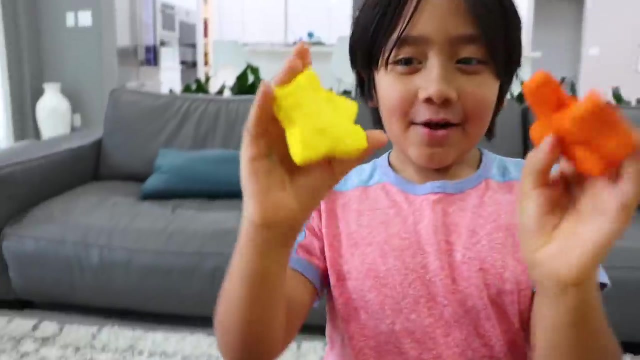 Can you hold this down? There we go, There we go, Just lift up the outside layer and, bam Bam, We got a star. Twinkle, twinkle little star. How I wonder what you are. Star plane, What do you guys wish for? 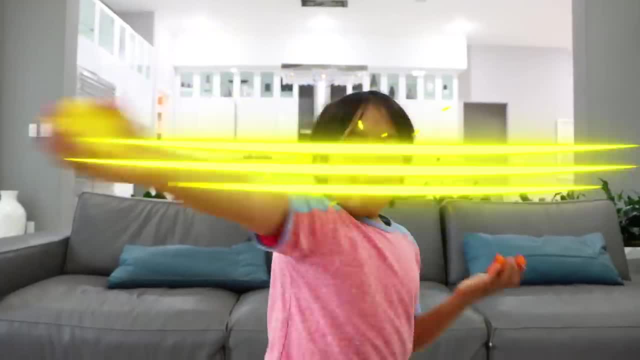 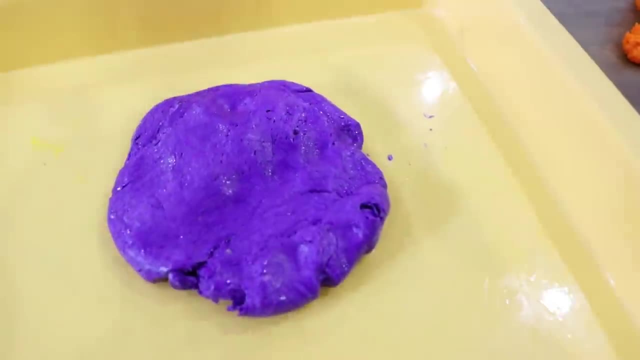 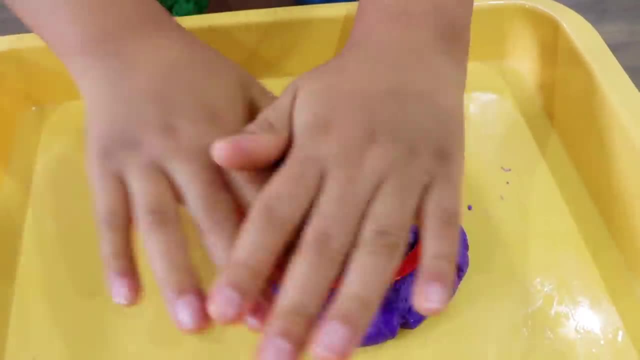 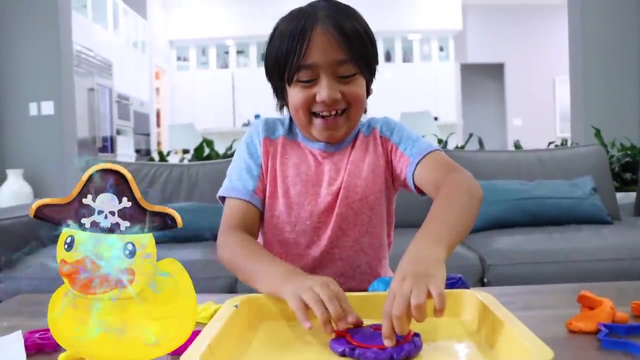 Purple ducky, Why not Plasma ducky, A plasma ducky. What is a plasma ducky? It's a ducky. that's plasma, Oh Fancy. All right, Let me take out the sides. Whee, There we go. 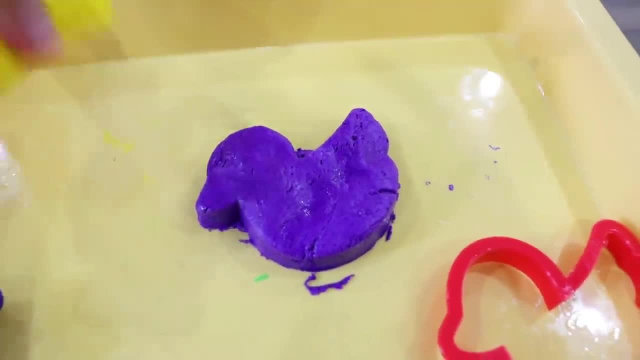 Do we have a ducky Yay, We have a ducky Yay. Star star, ducky star, ducky plane. Star star, ducky star, ducky plane. Now let's make a rainbow play-doh tower. 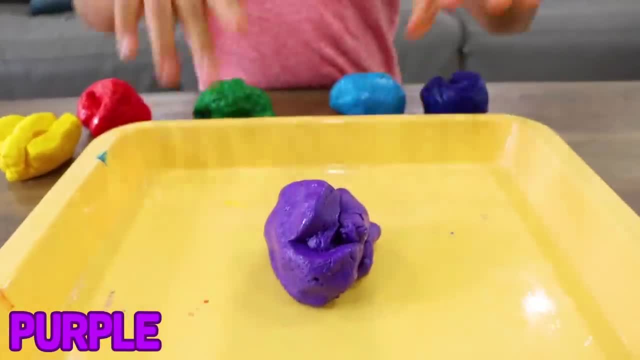 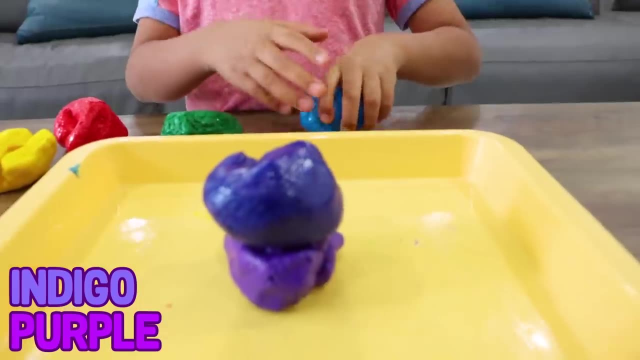 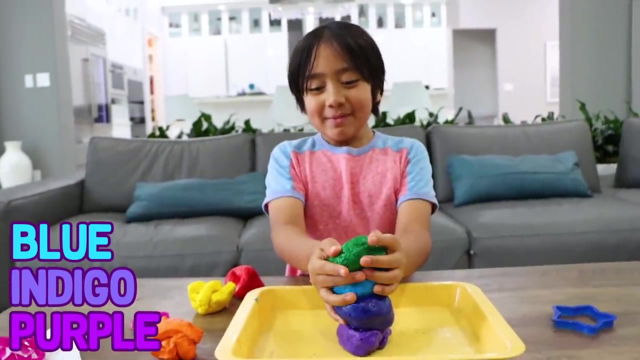 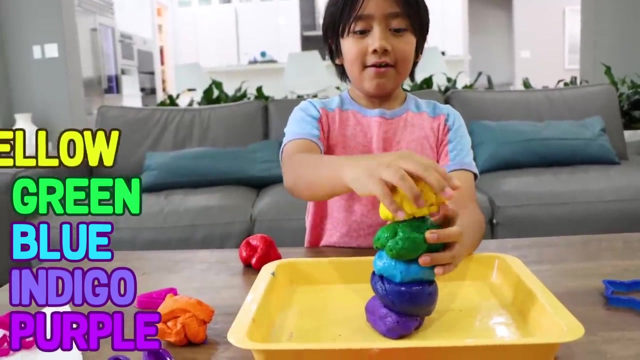 Now let's make a rainbow play-doh tower, Okay, so purple And indigo, There you go, Just smash, smash, smash, Then blue, Then blue, Blue, This might fall already. Green, Okay, Yellow, Nice. 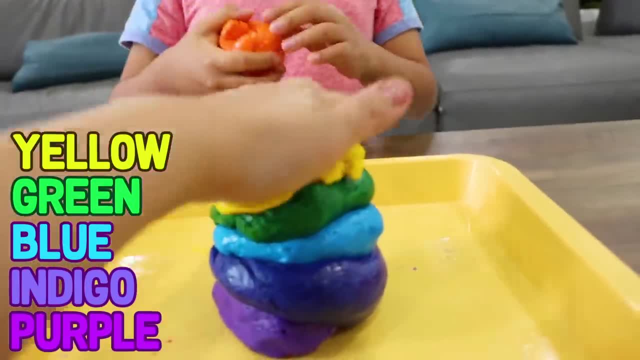 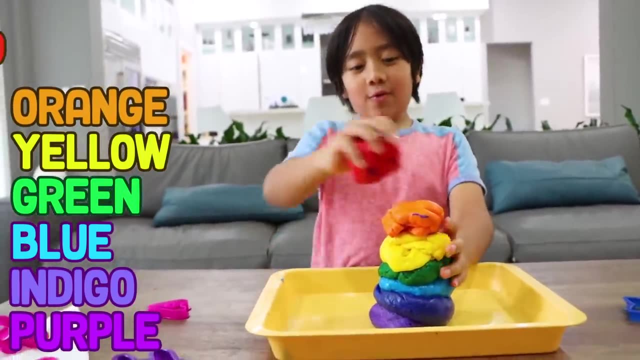 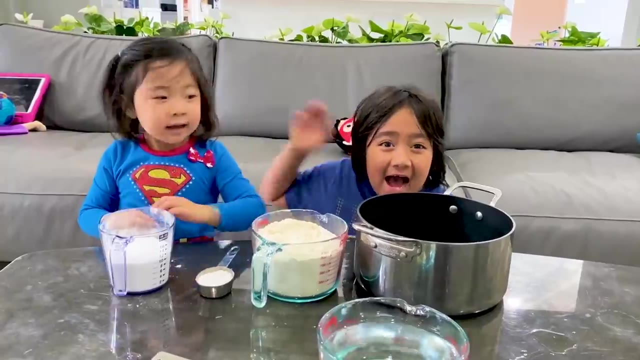 Is it going to fall? Maybe, Let's see. Okay, Orange And red: Yay, Color the rainbow play-doh. Oh yeah, Hi guys, Today we're going to be making our own play-doh, So first thing we're going to add is some flour. 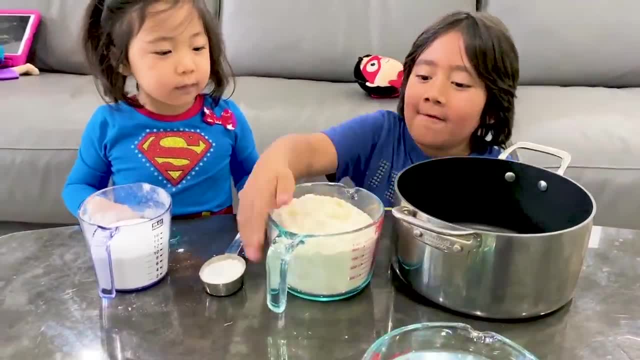 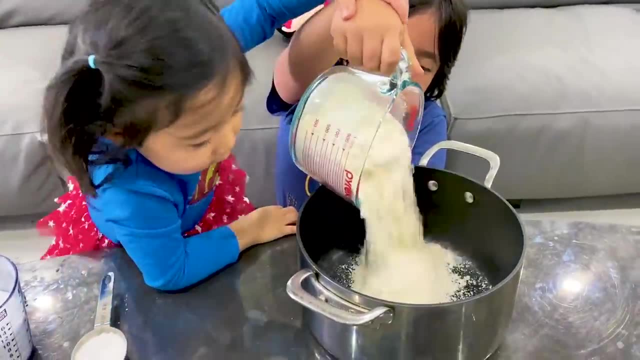 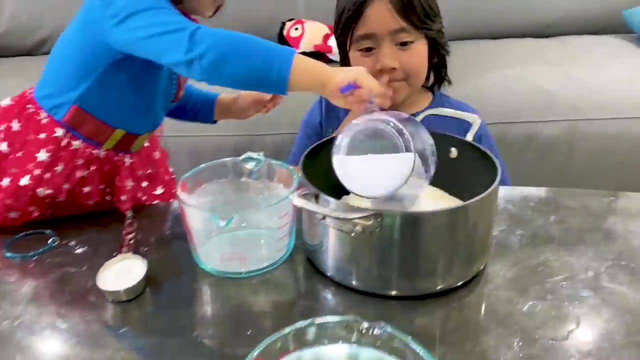 So we're going to have flour- Four cups of flour. We're going to put the whole thing in the pot. Okay, The whole thing. That's a lot of play-doh dough. Yeah, a lot of play-doh. And then that is salt. 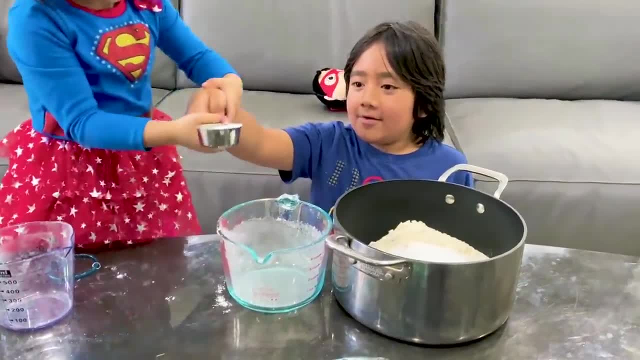 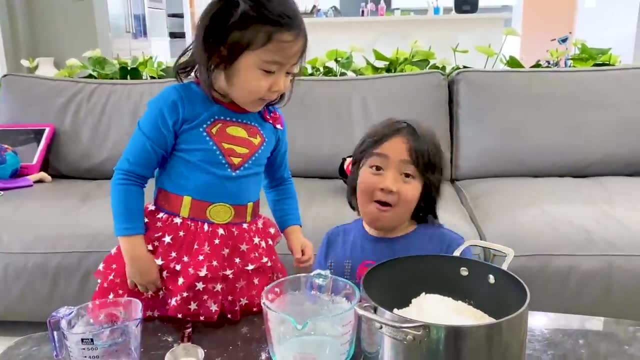 Two cups of salt, And then that is cream of tartar. One fourth cup of cream of tartar. Good, Does it look like play-doh yet? No, Not at all. No, We're going to add in one third cup of oil. 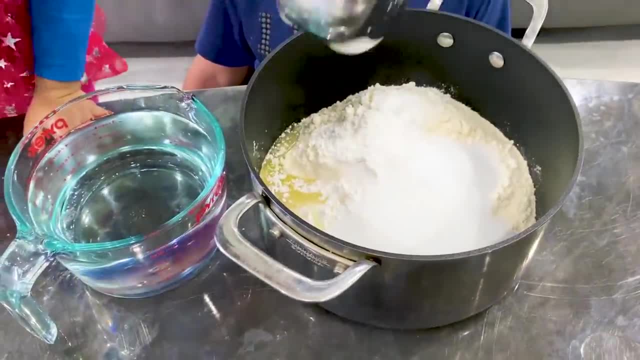 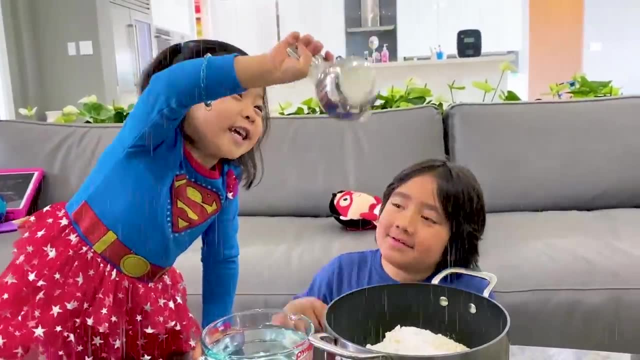 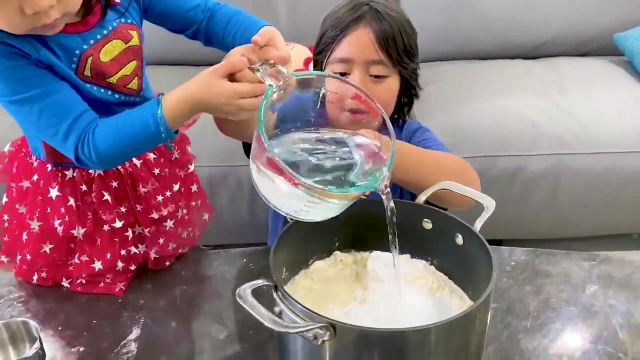 Vegetable oil. There you go. Oh, it's going to drip- It does. Now let's add in four cups of a little bit warm water. You guys got this A lot, Everything. yeah. Now does it look like play-doh. 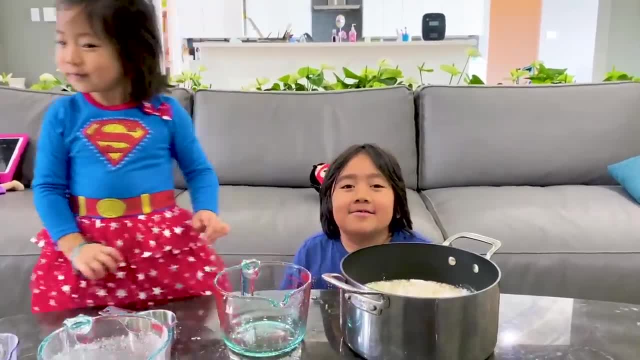 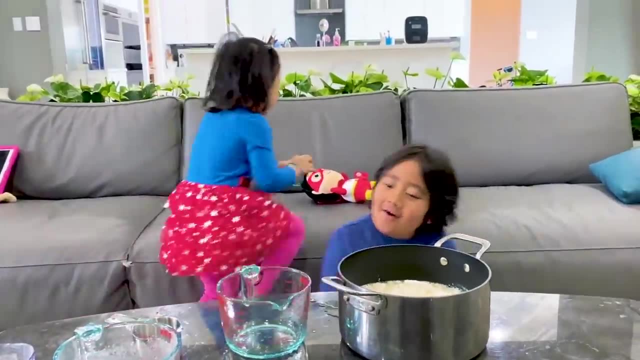 No, Okay. next step is for grown-up. only, I have to actually cook this on the oven, Okay, so we'll be right back and I'll show you. You guys go play while mommy do this part, Okay, Okay. so now I'm cooking the play-doh. 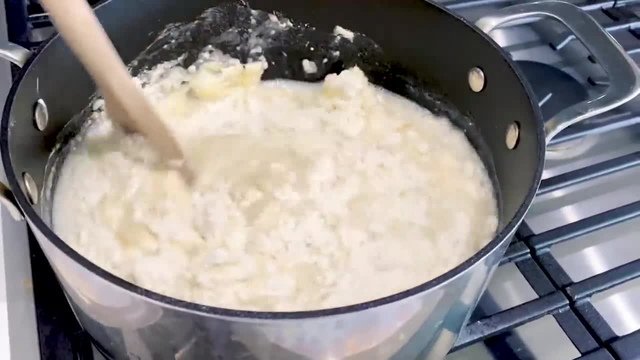 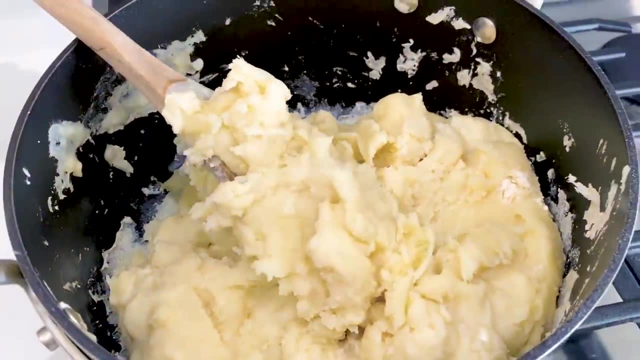 on medium heat here. Gonna just keep doing this until it hardens and thickens. Whee, Okay, I think it thickens and now I think it's ready to continue. Look. Next step, after it cools down, is just to. 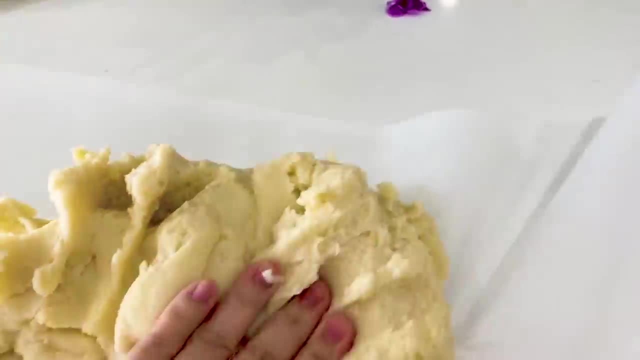 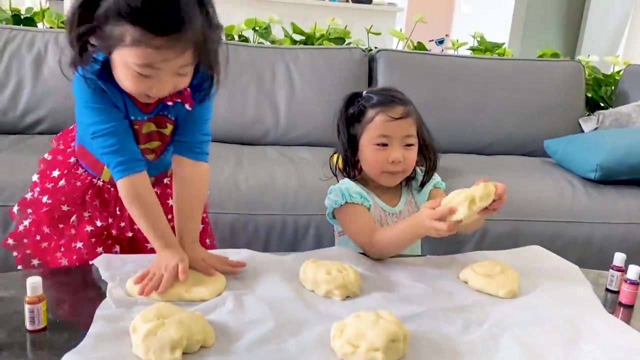 kneel the dough like the bread. Keep doing it until it's smooth. Whoo, I got all the play-doh out. Emma and Kate's gonna test it. Does it feel like play-doh? Yeah, Yeah, like play-doh. 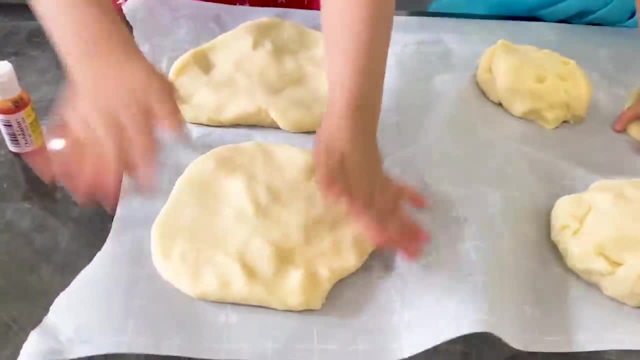 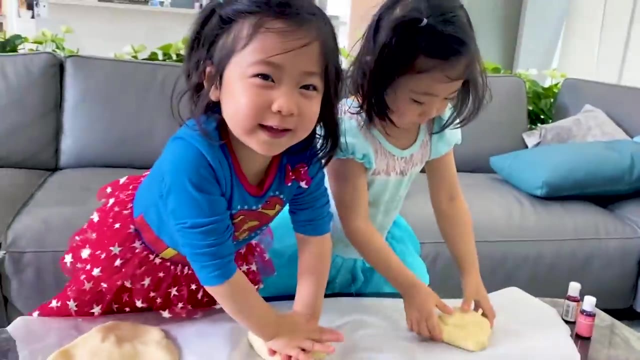 Whoa, it's like a pancake. Make it like a pancake. Okay. Emma wants to make each one like a pancake. Good idea, Oh, love it. I want to make mine like a pancake, Okay. Next step is to flatten it out. 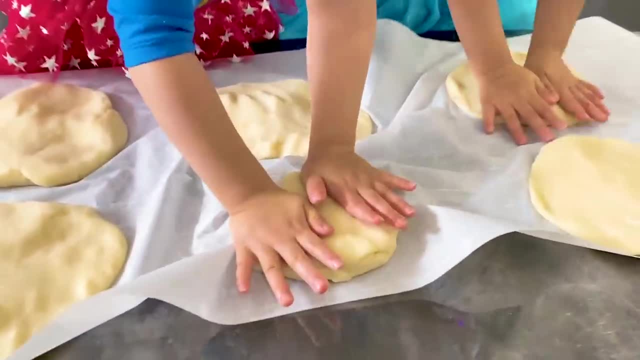 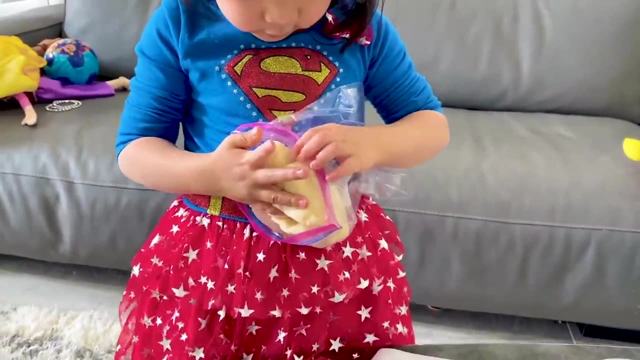 like a pancake. Emma says: There you go, We're gonna put each one in a Ziploc bag. Emma's helping me right now. Good job, Emma. There you go. like that, Good job. So now we put each one in a Ziploc bag. 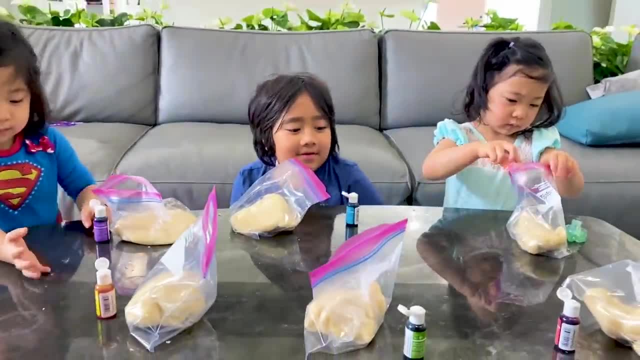 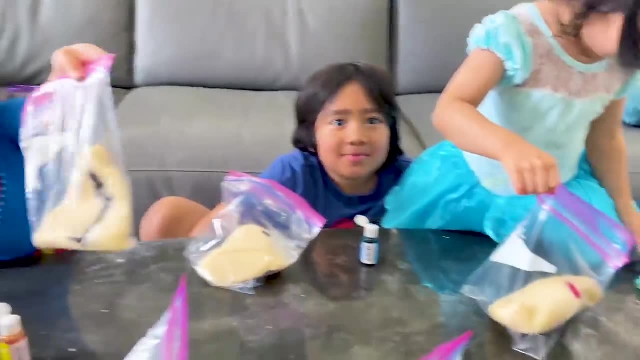 Then we're gonna add color to each one. Alright, so go ahead, Add the colors. Can I put this on first? Sure, Oh, there you go. So Emma put in purple, Ryan put in blue. You can add a little bit more, Ryan. 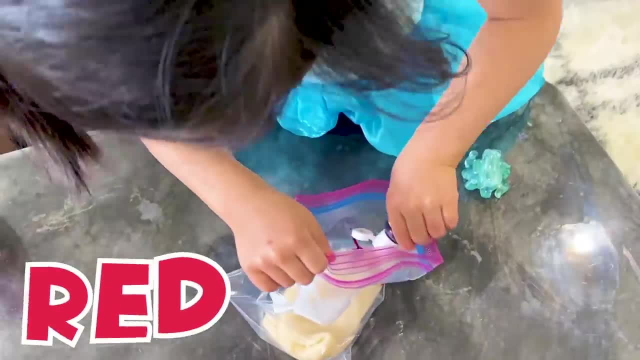 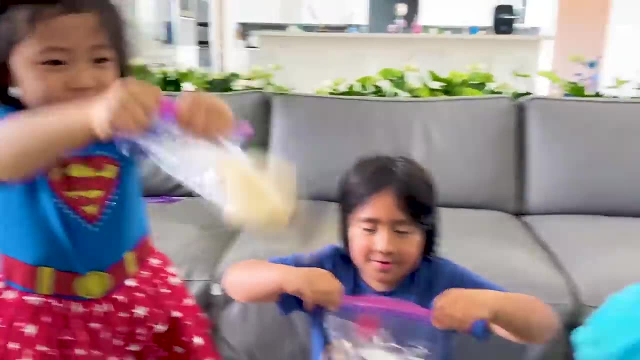 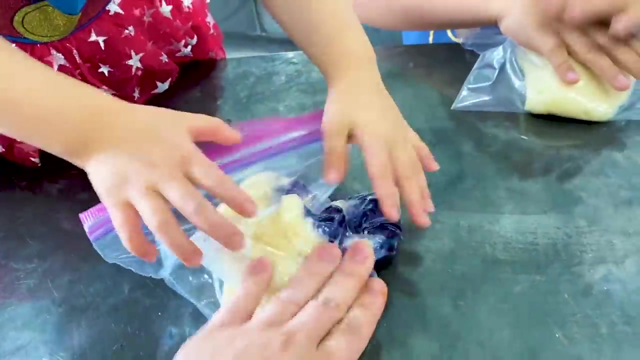 Purple And Kate added pink-red. There you go. Kneel it together on the outside. There you go. like Emma's. Not shake guys Like this, Just kneel it like that. There you go. Good job, Kate. 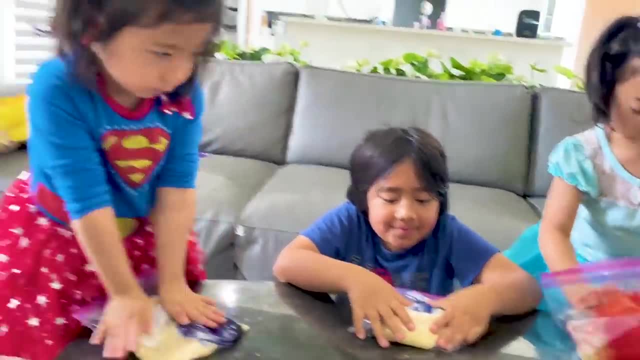 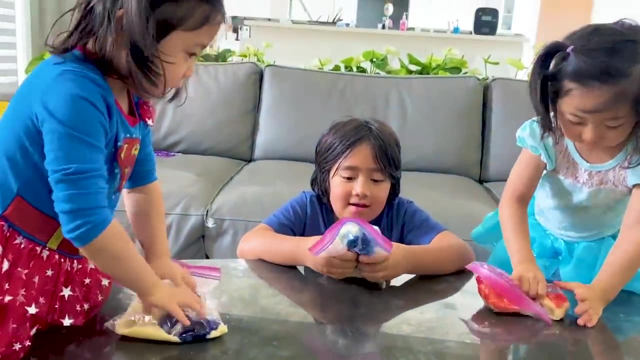 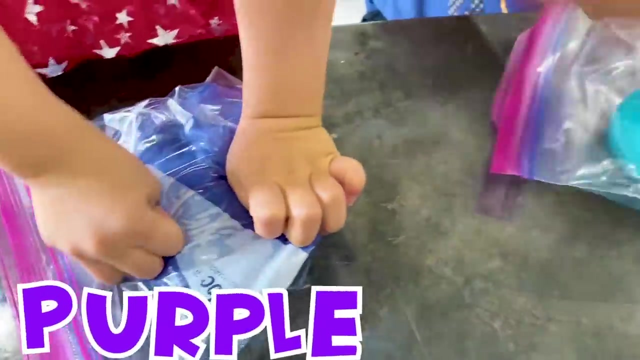 Yeah, There you go. Good job, guys. Make a pizza Feeling it like a pizza. That's right, Emma. Yours is almost done, Kate. Good job, Emma. you too. Good job, Emma. Guys looking good already. 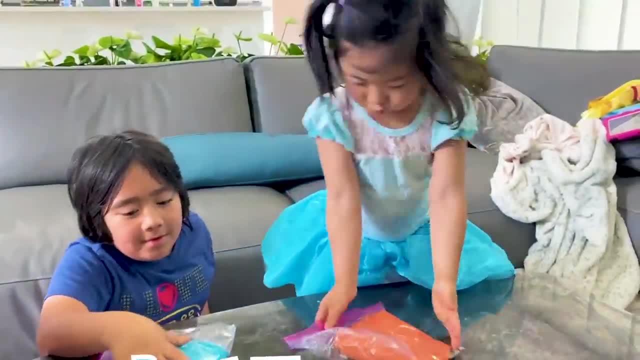 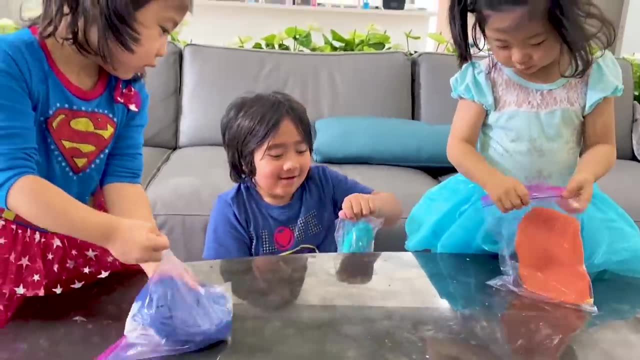 Look, it's purple for Emma, blue for Ryan, and then I thought it was pink, but Kate was doing orange. Yeah, looking good, You guys can take it out now. Actually, it feels like Play-Doh, Does it? Yeah? 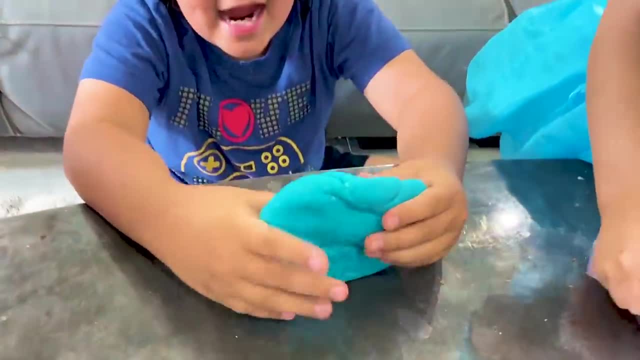 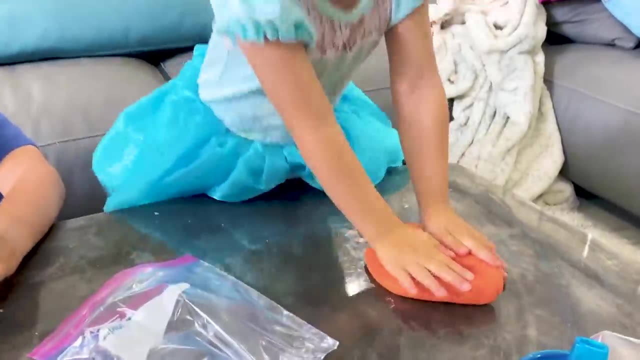 Homemade Play-Doh. We made it ourselves. Is this already Play-Doh, or is there something we need to add? Nope, it's already Play-Doh. Wow, Play-Doh, Play-Doh, We made it, It's cool. 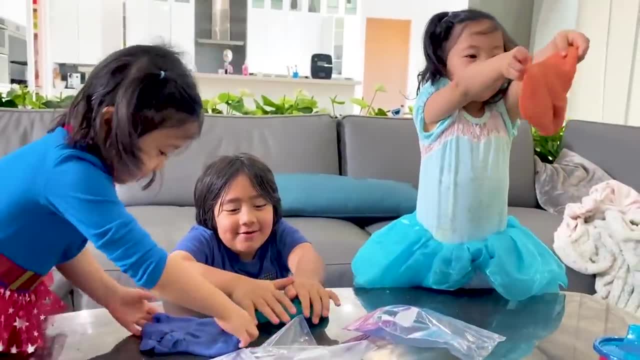 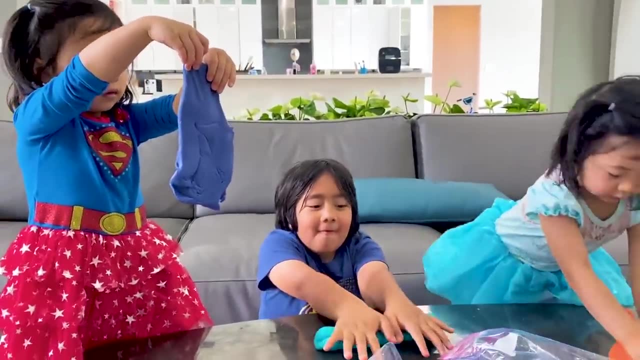 It's cool. Yeah, I like this Play-Doh. Did you bake it? Yeah, I did, We baked it, I bake it, But you guys made it too. You guys helped me. Good job, girls. Wow, Ryan. 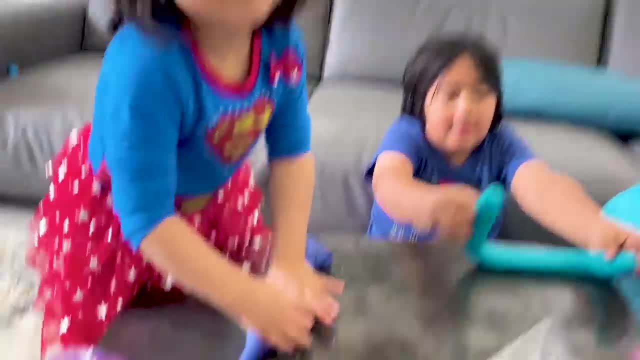 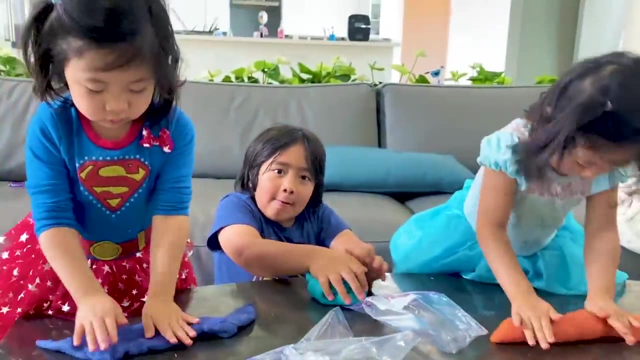 You guys make super long. I'm making Play-Doh. I know I'm gonna do whatever this is. Mom, can you buy me a roller or something? Oh you, Ryan, Next time I buy you a roller, What do you do? 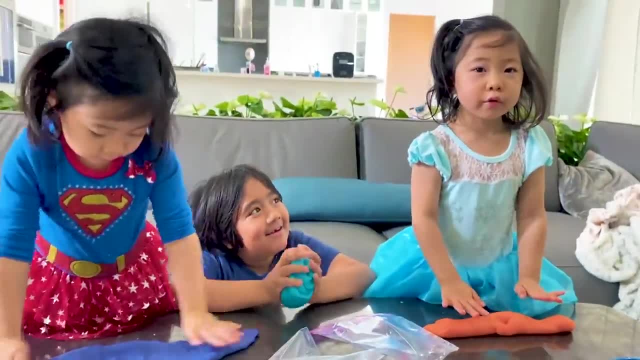 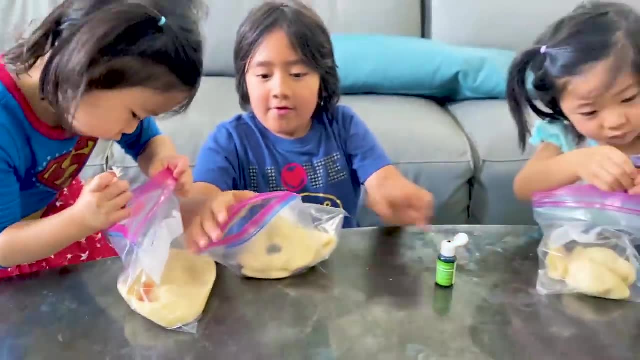 Homemade roller. What if I cut it? You're right, You need to buy roller and cutters for next time. Alright, we're gonna continue making our Play-Doh: Emma's putting in yellow, Ryan's putting in green And then Kate's putting in pink. 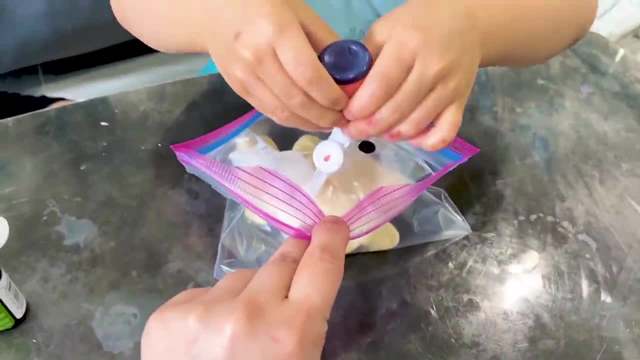 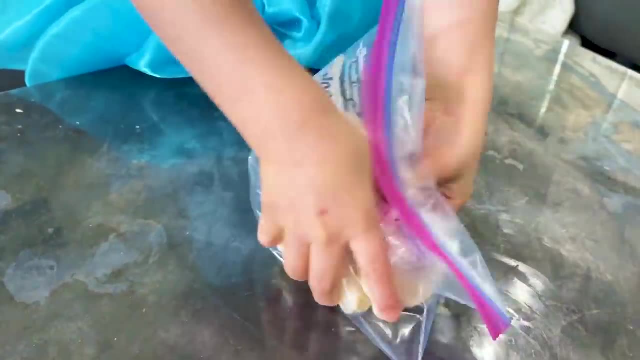 Good job, Kate. There you go. I see some color going in there. Nice, Keep kneeling it. There you go. Oh my gosh, mine went pretty far already. Yeah, There you go. Good job Spreading it all out guys. 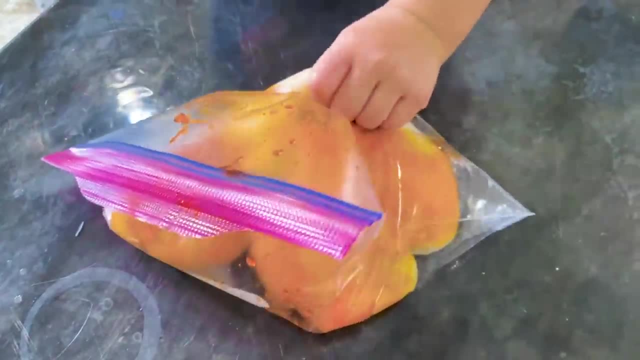 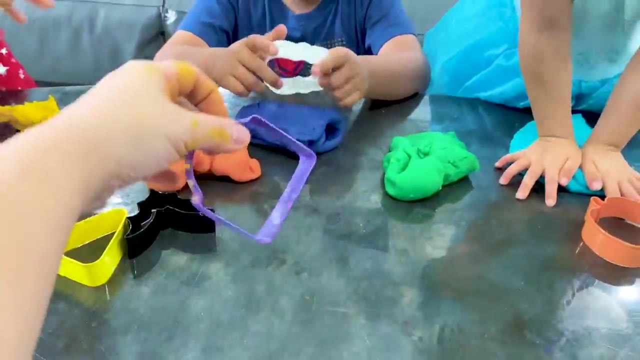 Spreading it all out. Good job, Emma. Emma's looking good too. Alright, I'll show you guys the final result when they're done. So we got all our colors already now. So we have leftover Halloween cookie cutter. We're gonna use that. You guys can use any cookie cutters. 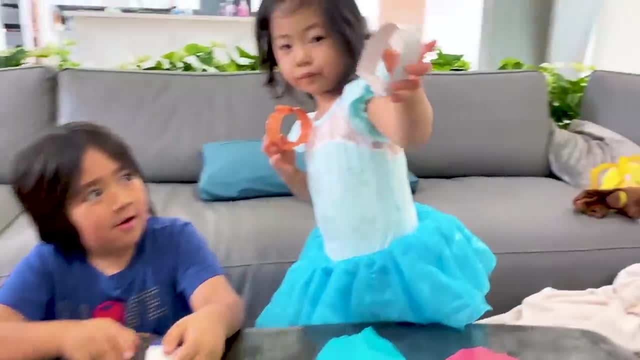 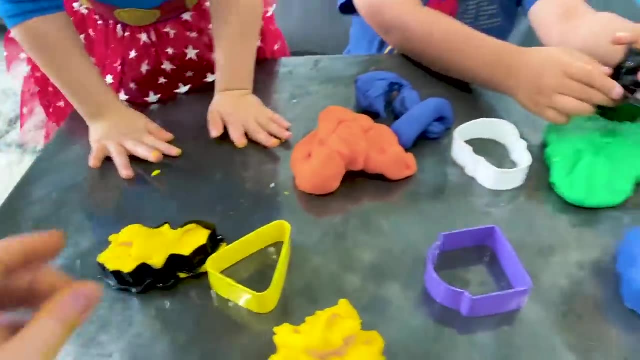 if you have it, Mom, this is a ghost. Oh, that is a ghost. You're right, Oh yeah, And this is a pumpkin. That's right, Pumpkin. I see your bat, Emma. Good job, That's a bat. 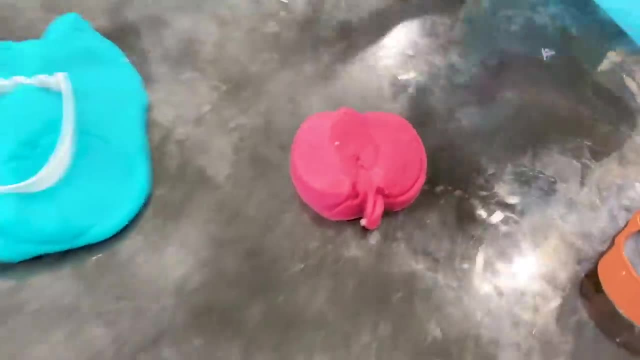 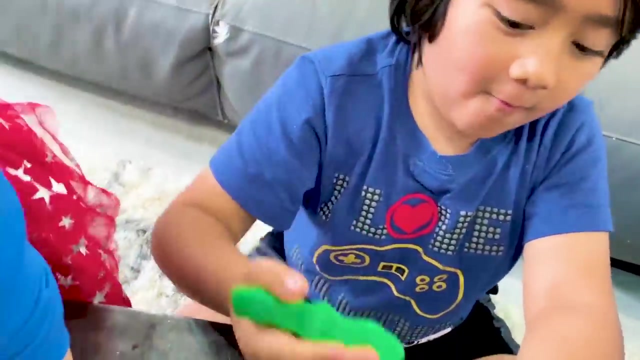 I made a pumpkin You did. Oh, it is a pumpkin, Good job. Alright, let me see your bat, Ryan. Okay, my bat is like this: Oh, it does look like a bat, Good job. All I was missing is some eyes. Good, 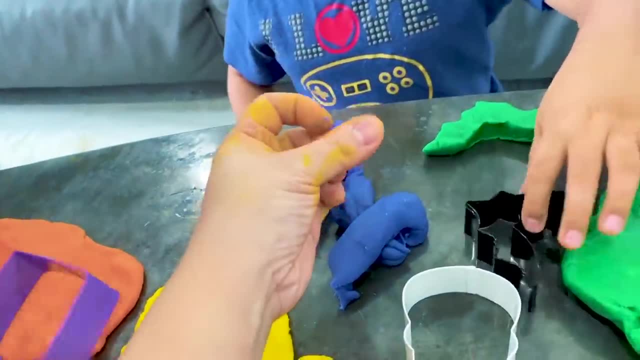 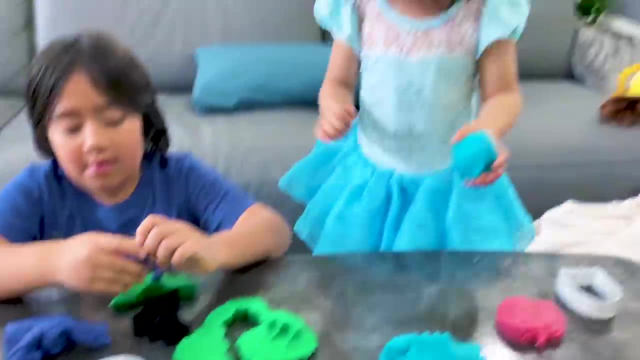 The thing about Play-Doh is you can just get a little thing like this right and then you just make eyes. Oh no, I'm playing. Ryan's bat has a giant one-eye bat. Can I smash it and make a bat? Sure, you can smash it. 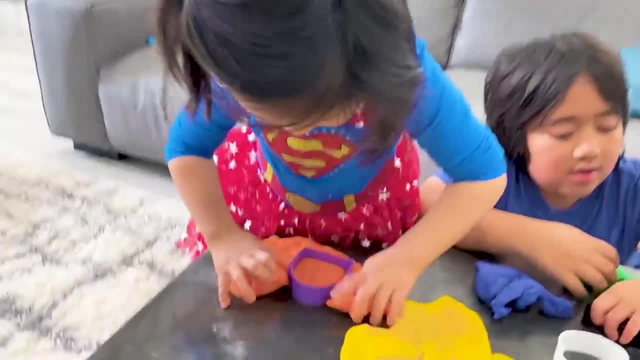 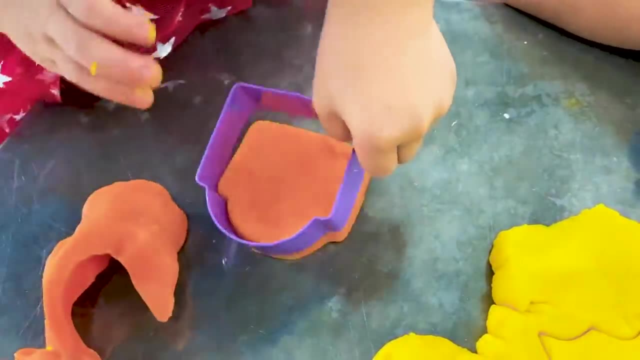 Here. Oh, Kate smashed her bat. What are you making, Emma? I made a house. Oh, it's a house. I made a cookie. Love it. Can I make a cookie Cookie house? yeah, Wow, Oh look, Ryan made a face. 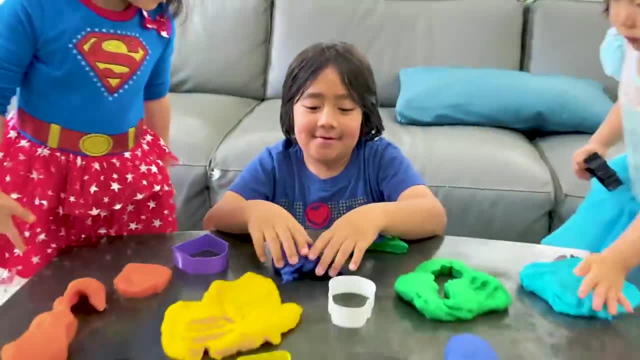 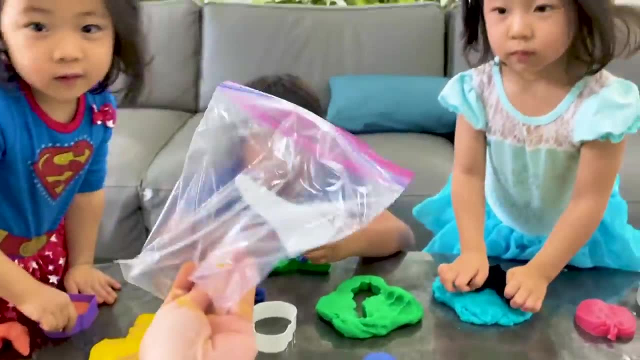 Ha ha ha. Love it. There it is, guys. That's how you make a do-it-yourself Play-Doh, Yeah, And when you're done, you can just put it in a Ziploc bag and save for later, right. 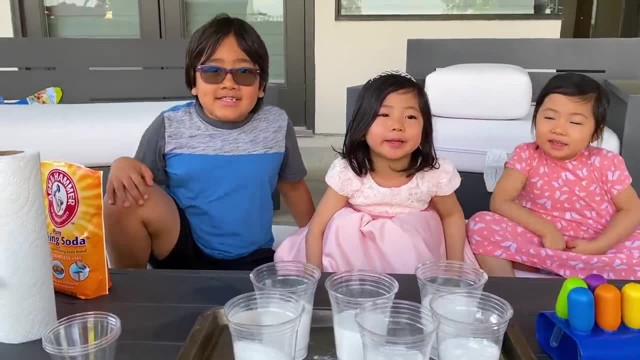 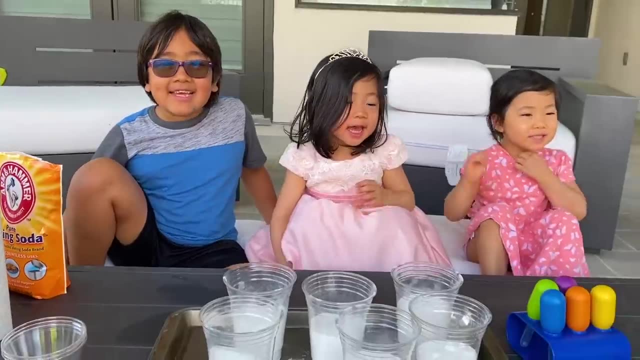 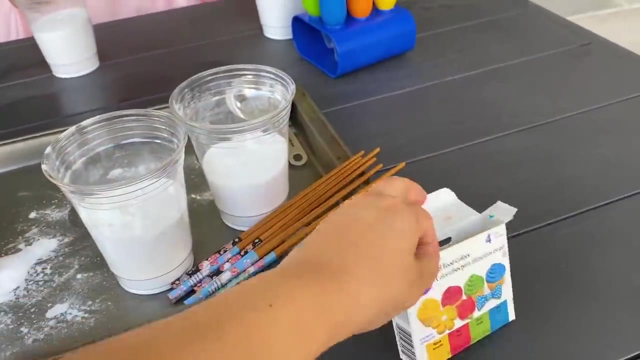 Yeah, We're gonna eat it. Hi guys, Today we're gonna be making a rainbow baking soda and vinegar science experiment. Are you guys ready? Yeah, Okay guys. First step is you just gonna need a cup of baking soda and then your favorite. 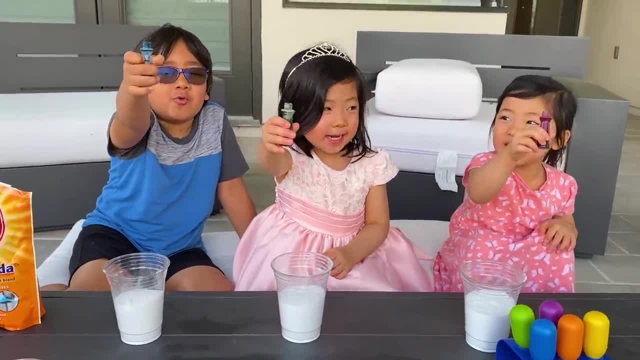 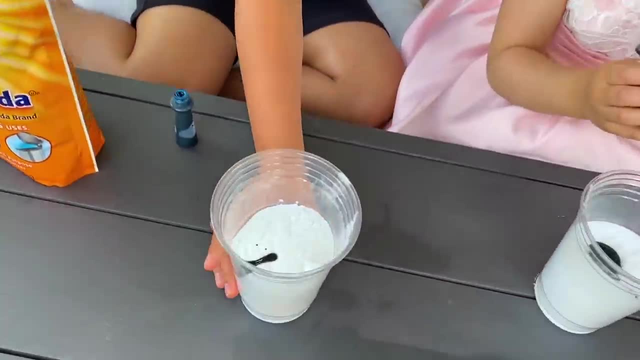 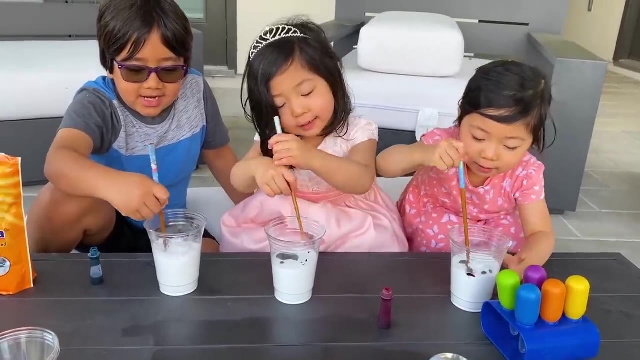 color. So what color are you guys gonna add? Green, Okay, go ahead. Kate did some red, Emma did some green and Ryan did Blue. Next, you're gonna need to agitate to get something. to agitate, Agitate, agitate. 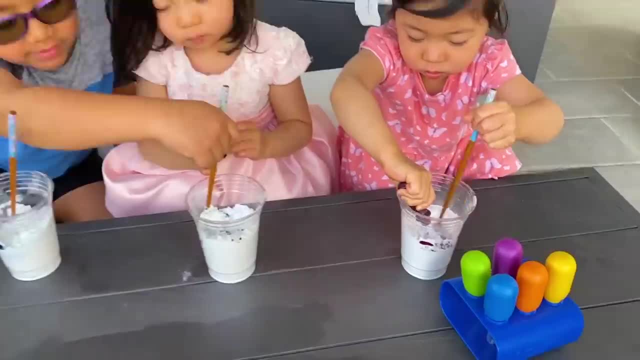 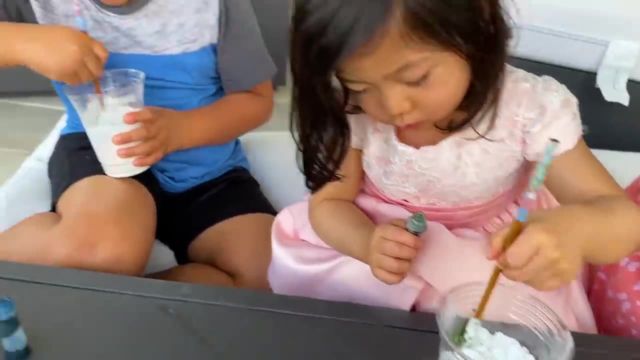 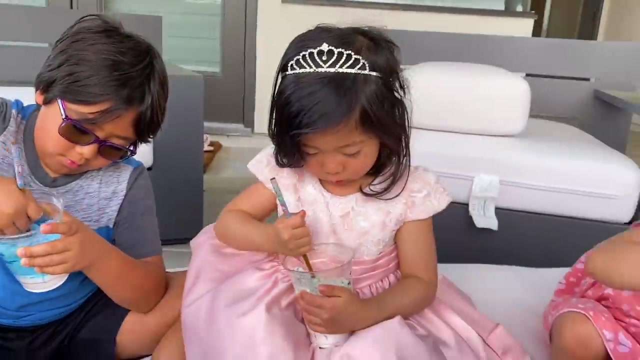 Yeah, Agitate, agitate. There you go, Agitate, agitate Good girls, Good Emma, Good Ryan. Look guys, Mine's almost fully blue. Wow, yeah, Agitating. good, I'm gonna mix in a little more. 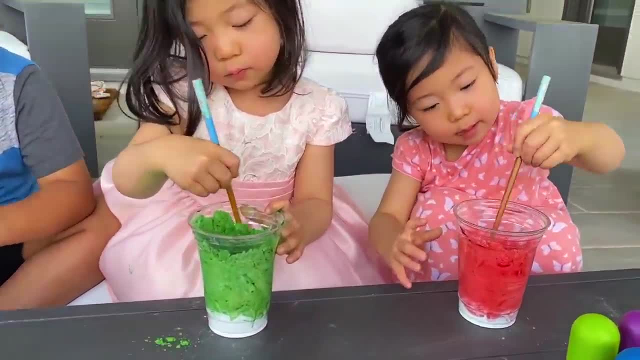 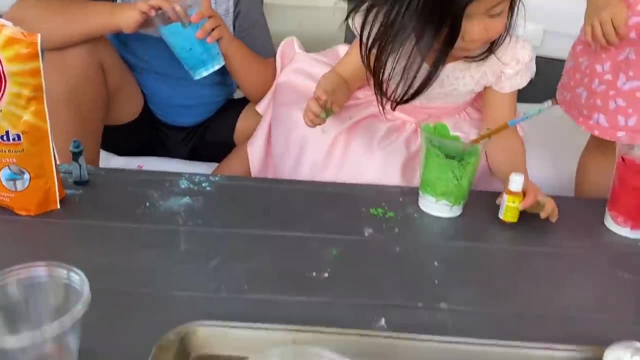 I'm gonna mix in a little more. Yeah, so you guys' colors are going good, See Red, green and blue. Good girls and boys. Okay, so we're done with our three cups. Now we're gonna do these three. 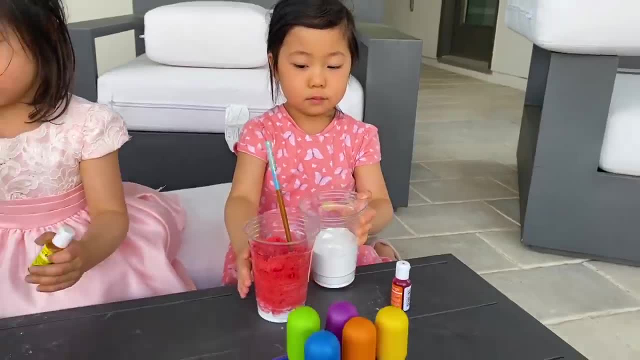 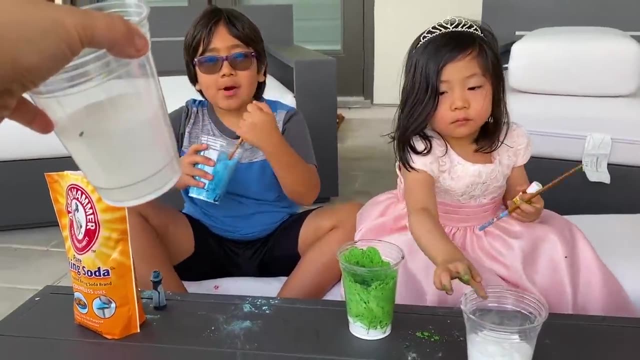 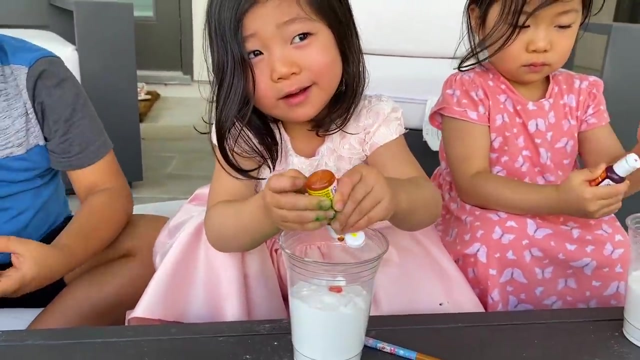 Okay, so Kate's going to do orange, And then Emma's gonna do yellow, And then Ryan's gonna do Purple. Good, There you go, Add your color Purple. It still doesn't look like yellow, It will. Good, There you go, Yellow. 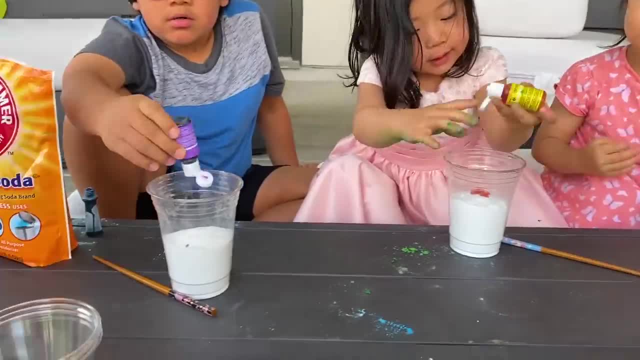 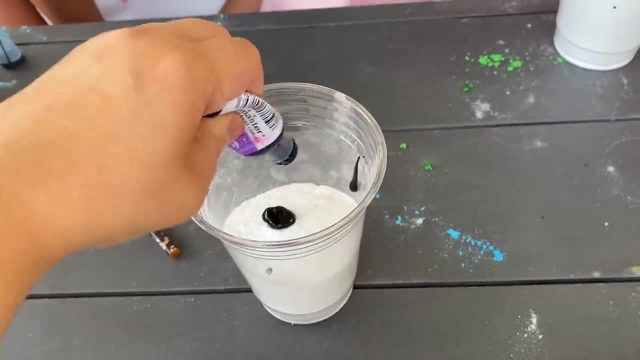 Looks like orange. Kate got her orange. Okay, I think that's enough. Okay, there it is Purple's out, but it's okay. Whew, look at the bubble. Look at that giant purple bubble. Alright, start agitating. 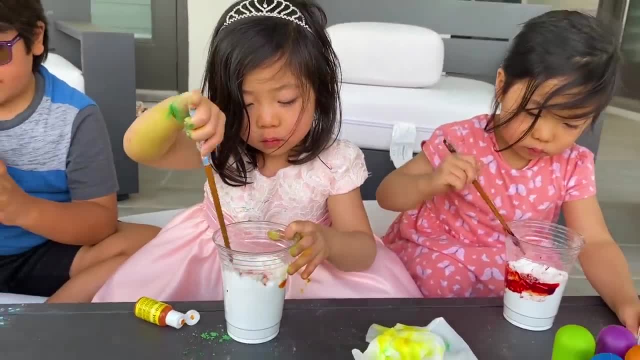 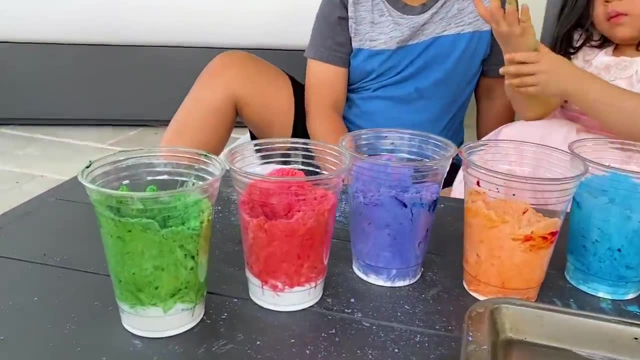 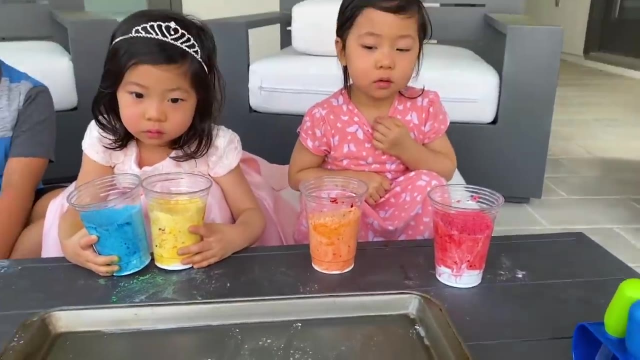 There you go: Agitate, agitate, Agitate, agitate, agitate, agitate, agitate. Okay, we got our rainbow colors. Nice, Okay, guys. so now we're gonna pour all the colors into this pan here. So, Kate, you can. 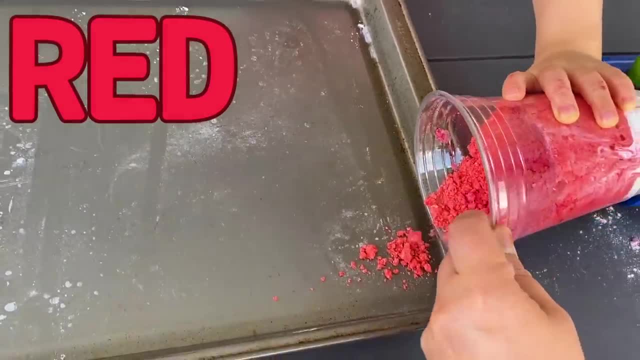 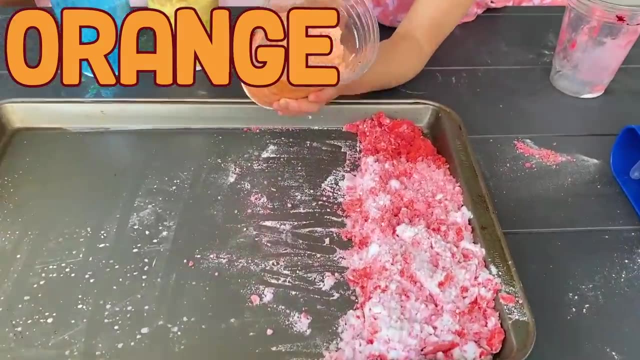 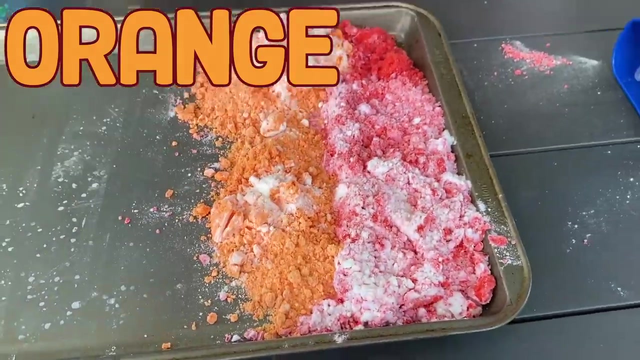 start first with red, Pour it in. Yeah, There we go. Okay, we got our red and now we're gonna do our orange. Alright, there we go. Orange. Ooh, Nice. Good job, Kate, Let's go. 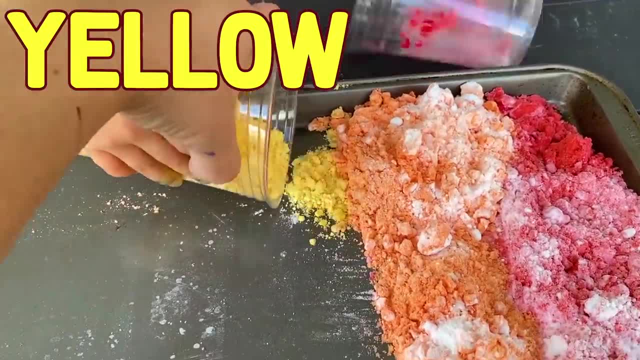 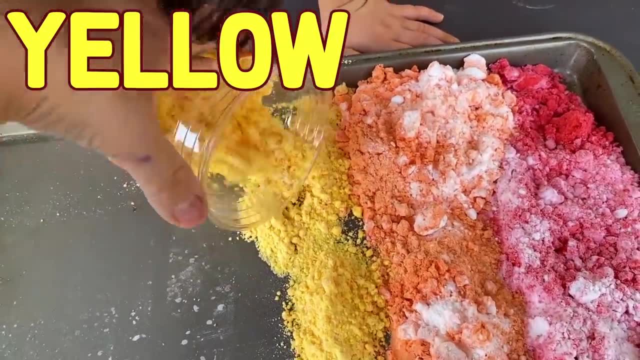 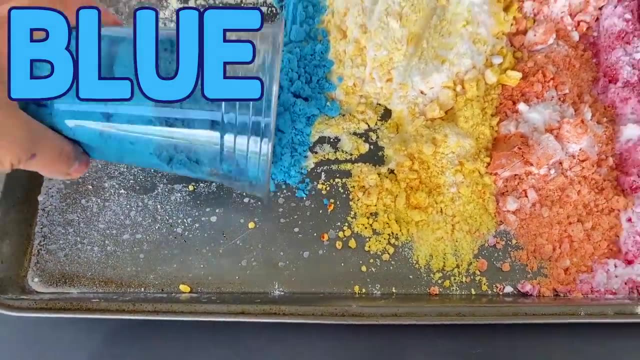 There you go. Good, I help you. It's okay. There you go Good girls. Wow, So beautiful. huh, Yeah, it's like a rainbow. Yeah, Now we do blue Good. There you go, Yeah. 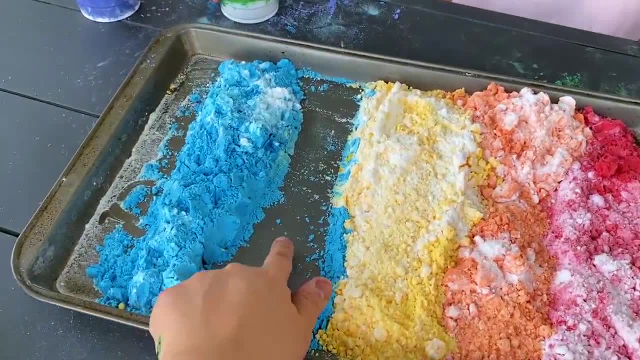 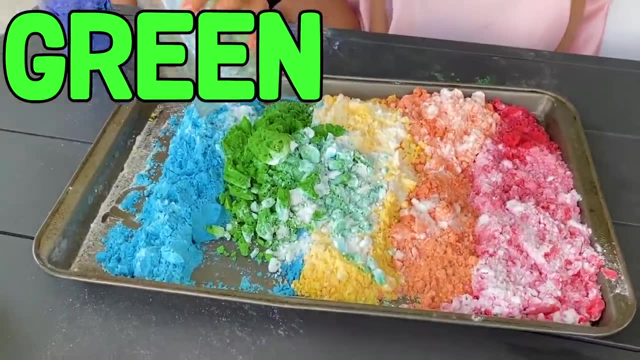 Beautiful. Okay, so we accidentally forgot the green here, so Ryan's gonna pour the green. Yeah, There we go. Whoa, It's okay, We can fix it. Spread out the green. It looks pretty. huh, Yeah, There's actually a lot of green. 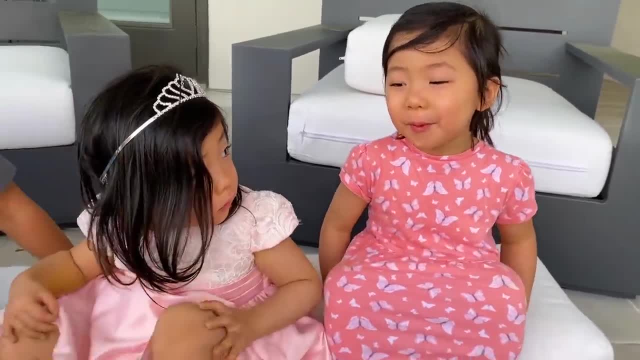 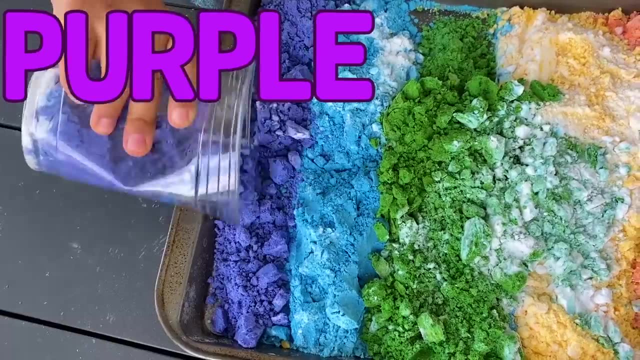 Yeah, It was like a rainbow, but now we need purple. That's right, purple, Yeah. Wow, so beautiful. It looks like a rainbow, It does. Now Mom can use these. Yeah, almost done. Good job, guys, You're gonna need some. 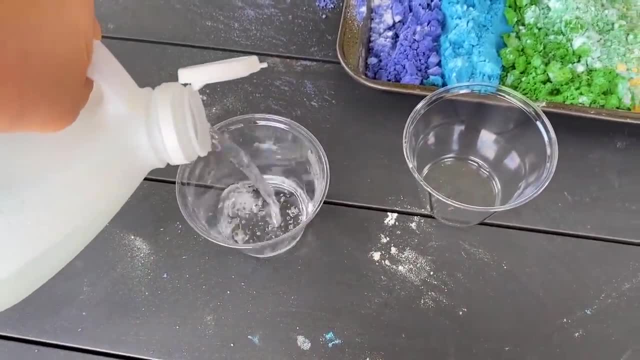 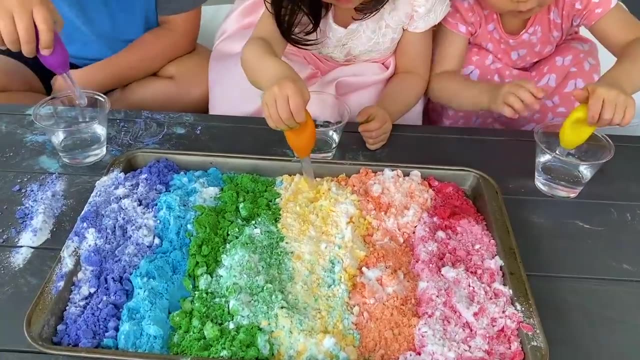 vinegar here? Yeah, of course. Okay, I'm gonna pour some vinegar in each cup for you guys. Okay, there you go, Pick up some vinegar and then just do it. Yeah, Emma, squeeze Like this. You see the bubbles. 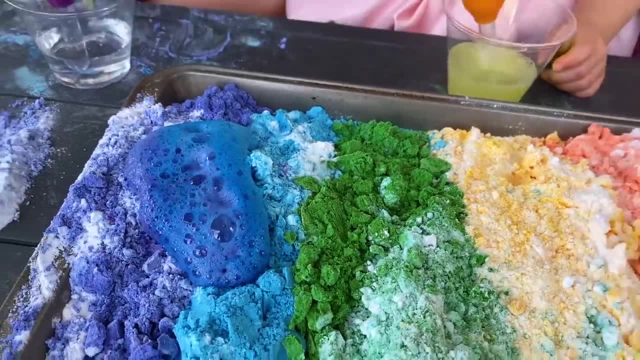 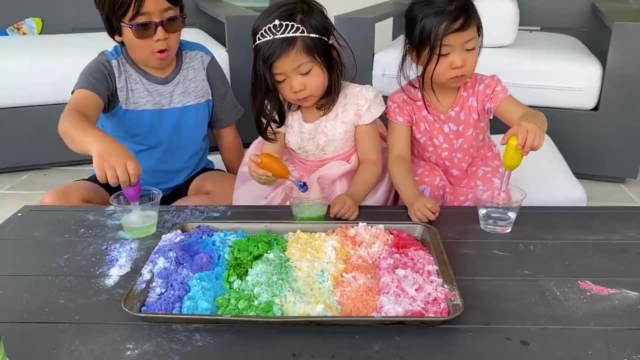 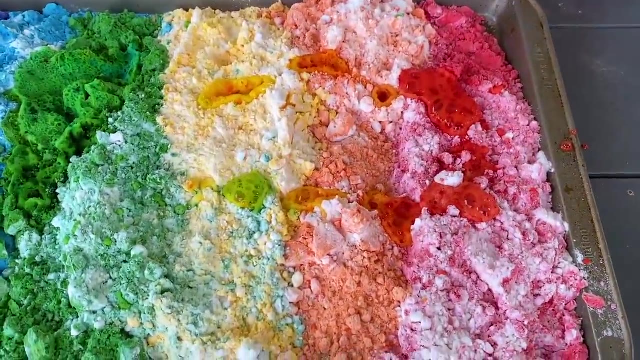 Emma, look, Whoa, Look, I put some bubbles. The way you're mixing the colors: Whoa, Whoa, Whoa, Whoa, Wow, And it's so many colors at the same time. Yeah, And it's growing. 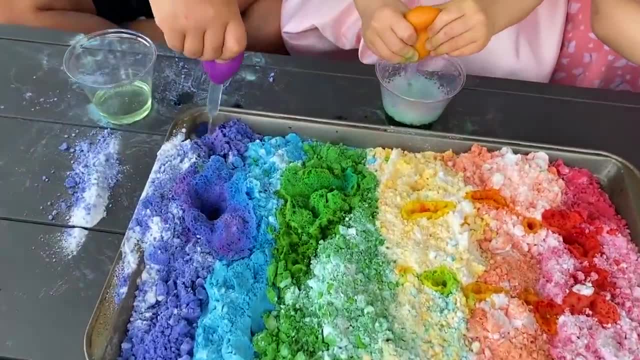 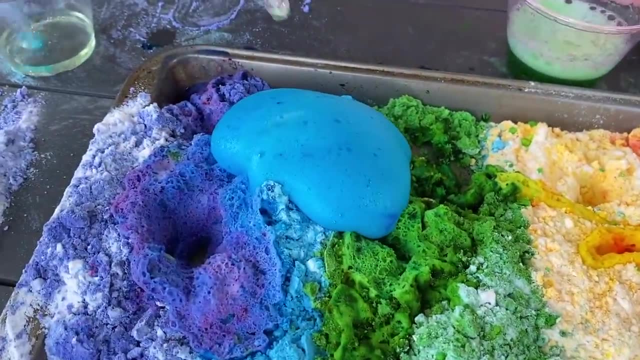 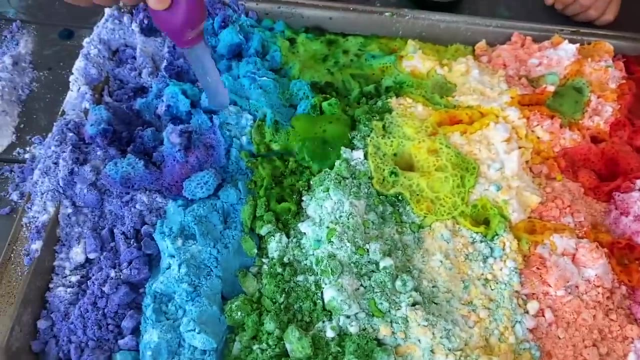 And that's just mixing up. I'm gonna do the same with all of the colors. Okay, Whoa, Whoa, Whoa, that's a big one. I have a reaction inside my cup. Whoa, Whoa, That's cool. 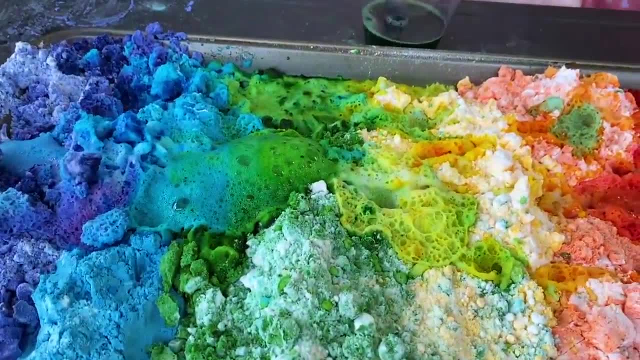 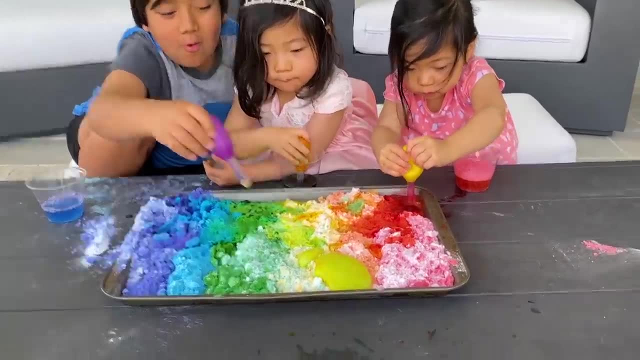 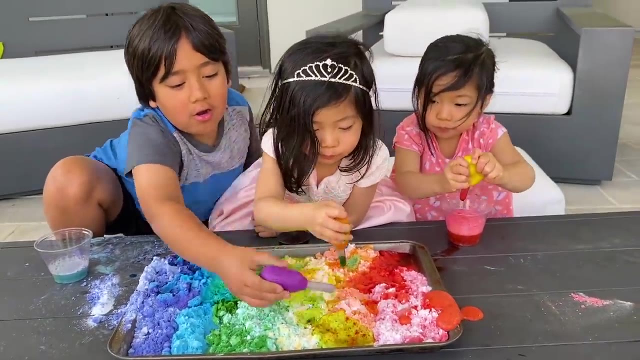 Whoa, Whoa, There's a spot you guys haven't done yet. Okay, I'm gonna do it on one single spot. Okay, Whoa, that's giant. Another one, One was wet. Whoa, This is so wet. 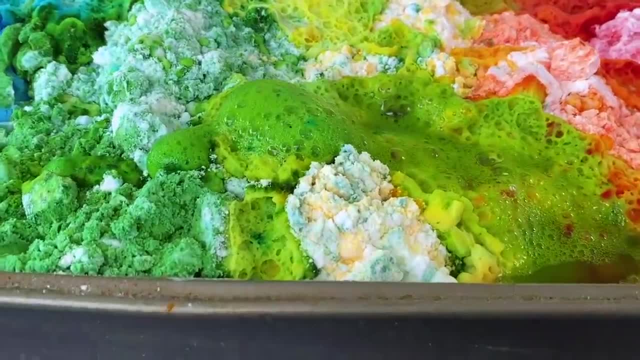 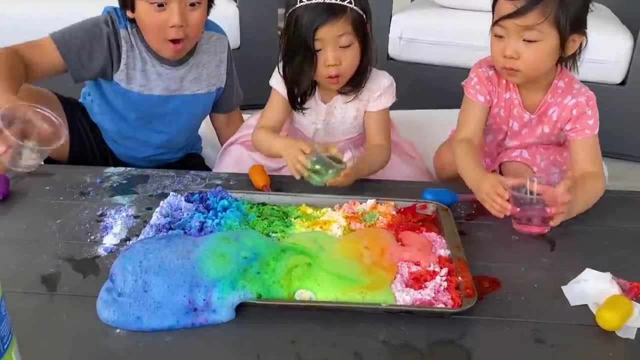 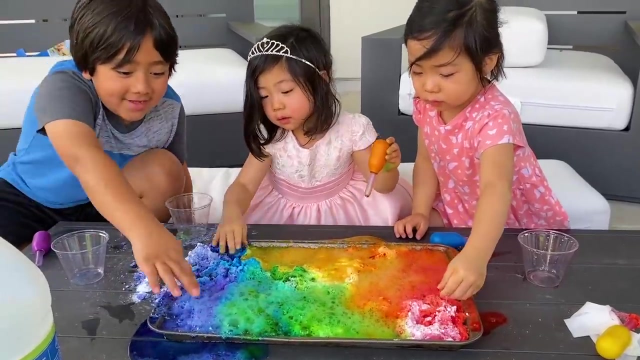 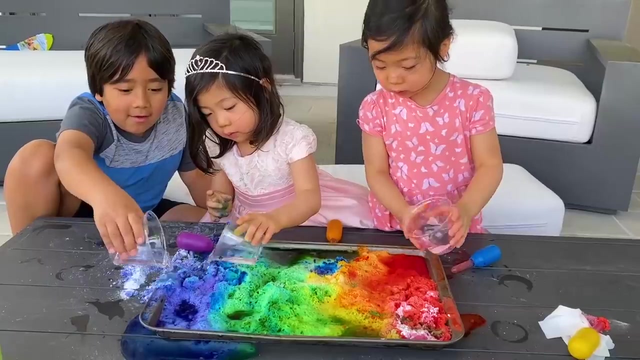 Yeah, Whoa, look at the bubbles. Okay, Okay, we're gonna pour it now. Whoa, Whoa, Whoa. Can I touch it? Yeah, Look at this, Whoa, It looks so cool. That was fun, huh. 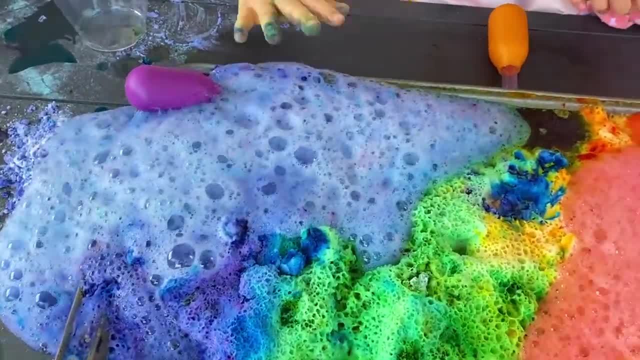 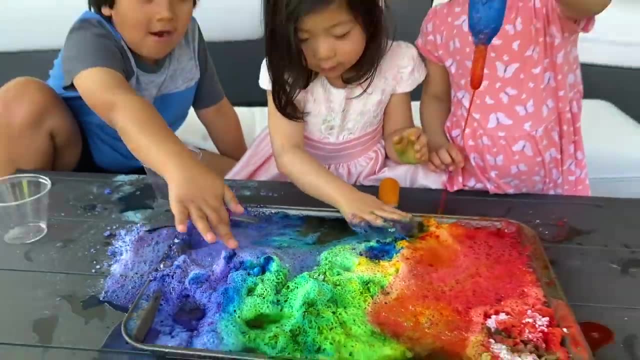 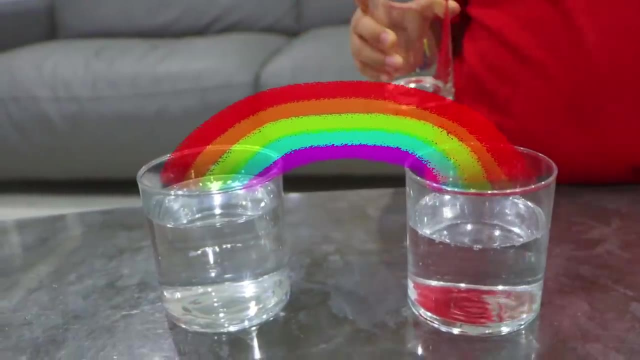 Yeah, Whoa, Can I touch it? Yeah, Whoa, That's super cool. Yeah, Hey guys, today we're gonna grow our own rainbow. All you need is a paper towel, scissors, markers and cups with water. 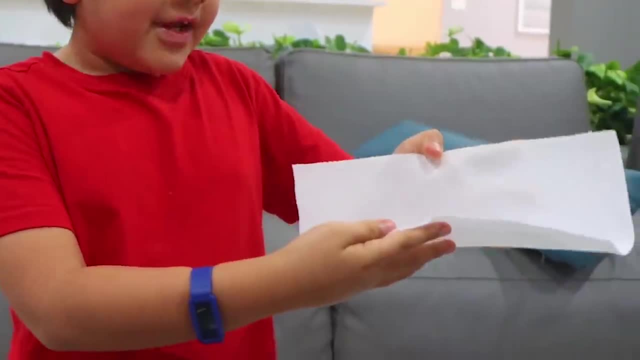 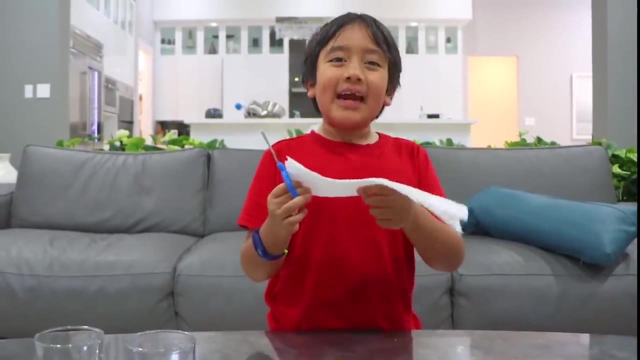 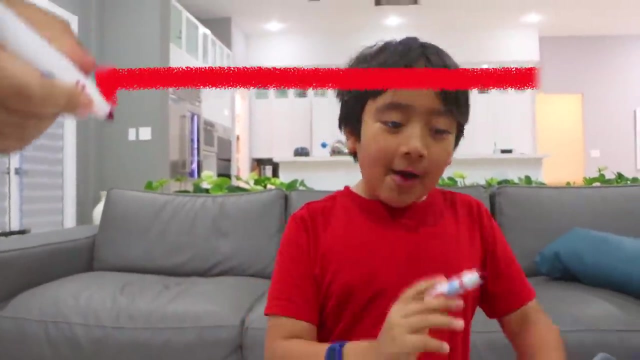 First, using your paper towel, you're gonna fold it in half And then we're gonna cut it. one fourth, Don't forget to ask a grown up for help, And I have mommy here, Hi, Thank you Now with any marker you want. 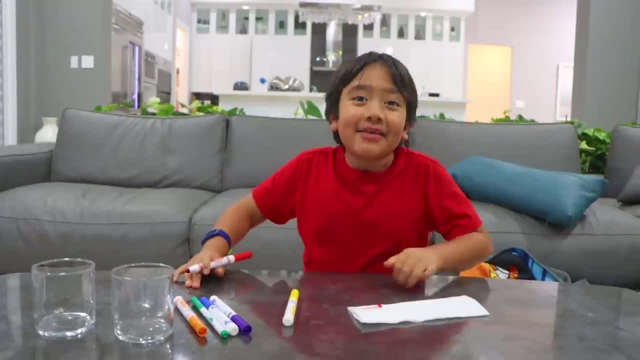 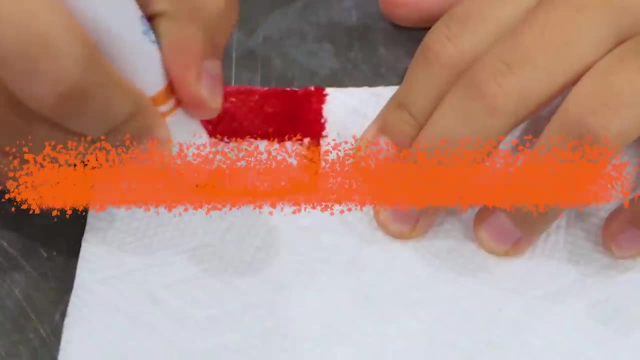 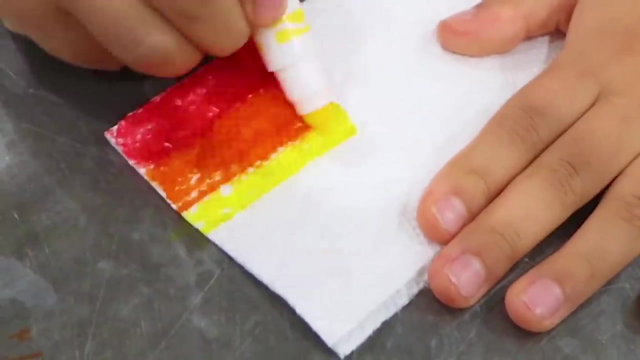 make a rectangle like this: Now, let's color it in. The next color in the rainbow is orange. Put it like this: Now let's fill it in. Next is yellow. Okay, let's fill this in. Next is green. 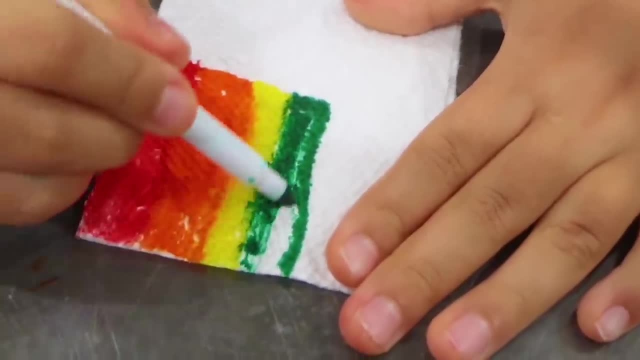 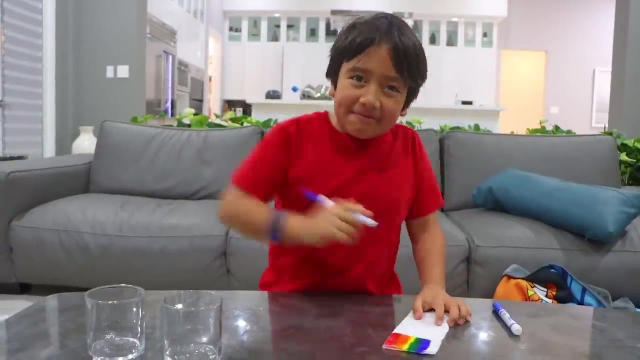 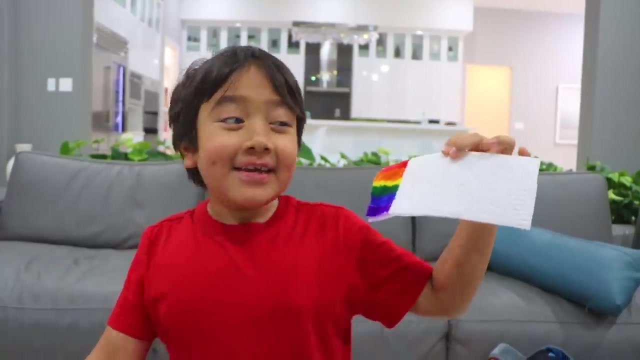 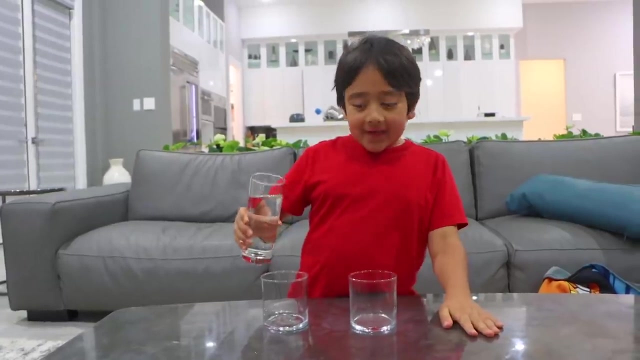 Fill it in Green. Next up is blue. We're gonna finish it off with my favorite color, purple. Now do the same thing to the other side. Like this, See, Like so. Next, fill up your two thingies of water. 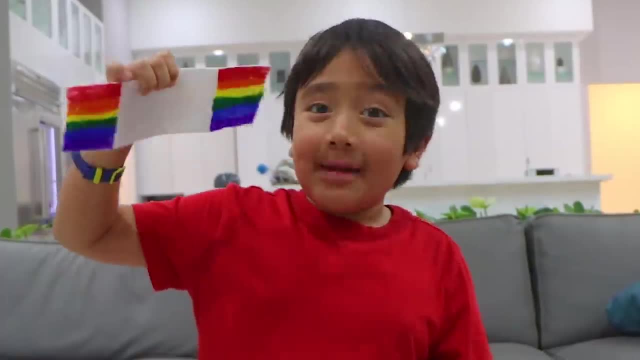 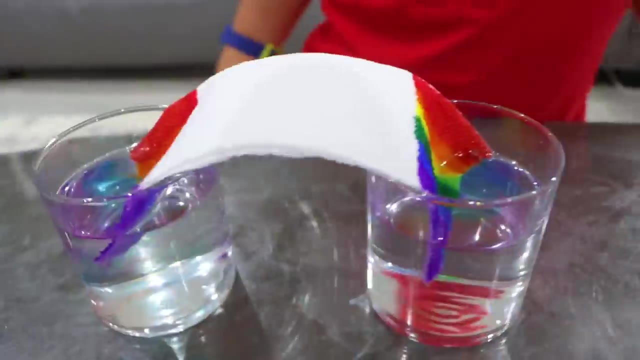 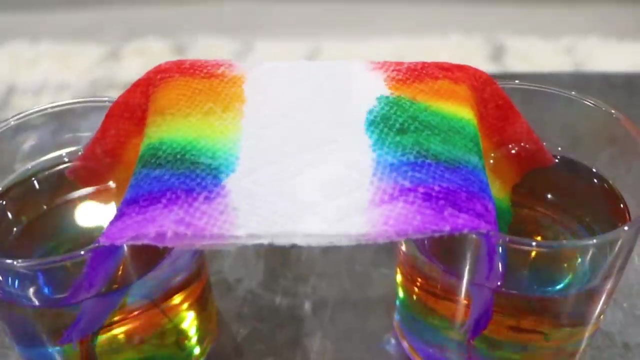 And the second one. Now take your rainbow paper that you drew and put half of both of the sides in the water. Now we wait. Watch the rainbow form. Look, it's already forming a little bit. Whoa, guys, did you see? 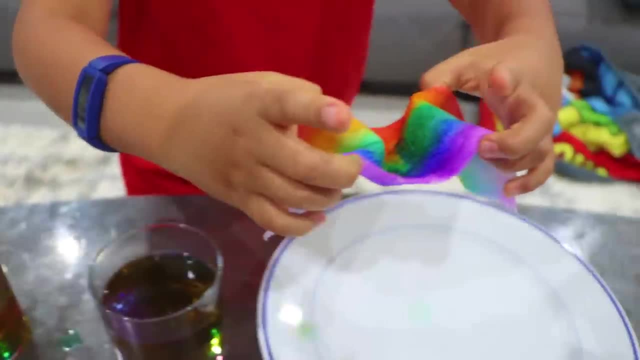 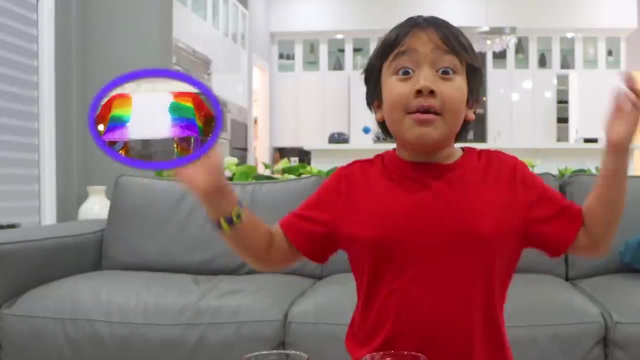 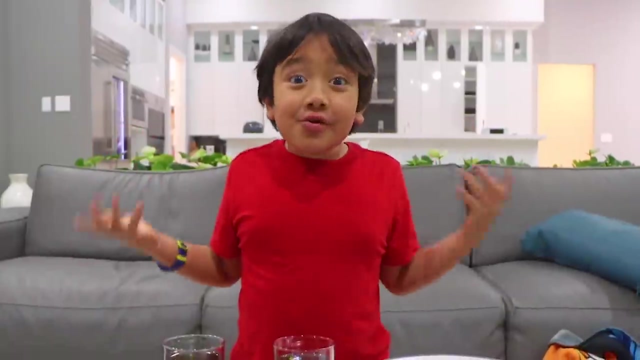 We made our own rainbow. Whoa Put it right here. This is so cool. Did you see the marker die? move up the paper towel and touch each other, Cause that's called capillary action. Did you know regular plants also use capillary? 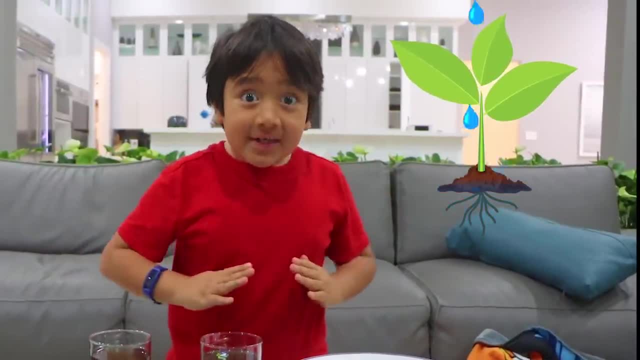 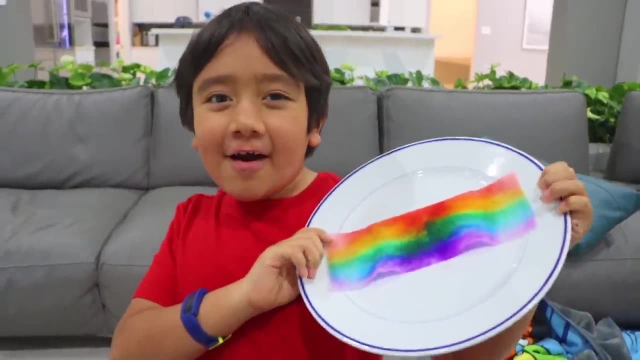 action cause they bring the water from the roots and make it go all to the other parts of the plant. I hope you guys had fun making our own rainbow together. Hey guys, today we're gonna paint our names. We have E for Emma. 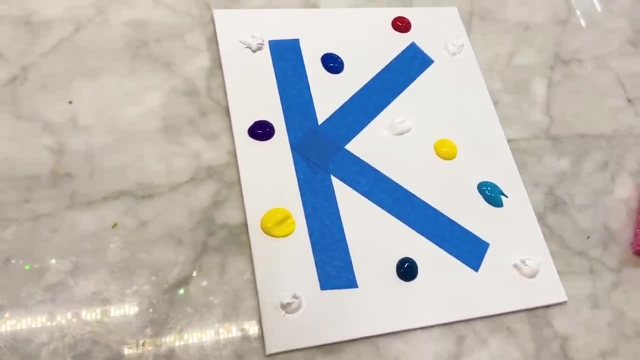 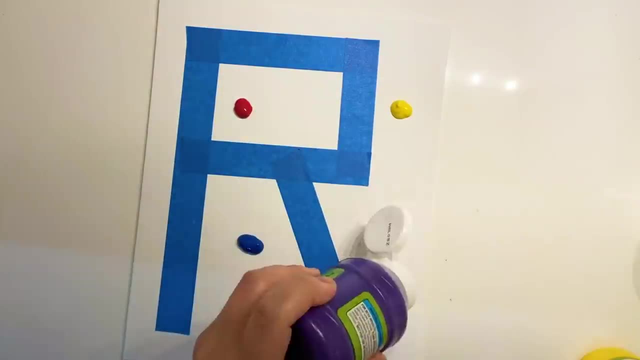 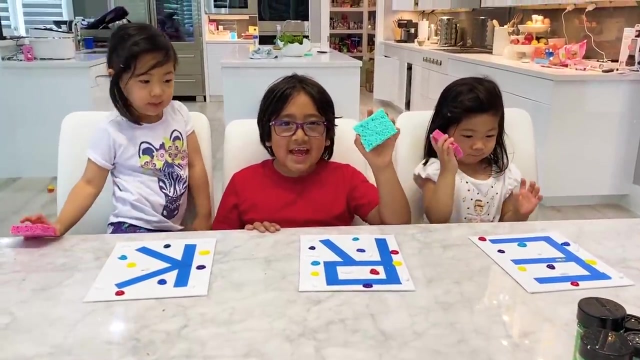 R for Ryan and K for Kate. And here's how I did it All. right, you guys ready? Yeah, So first we're gonna take our sponge and then dab. Is this dabbing? Yeah, This dab. Yeah, any way you like. 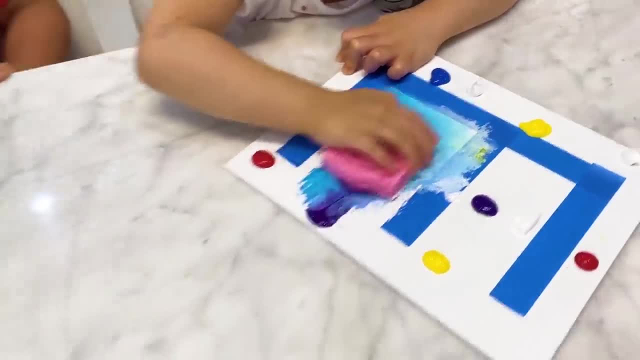 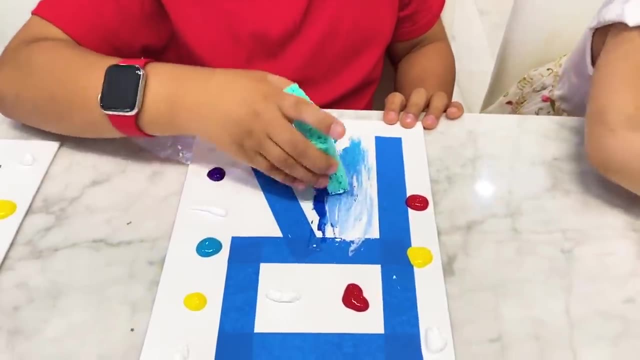 Whoa, that's pretty, Emma, Thank you, Okay. and then, Ryan, Mommy, when I dab with this, then we open the table. That's right, Okay, Ryan, It turned into a dark yellow. Oh, nice, Good job, Kate. 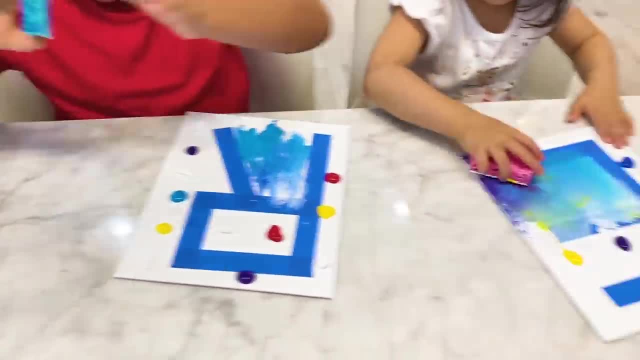 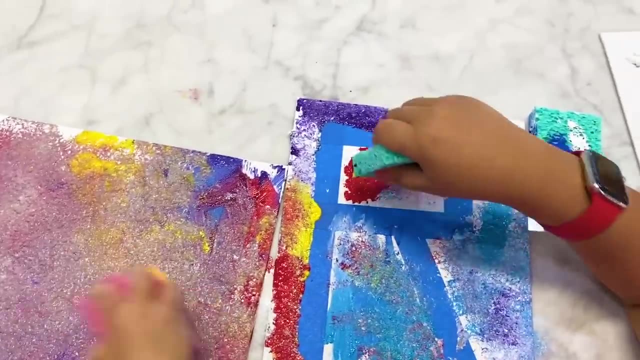 Okay, So we're gonna just mix the color together. Good job, Kate. Oh, that's pretty, Ryan, I think I'm almost done. Beautiful Emma. Thank you, Mommy, I'm done. Okay, Emma's done. I'm waiting for Ryan. 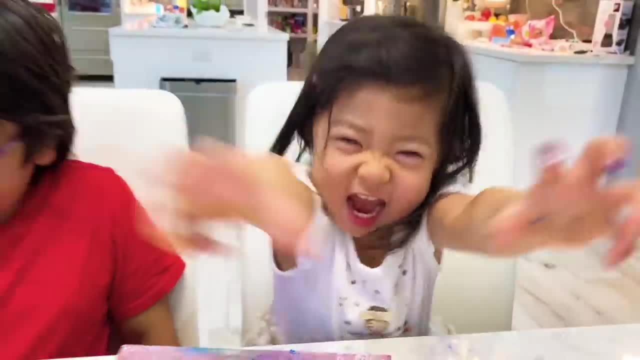 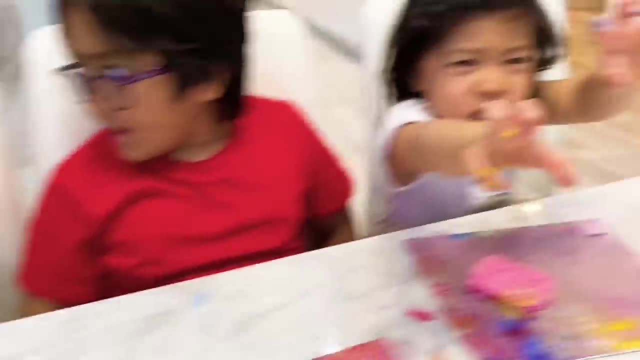 Ugh, I think I'm done too. You're done. You gotta cover every single space, like Emma, And now it's just Kate left. Wow, I'm turning green. Yeah, you're doing great, Kate. There you go. Good job, Kate. 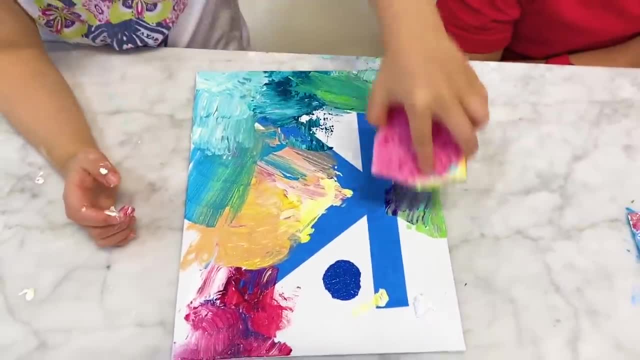 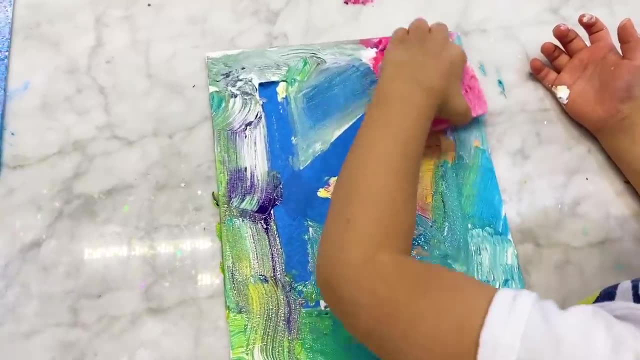 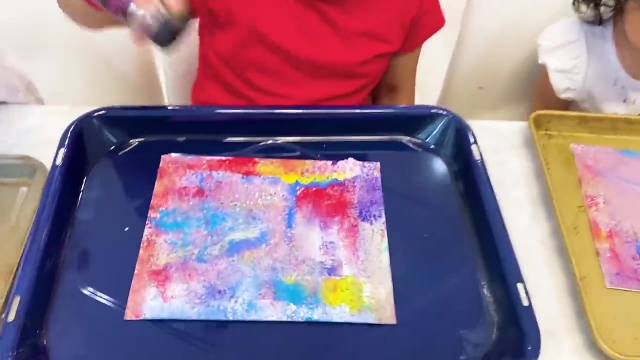 That's good. Whoa, That's pretty. huh, Yeah, Wow, Beautiful artwork, you guys. Thank you, Done Kate. Good job. Now for the fun part: Glitter, Alright. so everybody pick your favorite glitter and just sprinkle it in. 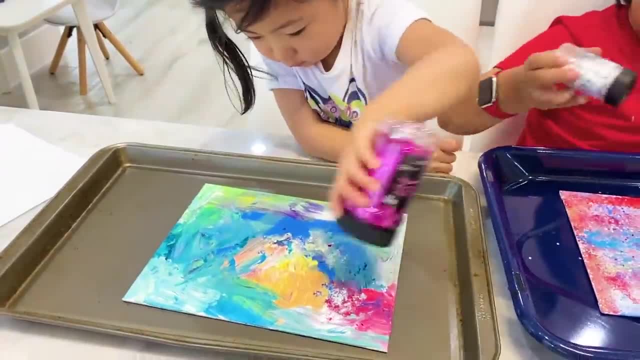 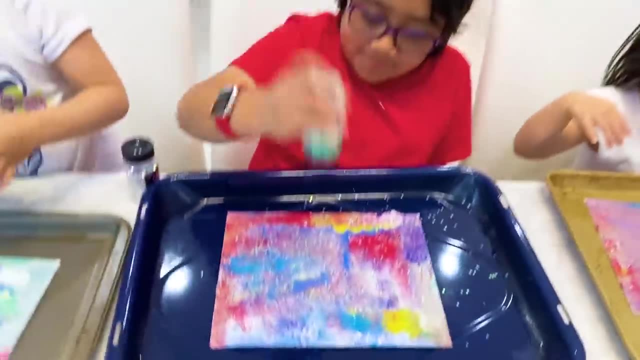 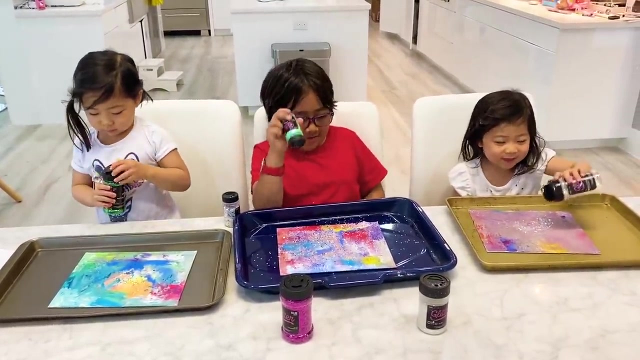 There you go. Good job, Kate. How about that one? This one, Yeah, This one's pretty. Wow, Pretty Okay, Ryan, over here, Like a salt, Like salt, We're gonna eat the sprinkles, That's right, No eating. 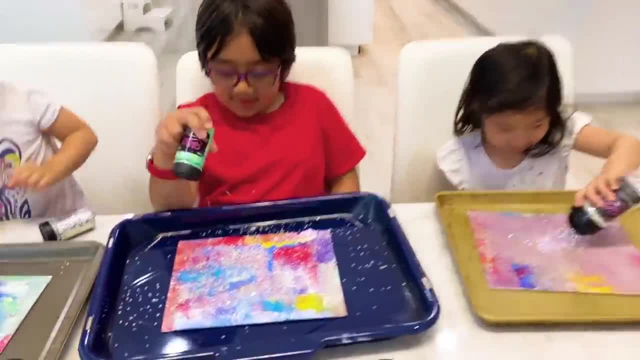 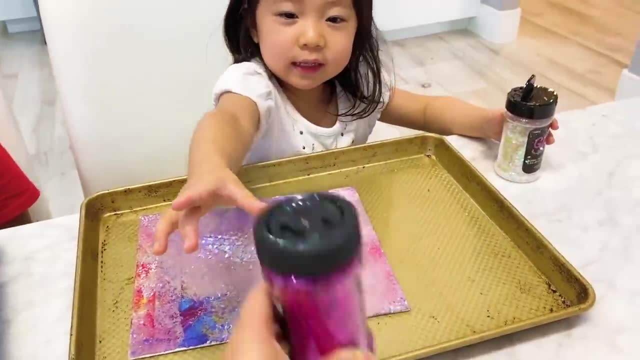 sprinkles. I don't think it'll go in my tummy. It's so tiny. It's pretty. Can I have some, Kate? Of course, Yeah, I need some pink to make it prettier. Okay, Emma, you don't have to forget to spread it around too. 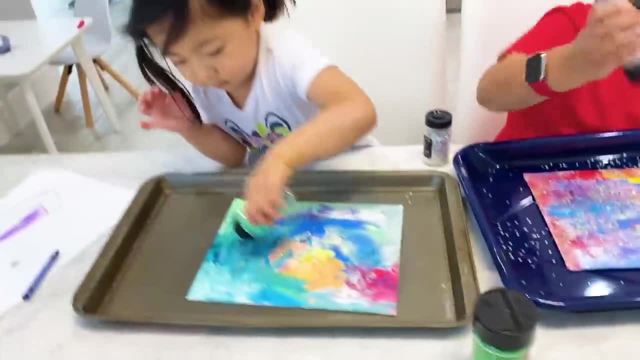 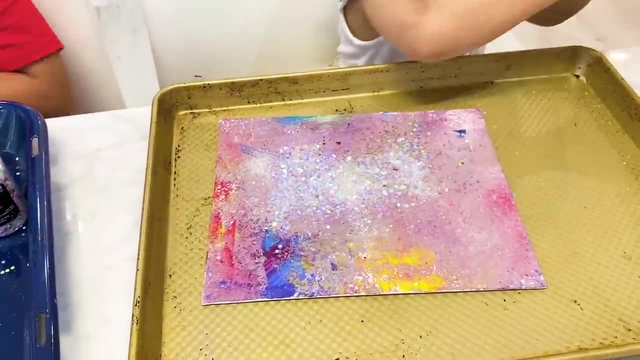 Not just one spot, Everywhere, There you go. Good job, Kate, Like that, Yeah, Everywhere. Oh, this actually kinda looks like salt, Huh, Oh, yeah, It does. Okay, I think this is perfect, Beautiful Kate, Emma's double doing it. 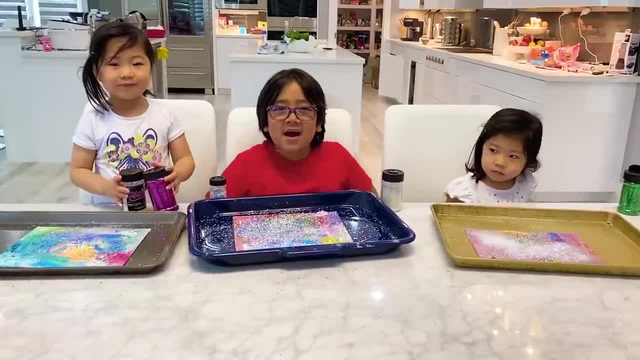 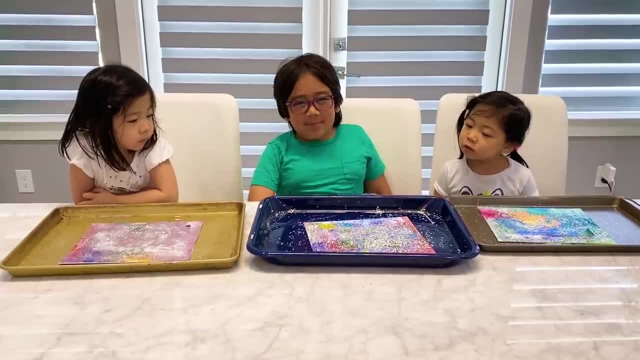 Wow, Beautiful Kate. Okay, guys, Now we're done. Now we're gonna wait for our art to dry. Here goes the money. Okay, guys, It's not super dry yet, but we're ready to peel off the tape, Whoa. 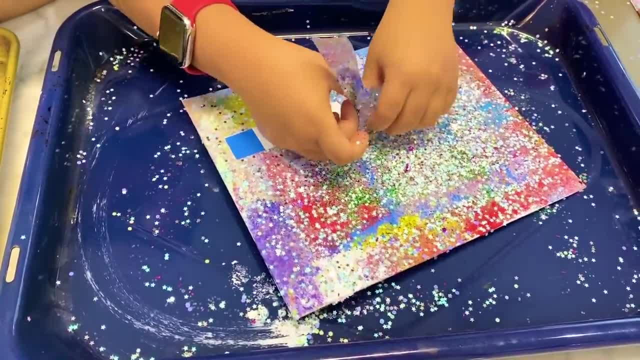 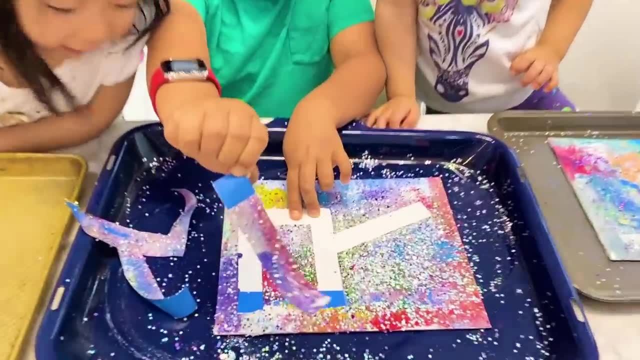 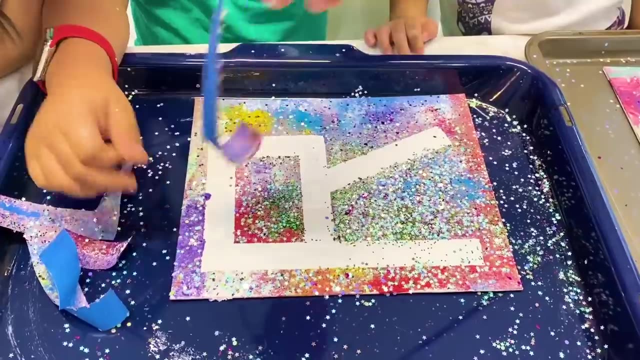 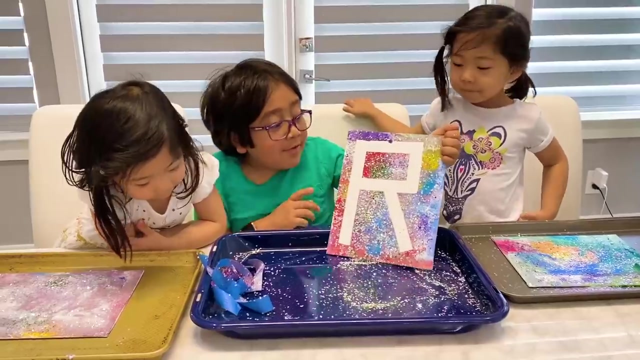 Oh, Look, look, look, Yeah, That looks cool, That looks cool. Yeah, Okay, One more, One more guys. Oh, Oh, good job. Whoa, That's beautiful Ryan. What do you think about my art guys? 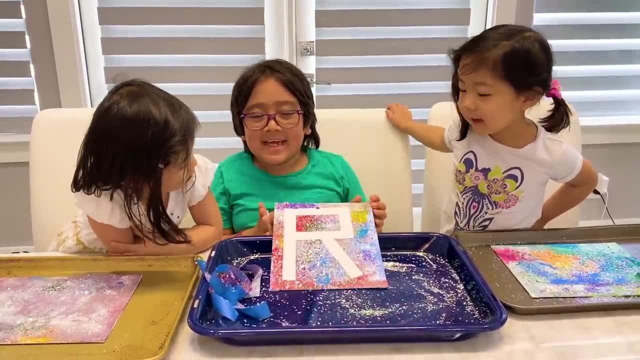 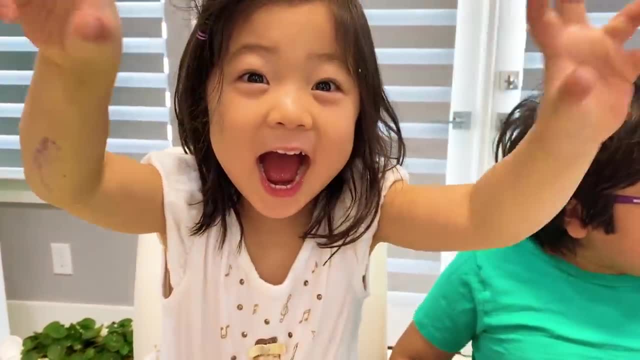 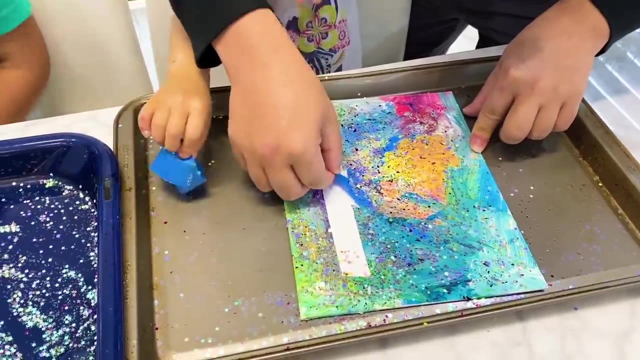 Is it good? Now it's Emma's and Kate's turn. Okay, come on, Daddy. Okay, Why don't you peel this one? You got it, Kate, Whoa, Mm-hmm. Nice, You can peel this one off too. 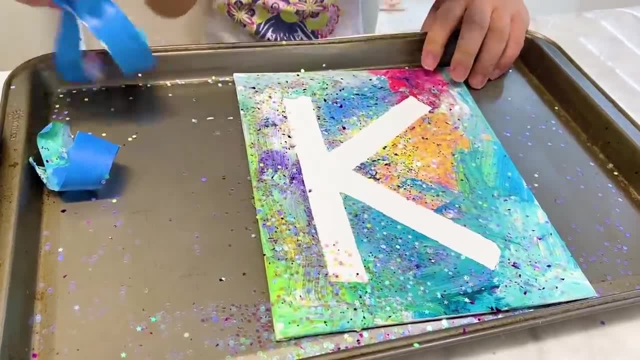 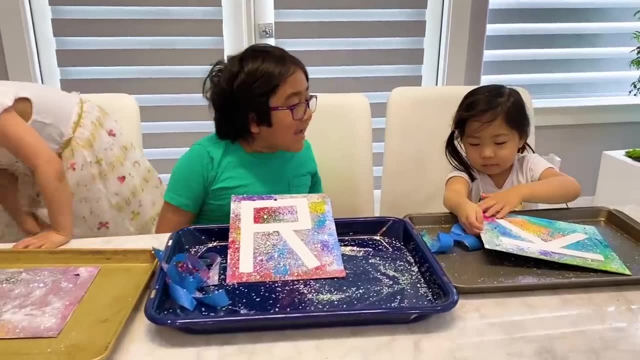 Whoa, Whoa, Whoa Kate. Yeah, Wow, Good job, Kate, That's beautiful. Whoa, Kate, Good job, Let's shake it, shake it, shake it, Let's get the glitter off. Yeah. 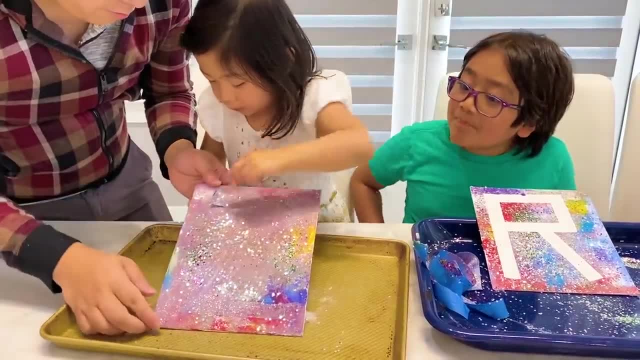 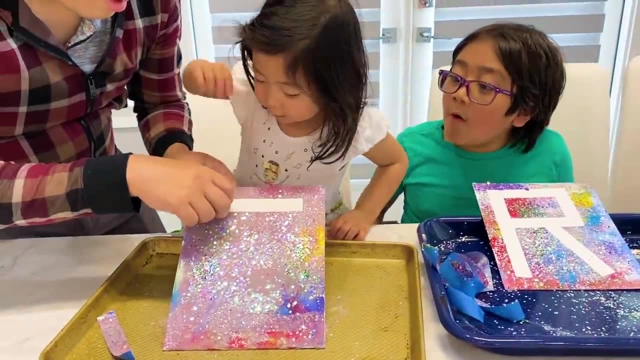 Let's shake it, shake it, shake it, Boom, boom, boom, boom. Why don't you peel this off? Okay, Whoa, Daddy, can I help you? Yeah, Yeah, Emma's peeling, Whoa, Whoa. 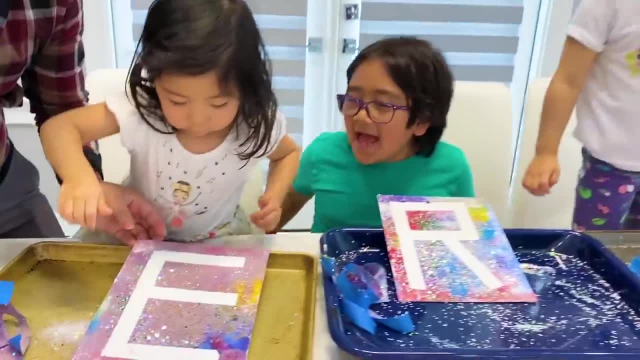 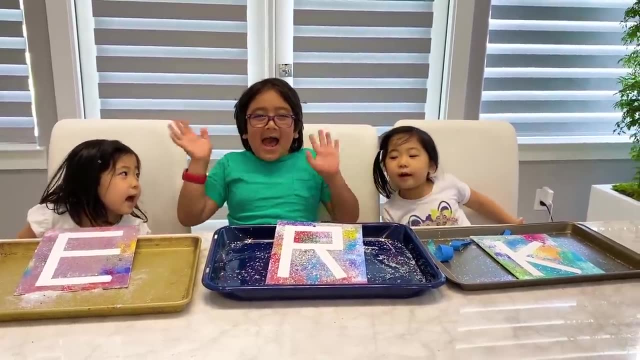 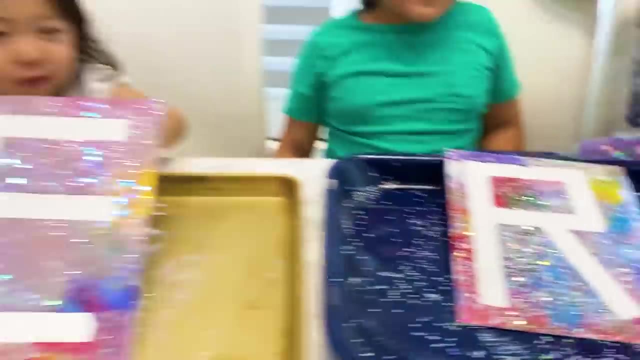 Whoa Good job. Yeah, Good job, Kate. You guys like it. I hope you guys like our picture. Bye, Remember, always stay happy and rise up. Bye. Do you like this picture of me? Yeah, Do you like Ryan? 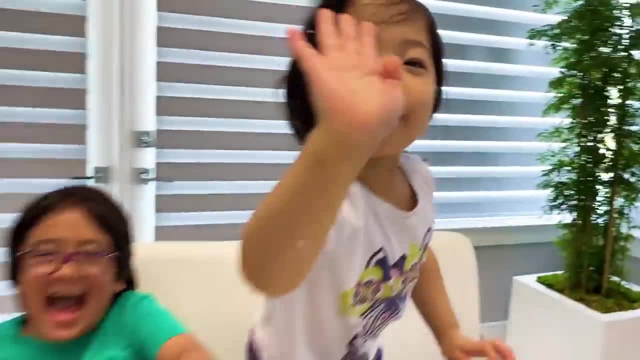 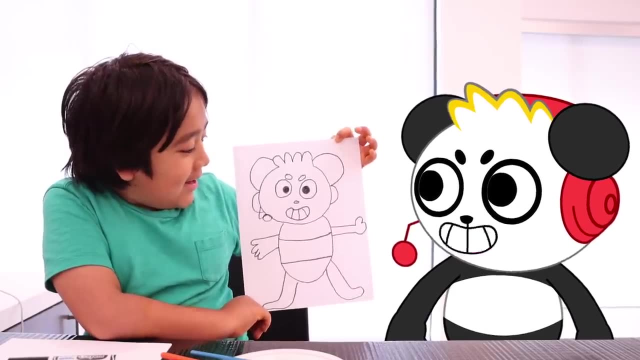 No cry babies, No cry babies. Okay, guys, This is my combo panda drawing. What do you guys think? Wow, It looks exactly like me. Ryan, you did a great job. Now let's learn how to paint me, Oh, okay. 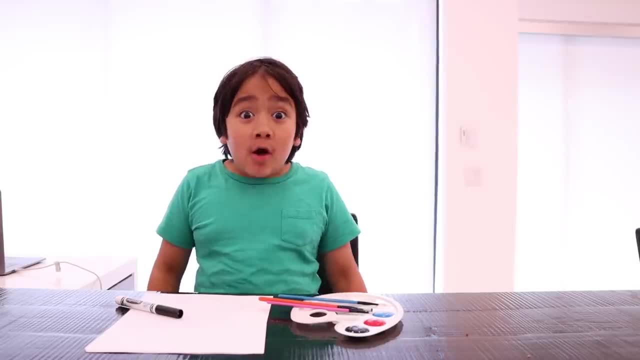 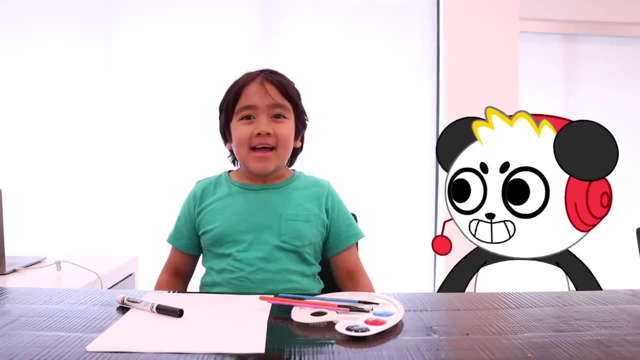 Hey guys, Today we're going to learn how to draw and paint Combo, Panda and Gil together. That's right, Ryan, I'm getting some help from a special friend to learn how to draw me. Are you ready? Let's get started. Combo Bunga. 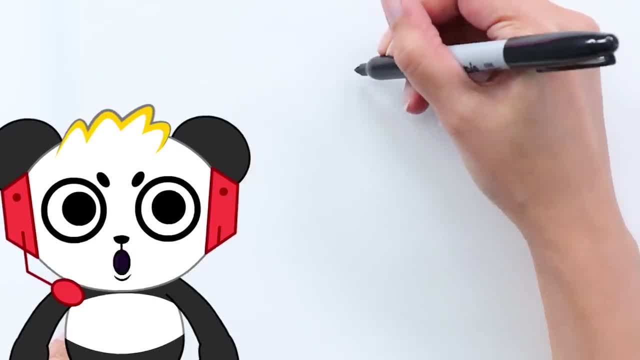 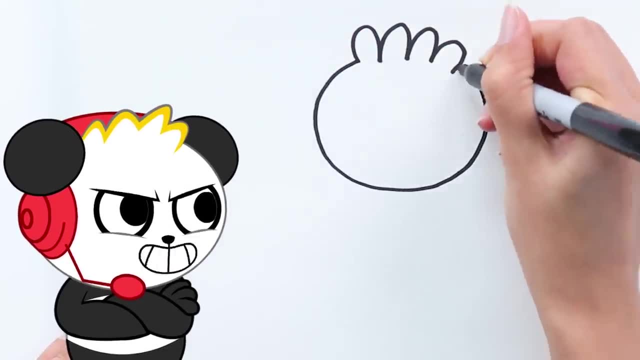 All right, Combo Crew. So we're going to learn how to draw me. So first we want to start with my little tufts of hair up at the top, Then we'll do my big head and got my round ears Not as big as Mickey Mouse's. 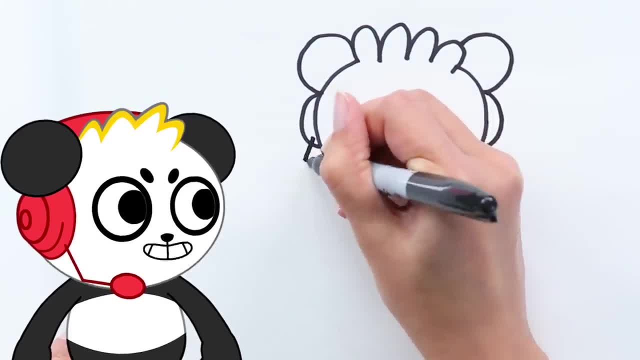 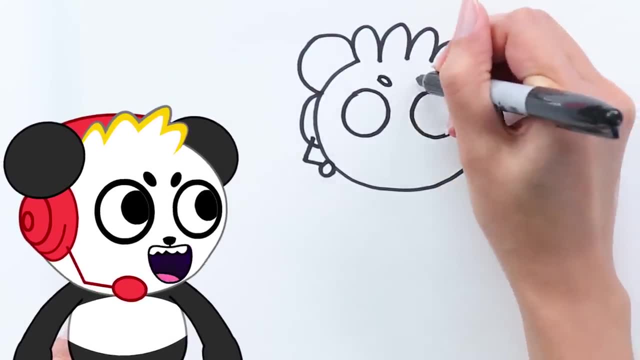 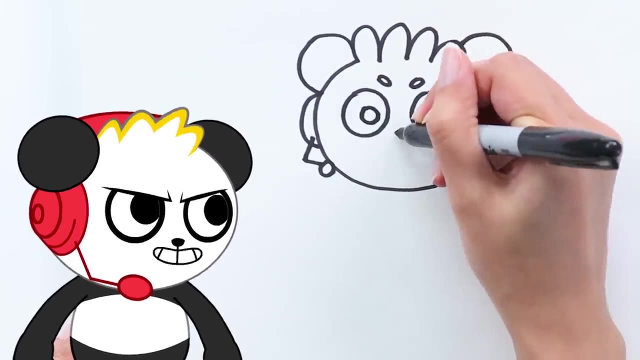 but a little smaller. Then you got my head set underneath, which is like tiny ears and a mic to speak into. Then you got two circles for the eyes- Don't forget two little tiny eyebrows. You got my pupils. Just do a little. 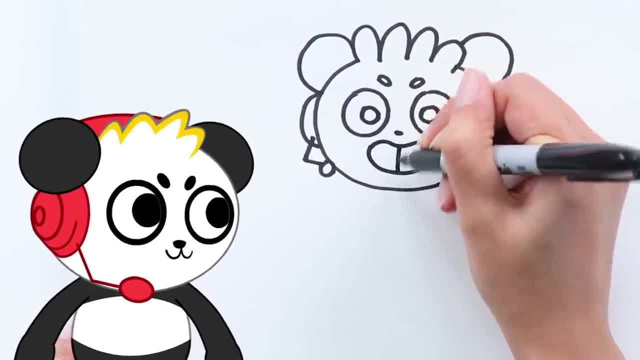 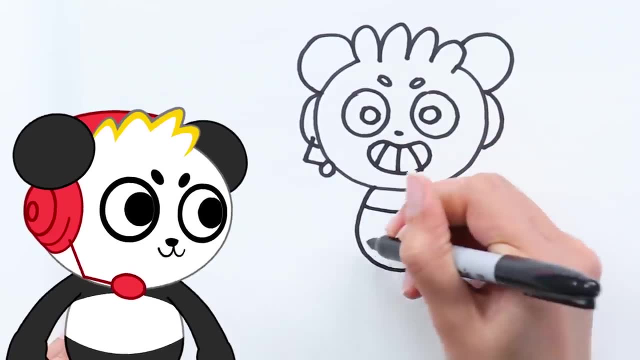 button nose, Give me my nice little smile, Draw some teeth in there. My body's a lot easier than you'd think- Just like a round eggy guy. And then put one stripe on it. Then we're just going to do some simple legs and feet. 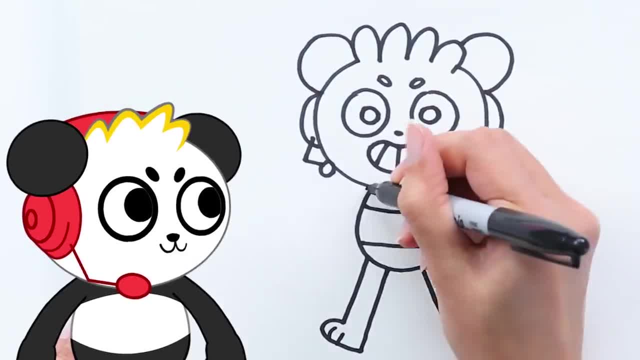 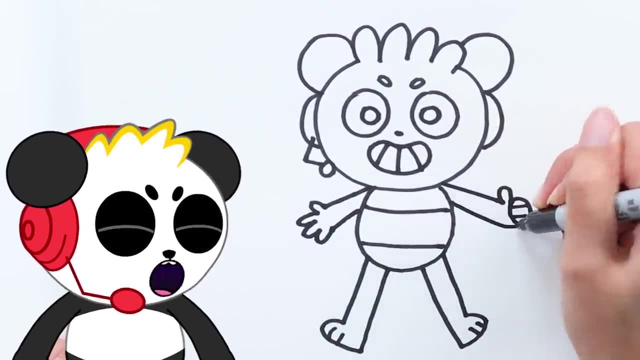 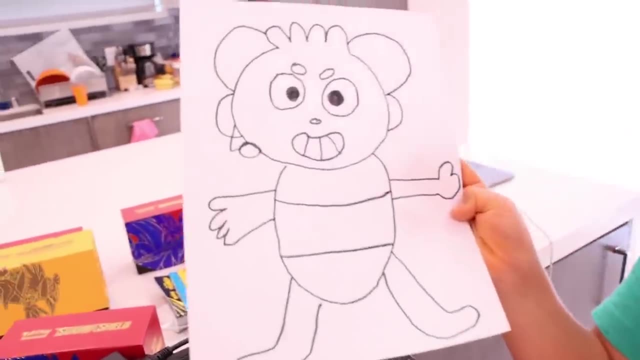 Give me some toes down there. Got my hand over here. We'll do one more hand And I'll be giving you guys a thumbs up for this drawing. Combo Bunga: you drew me. Okay, guys, this is my combo panda drawing. 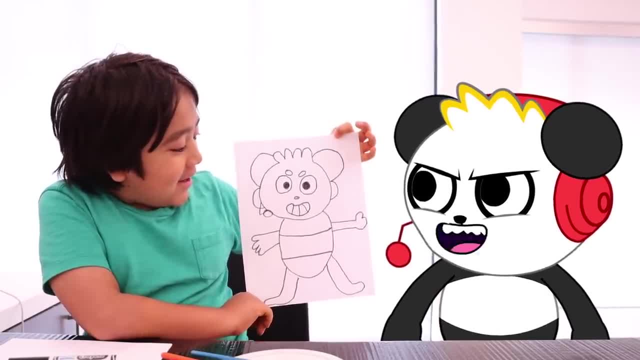 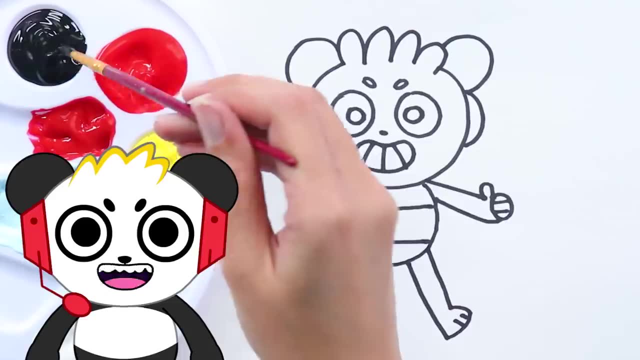 What do you guys think? Wow, it looks exactly like me, Brian, you did a great job. Now let's learn how to paint me. Oh, okay, So now we're painting me. Let's again start up here at the top with the head. 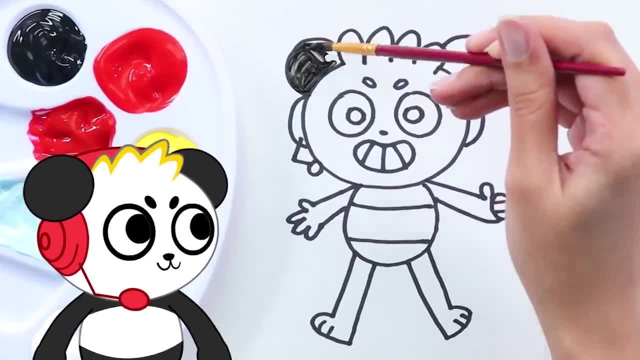 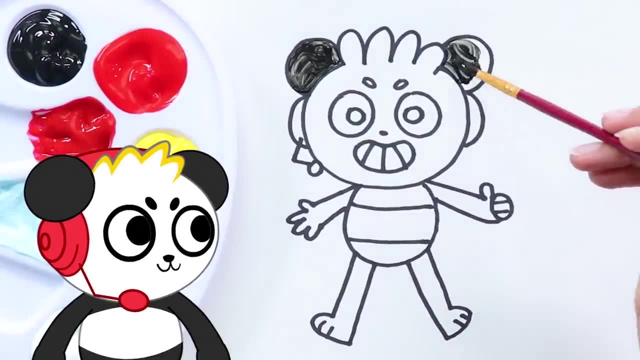 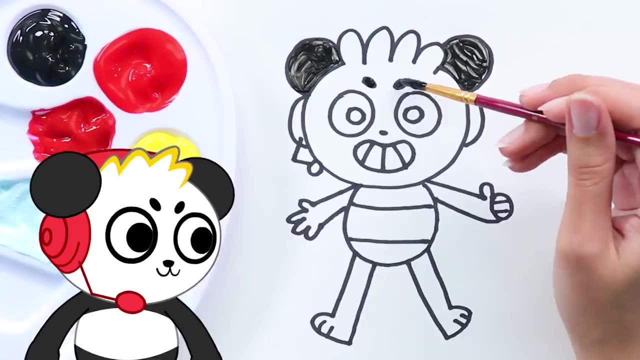 Start with my black ears. Make sure you stay inside the lines, or at least as much as you can. Both ears are black. Inside the lines, inside the lines. Yeah, Combo Bunga, Do my eyebrows. Just need a little tiny bit of paint for those. 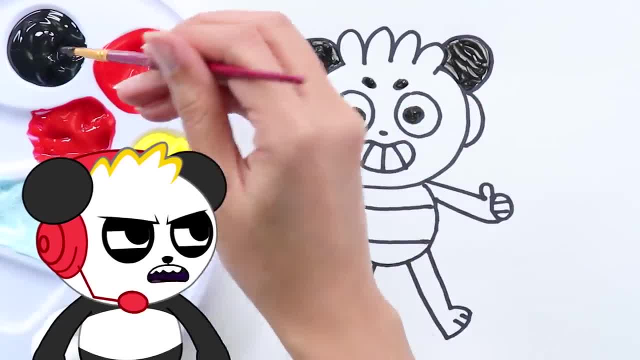 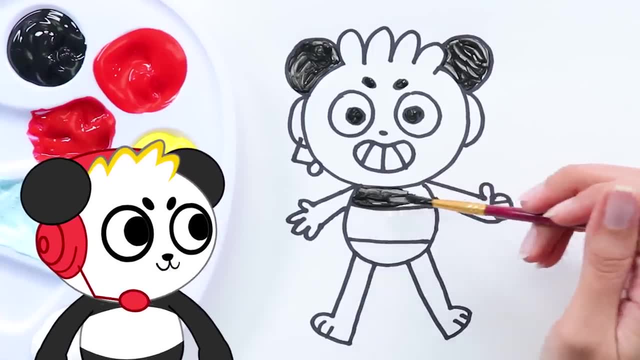 Not much to fill them in. Oh yeah, I got the pupils. What else is black on me? Oh yeah, The body You want to do: the top part of the egg body and the bottom part. My little egg body isn't as colorful. 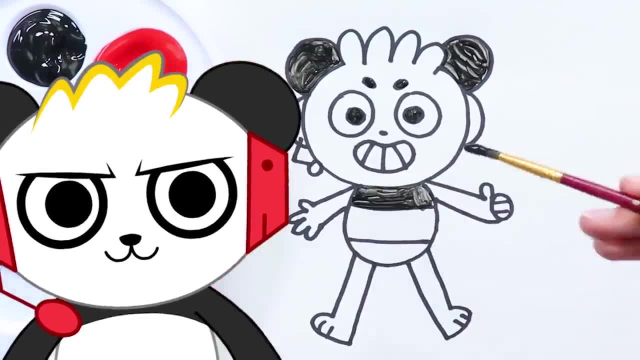 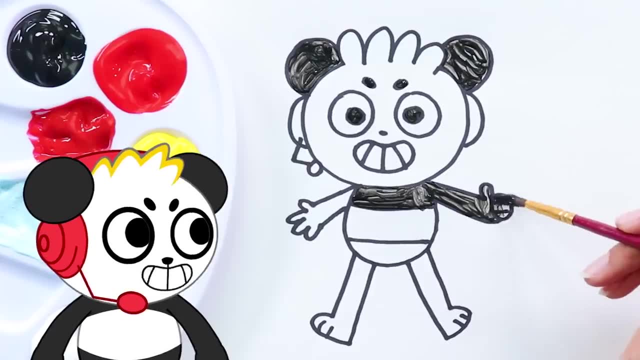 as like an Easter egg, but I'm probably a lot cooler, Might as well. do my arm over here, Get a little bit of my hand. Don't want to paint too much to cover up the fingers, so we'll kind of keep this layer light. 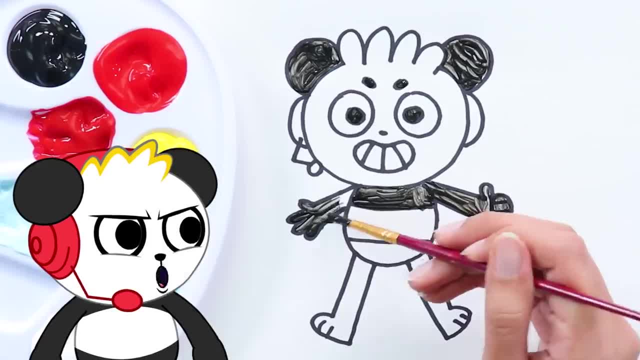 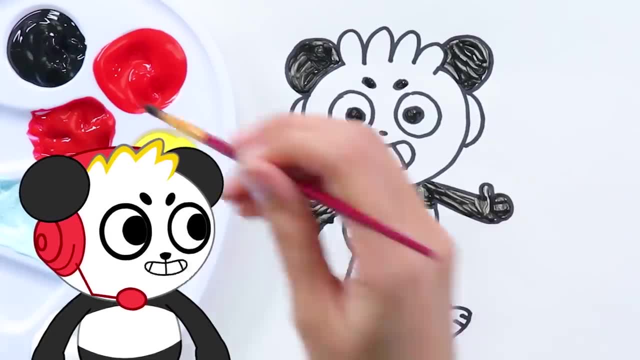 The other hand, should be a little easier to paint, since it doesn't have any fingers, like doing a little thumbs up. Oh yeah, need to get the bottom of the eggy And, last but not least, my combo pants, Or you know. 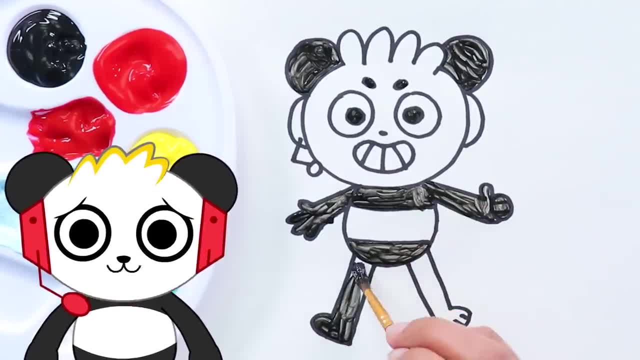 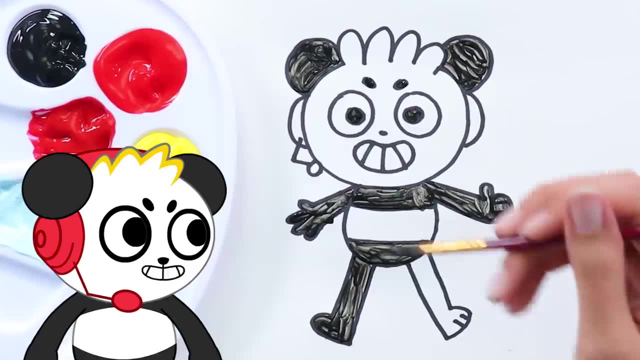 the pants that I was born wearing. Man, I'm so easy to paint. you're already almost done with me. Alright, now let's paint the white parts Done. We're on to the final leg of this painting, Not the actual final leg. 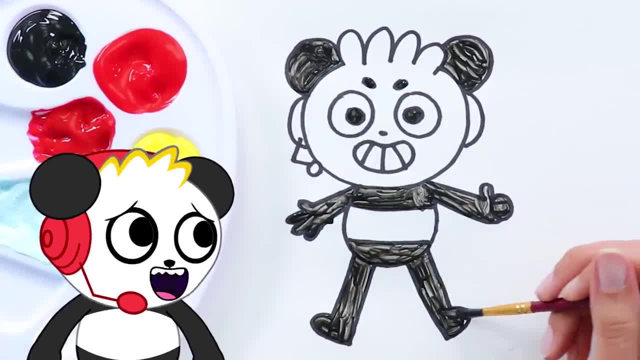 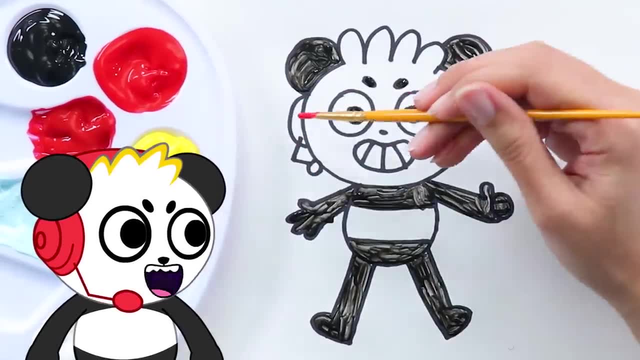 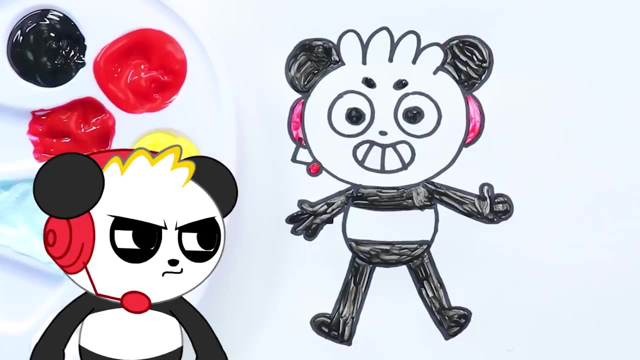 just the final leg. The final leg is the headset. Got to make sure my red headset is in the right place. I'm going to make sure my red headset is perfectly standing out. Give it a nice bright red. Maybe it's a cherry red. 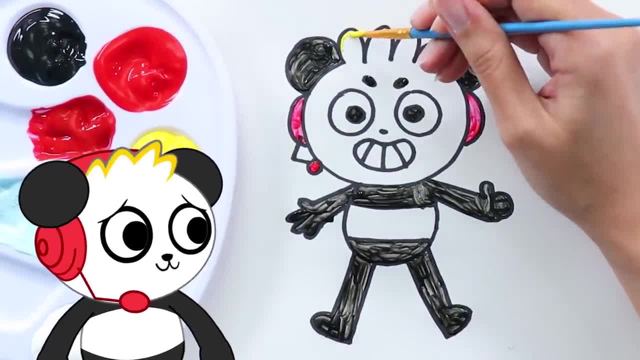 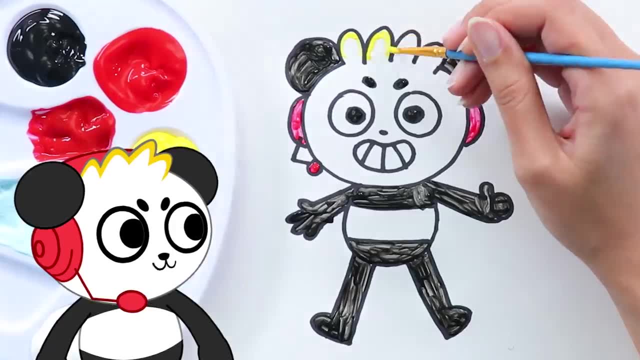 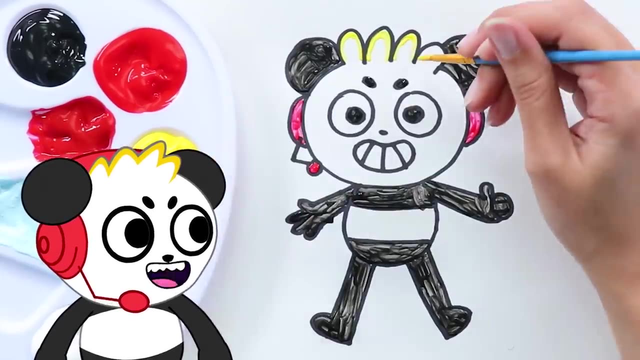 Or a strawberry perhaps, Just not tomato. Oh yeah, combo panda is looking good, But we started with my hair and we should finish with my hair, And the final perfect detail for a combo panda painting is the yellow tuft of hair on my head. 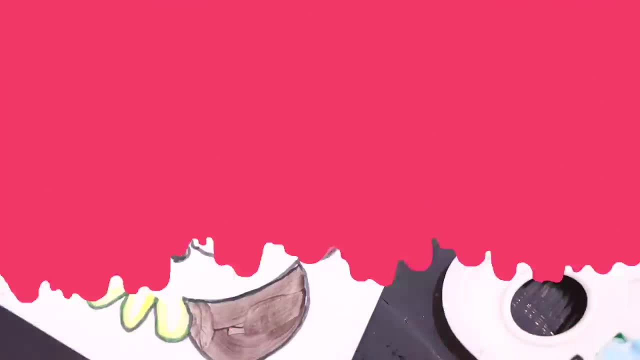 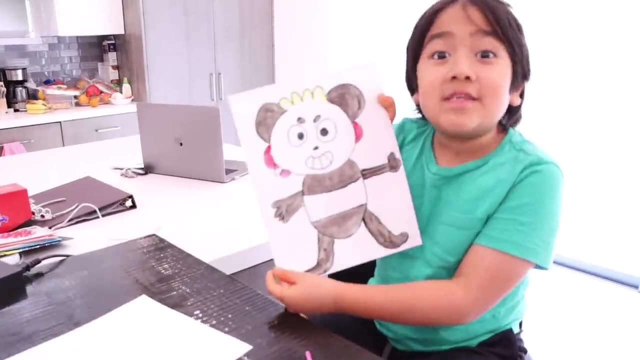 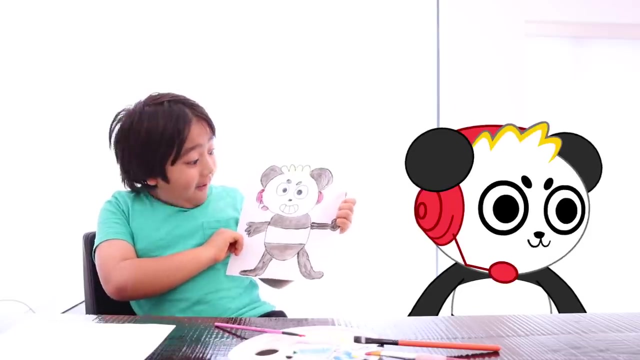 Combo bunga- Combo crew. Okay, just a little bit more Like this. What do you think? This is my finished combo painting. You did a great job coloring me, Ryan. Now it's Gil's turn. Gil, Come here. 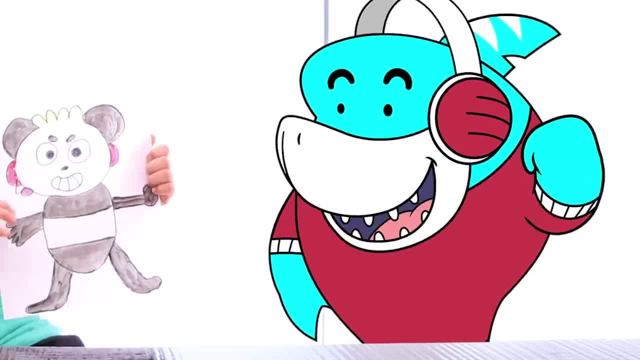 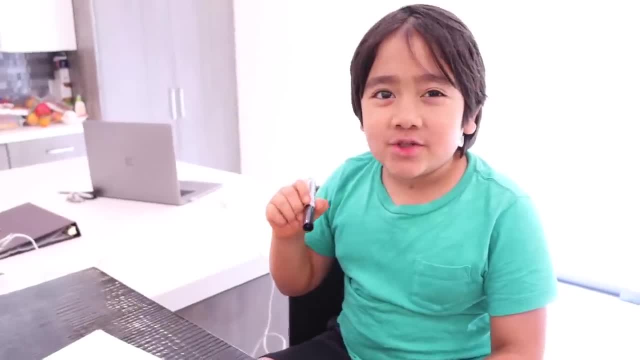 Oh, hi, Gil. Whoa, Ryan, are you ready to paint and color me? Yeah, Alright, me and my friend are going to show you how. Okay, let's get started and draw Gil. Okay, here we go. Start off with a circle. 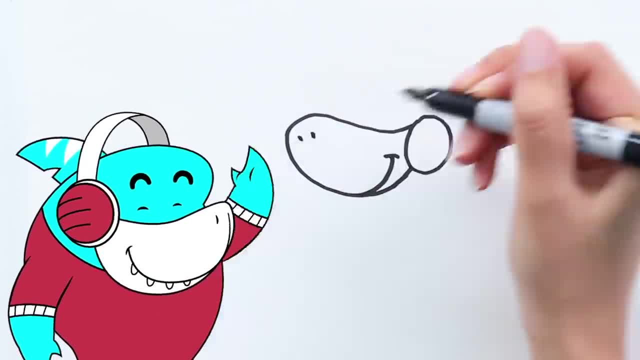 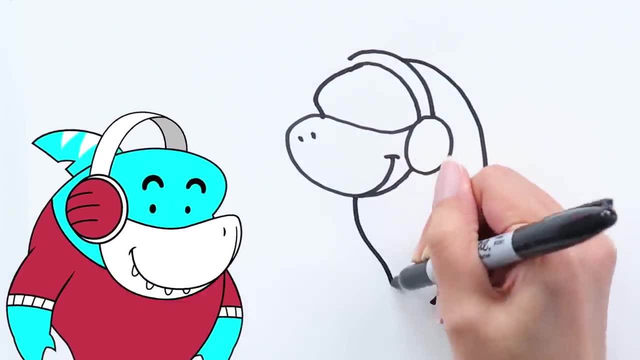 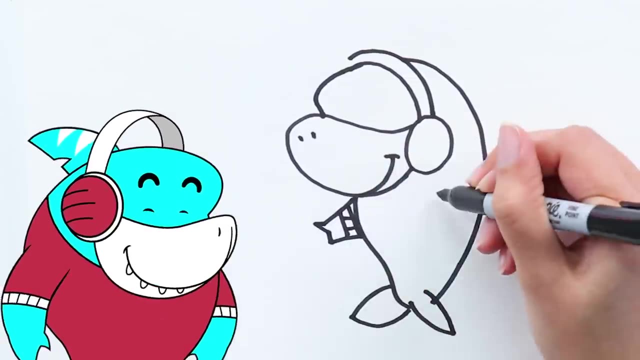 and there's my mouth. Perfect, Okay, now I gotta get the headphones. There you go, Top of my head. and now the body. Make sure you get those fins in there, Nice, Make sure you get the other fins too. Oh, there you go. 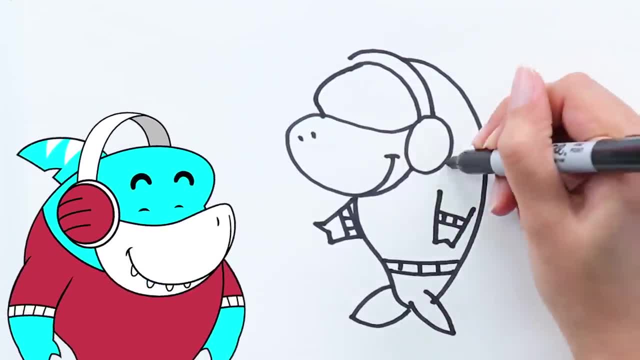 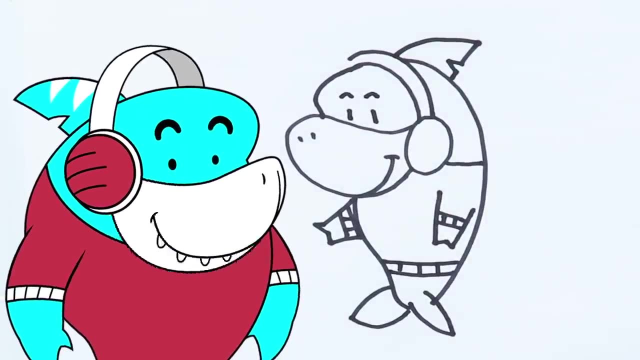 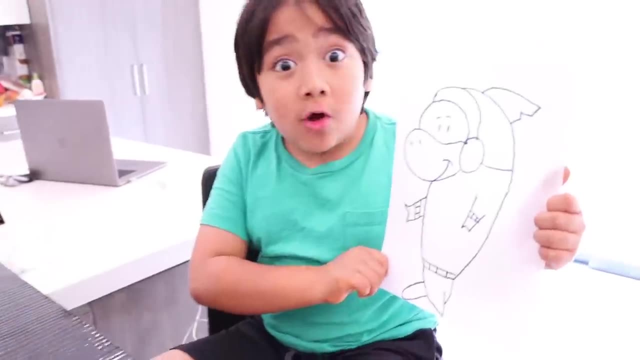 Have the little cuffs for my sweater- Aw yeah. And now, last but not least, the eyes Looking good. Aw yeah, Looks just like me. Okay, this looks really good. This is my finished drawing of Gil Whoa Ryan. 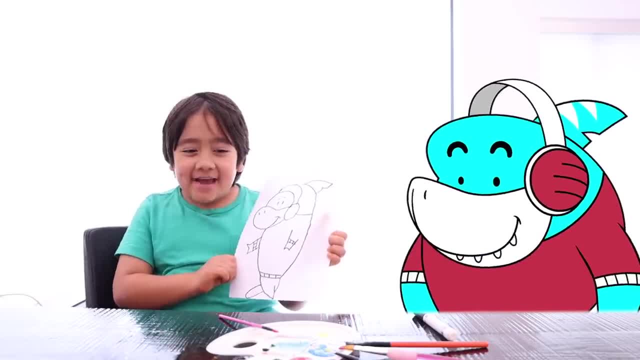 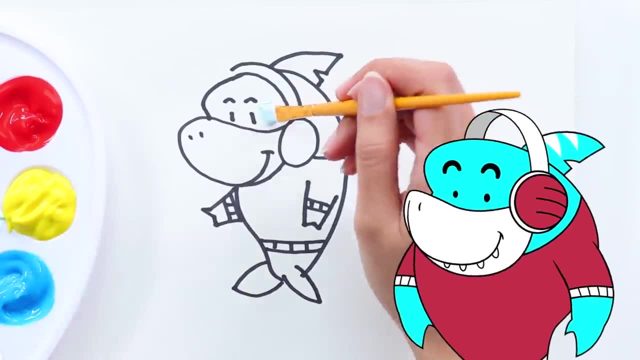 That looks good. Yeah, Let's see if you can paint me next. Yeah, let's do it. Alright, here we go. Get that nice blue Mm-hmm, you're gonna be using a lot of blue dude. 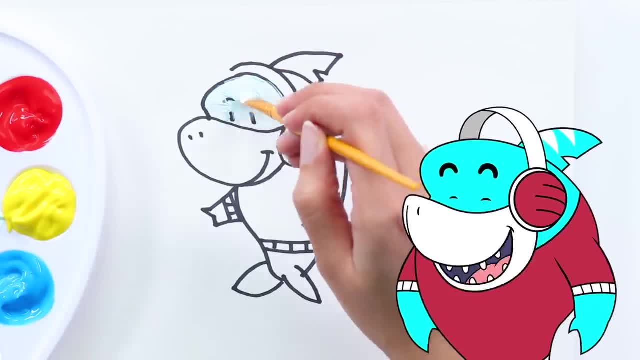 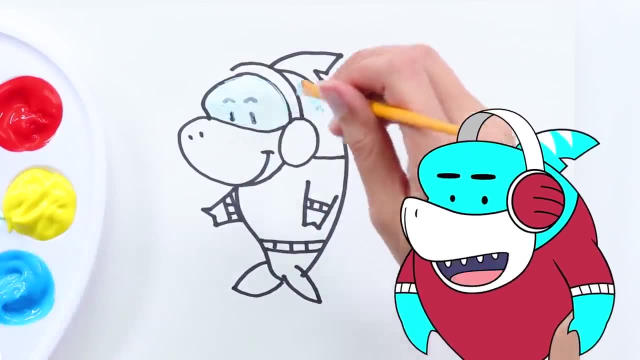 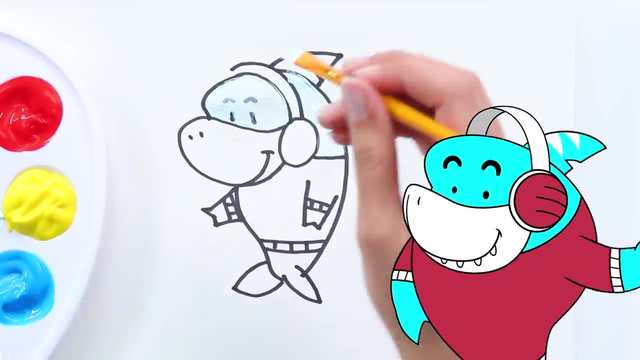 Perfect, perfect, Magnificent coloring, as usual, Mm-hmm. See, it's not like a dark, dark blue, It's more of a lighter aquatic life. aquatic blue for Gilly Right, Gilly gang, Aw yeah. 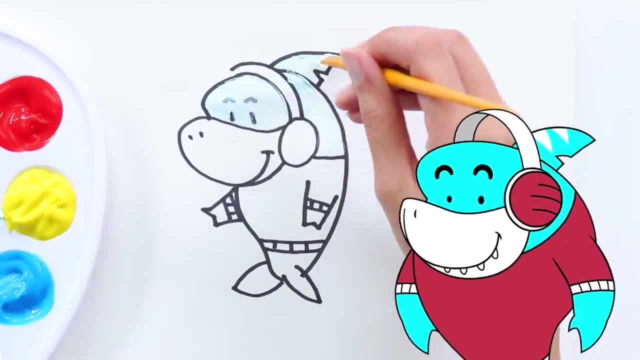 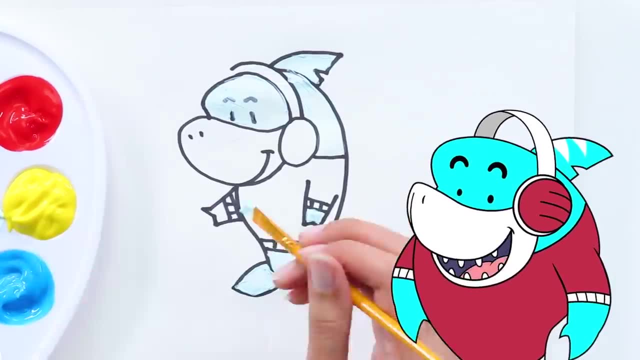 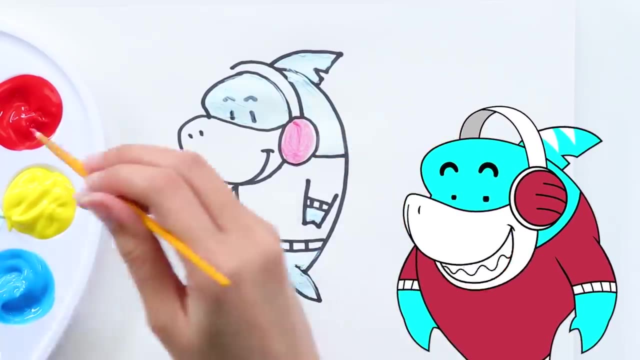 Okay, got my fin. Make sure you get the fin. Alright, the most important part of the shark, The fin. Okay got my little other tiny fins, Hand fins. Well, I do like the red, Nice and red Contrasting the blue. 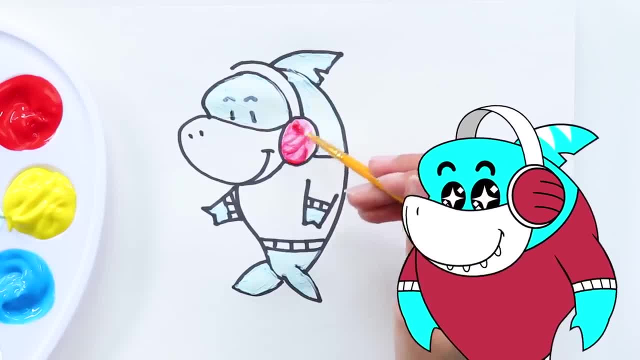 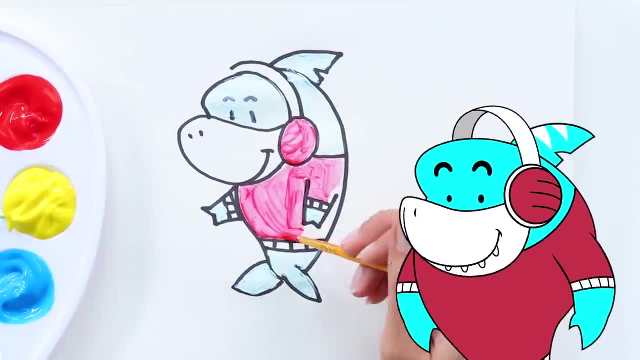 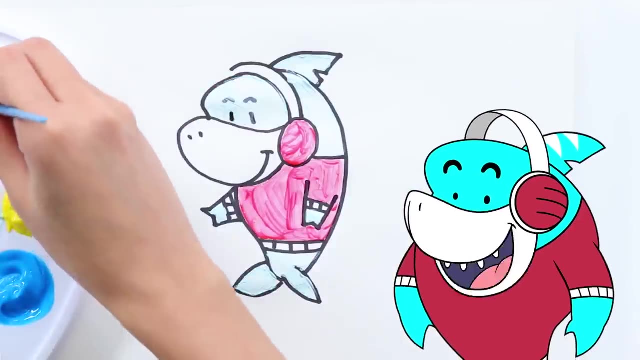 perfectly. It's looking pretty cute, Actually, pretty sweet too. Oh man, it's a lot of red for this sweater. Sweater time, sweater time. Make it red for sweater time. Oh, you're bringing my eyes back, Okay, I. 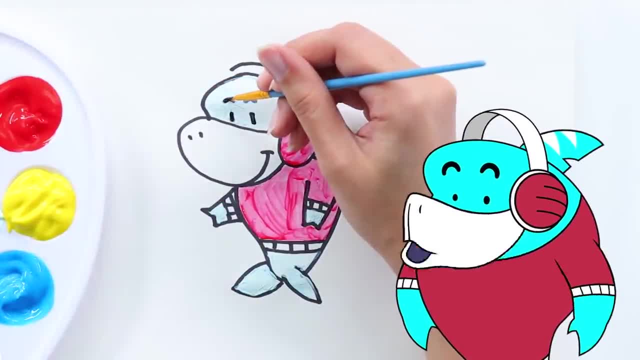 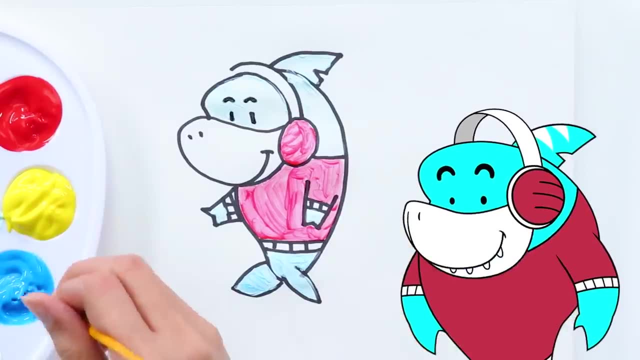 endorse this. I approve Gilly approved. Whew, look at that. Bold lines for a bold Gilly. There you go, Look at that. You know I liked the blue when it was a little light, but it was a little too. 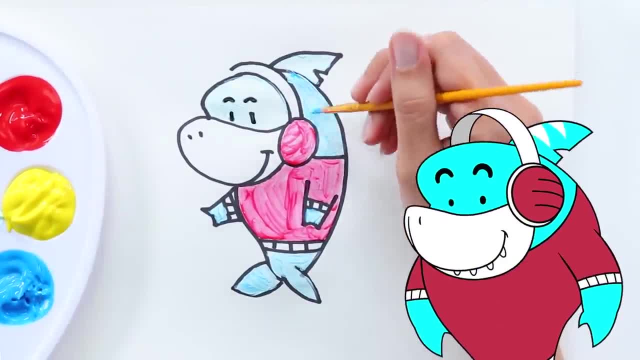 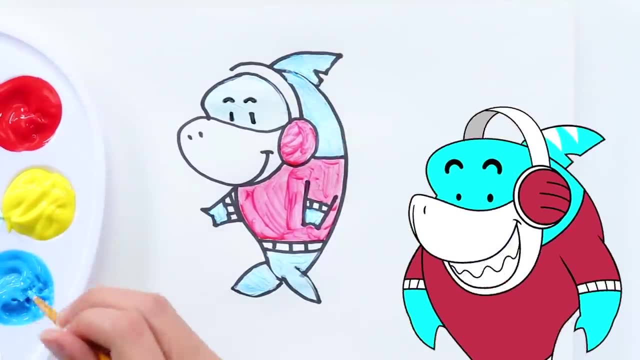 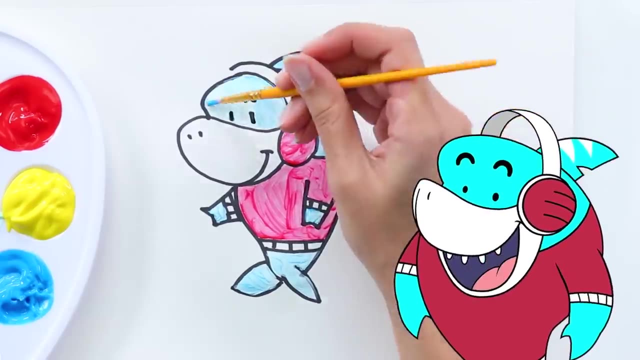 light, Just being honest. But now, oh man, it's magical, It's like it's looking in the mirror, A nice, nice painted mirror. Watch the eyes, Watch out for the eyes. There you go Alright, Almost there, to a true masterpiece. 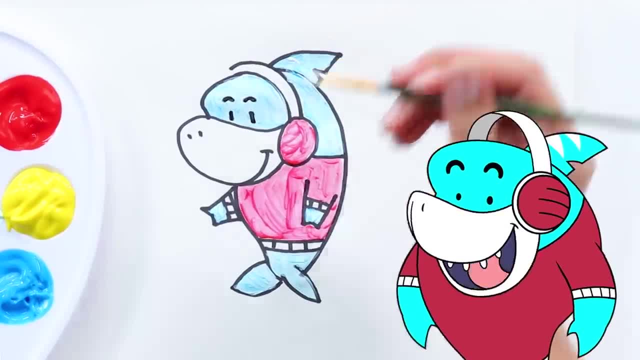 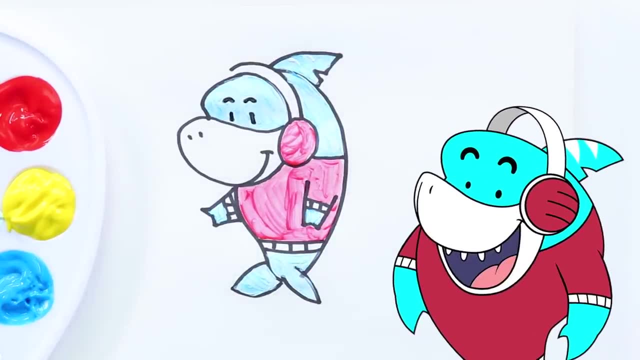 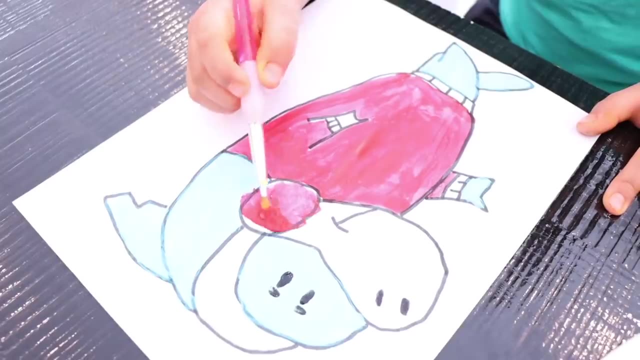 Oh, wow, you're going for my little thin stripes. Okay, Beautiful touch, And this baby looks like it's done, Done-skis. Let's do this last part right here: His headphones, And we're done. Okay, guys, What do you think of my Gilly drawing? 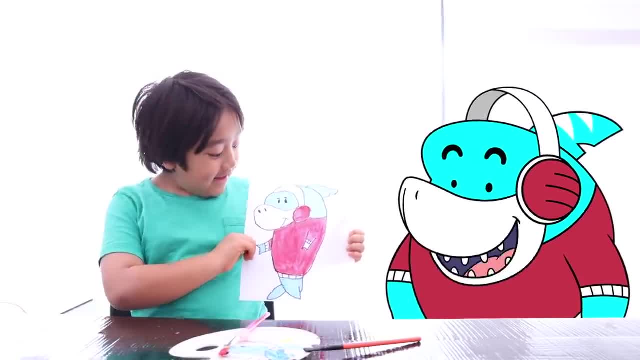 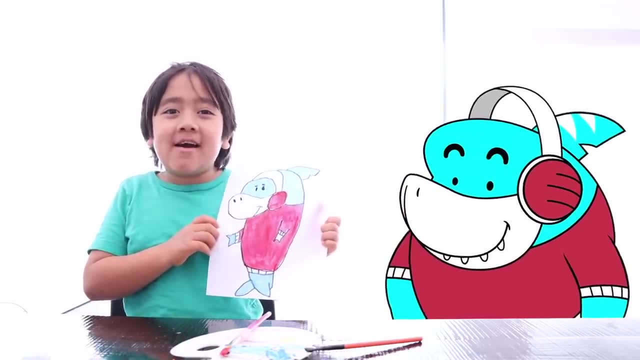 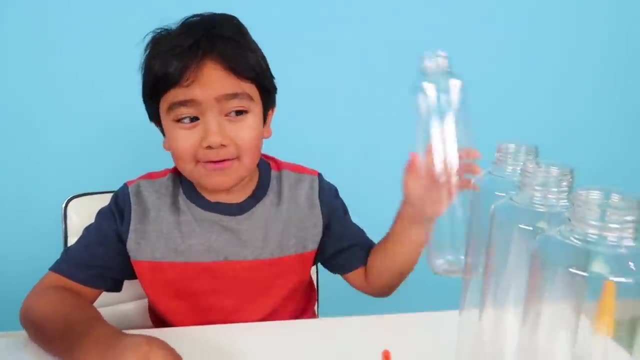 Wow, That looks exactly like me, Ryan. Great job, Ryan. Bye. Thank you for watching our drawing and painting combo and kill video. Hi guys, Today we're going to make fun sensory bottles. All you need is a bottle. 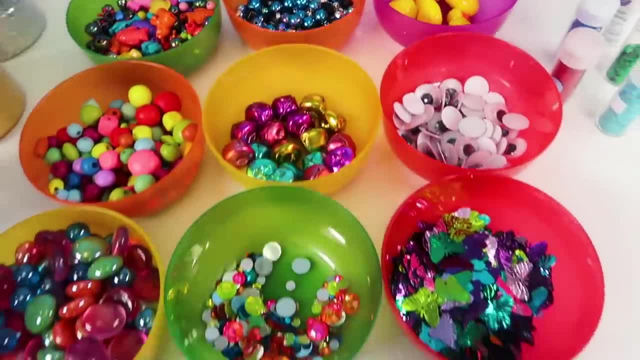 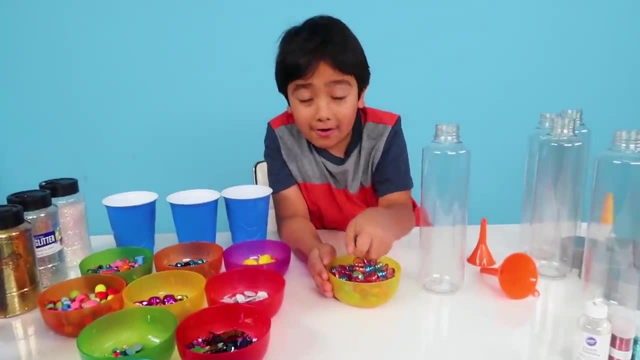 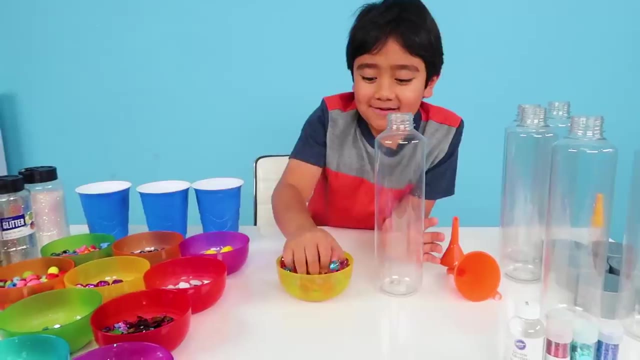 some water and some fun things. First. I'm going to put these in the first bottle, And they're so cool because they're colorful and they're hard. Okay, so you have to put half of fun things in your bottle, Oh. 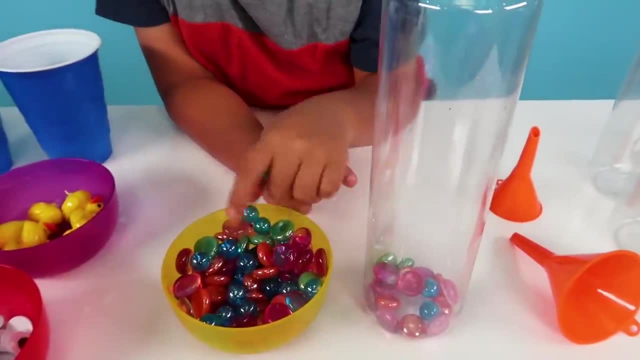 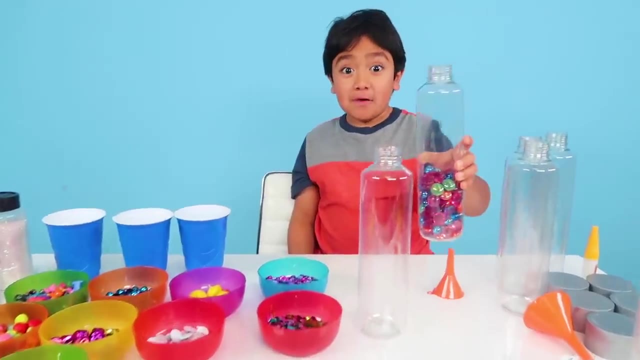 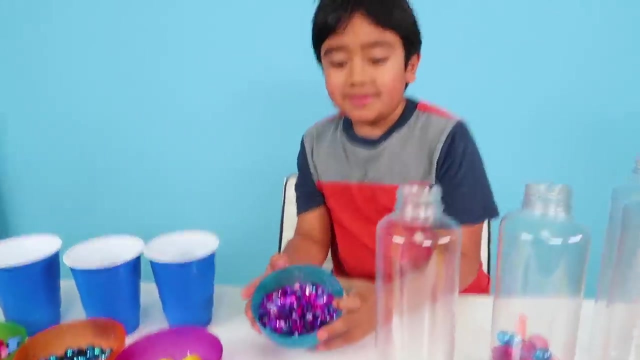 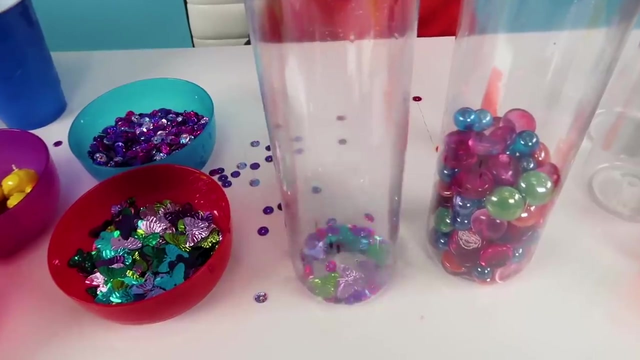 There's these and there's some circles. So this is my first bottle. Later, I'm going to fill it up with water. This is my second bottle. I'm going to mix it with some sequins, and some butterfly sequins. Okay, so my second. 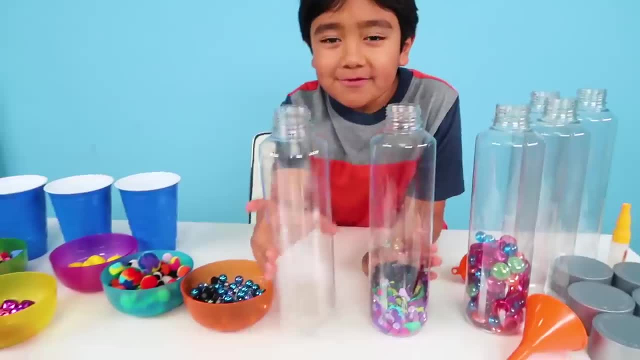 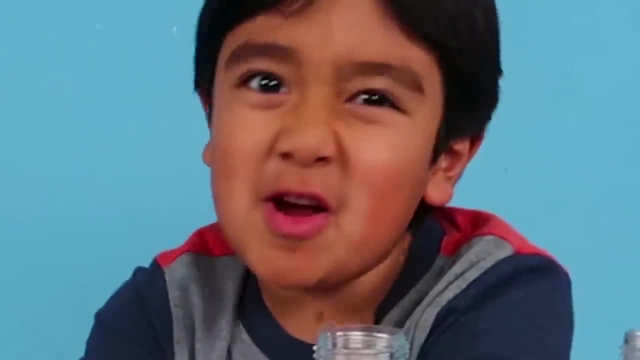 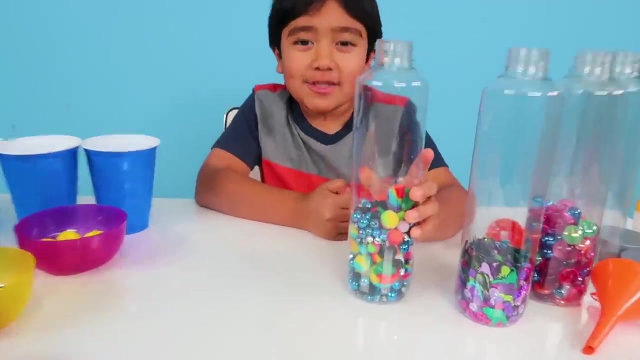 sensory bottle is done And now I'm going to do the third one. So I'm going to mix these and these Start the combined mixing. Okay, so my third sensory's almost done. I got four more, but look, I got most. 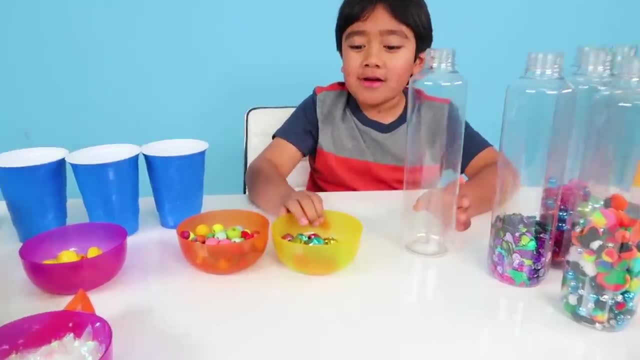 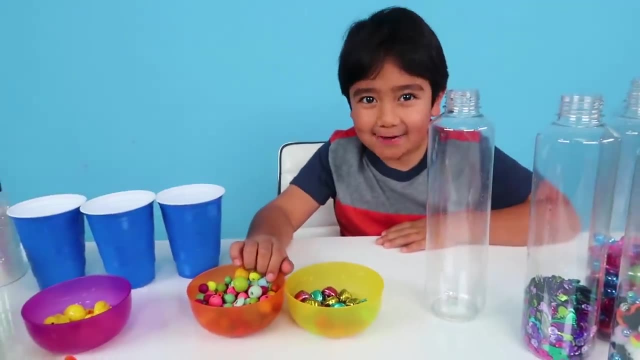 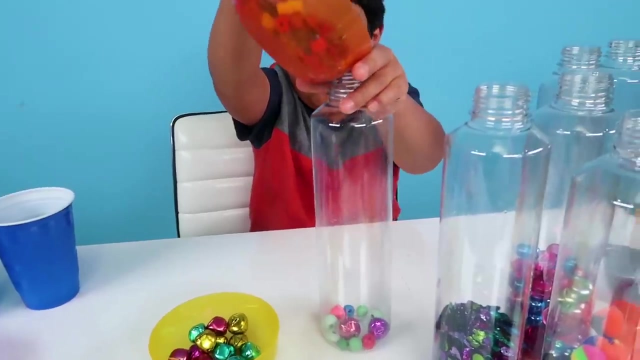 Whoa, For our fourth sensory bottle. we're going to get some bells and some more balls, But for this one we don't need any water. Ooh, I can put all of it: Whoa, whoa, whoa. 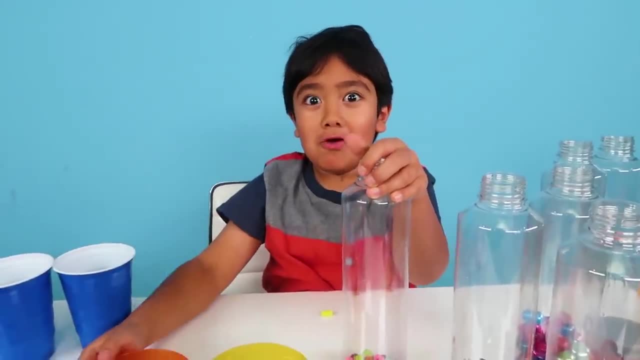 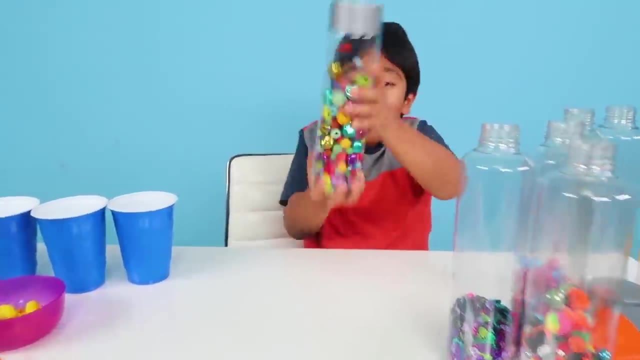 Wait, wait, wait, wait, wait, wait, Oh Uh-oh. This one's fun and I'm not going to put water in it because it's fun without the water. For my fifth one, I'm going to put a. 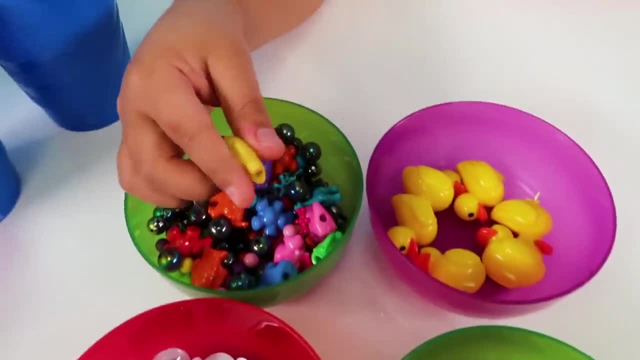 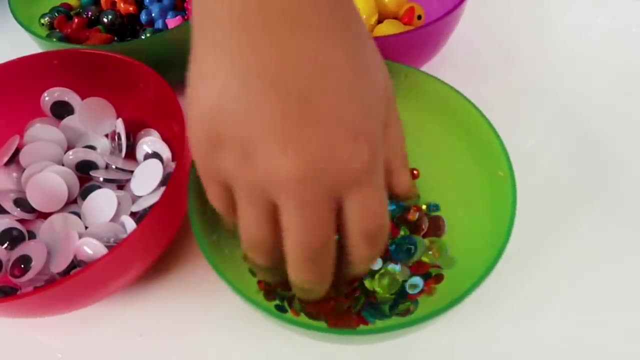 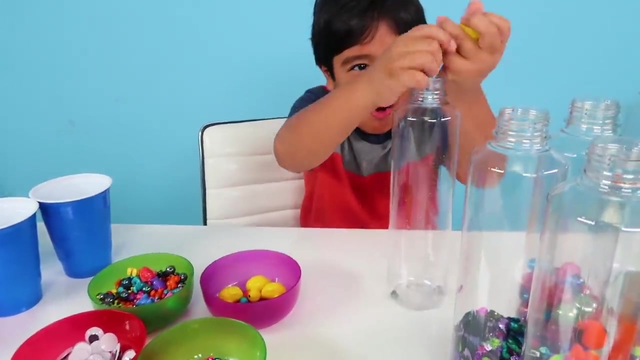 combination of all four of these And with the water it's going to be fun, because I have fishies, duckies and eyeballs And I have some of these which are probably like sticky sequence things. Let's start. Oh, oh, oh, oh, oh. 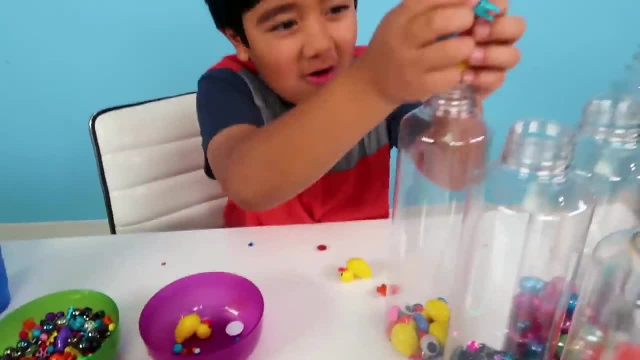 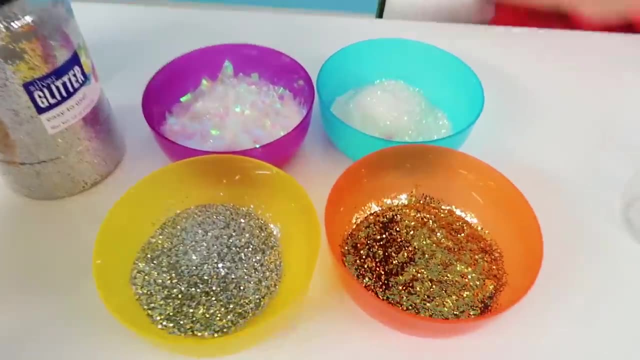 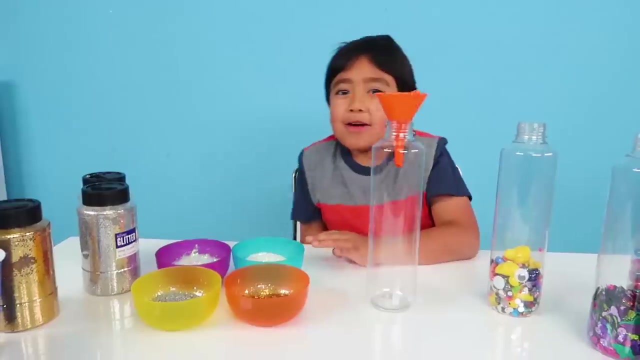 Oh, oh, yes. Okay, number five is done And the last bottle. I'm going to use a lot of glitter, Whoa Glitter party, And it's done. Okay, now let's put it in. So I think. 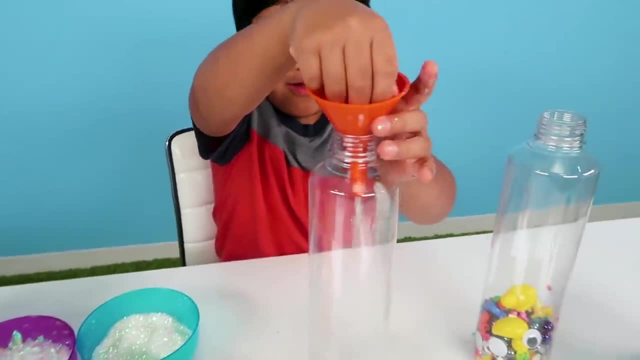 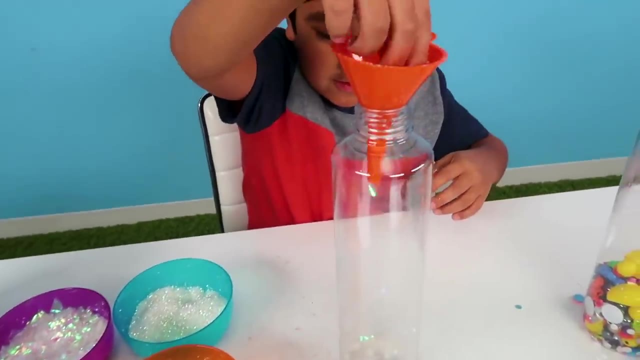 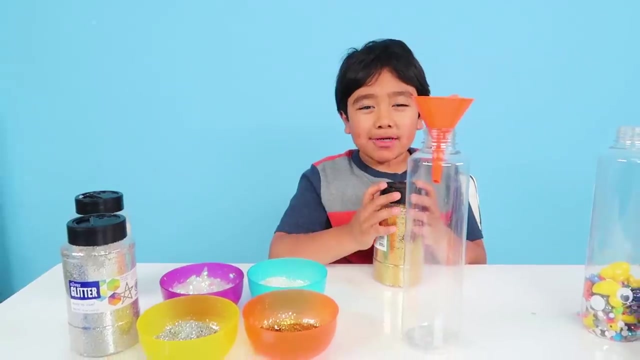 I'm going to get this much Maybe. Oh, I need a lot more Okay, a little bit more Perfect, And then some of these Whoa Silver. Now I'm going to do gold glitter. Ooh, Whoa. 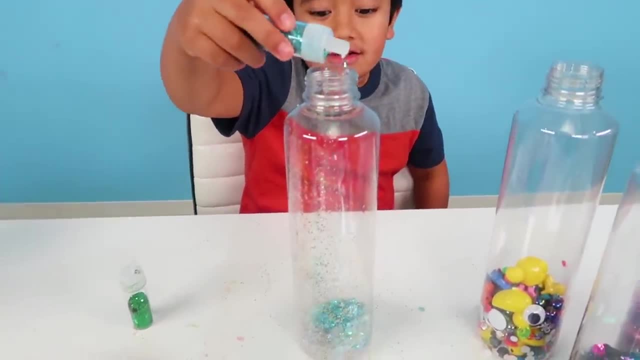 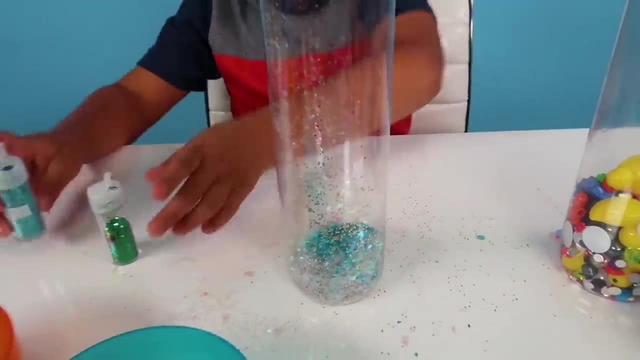 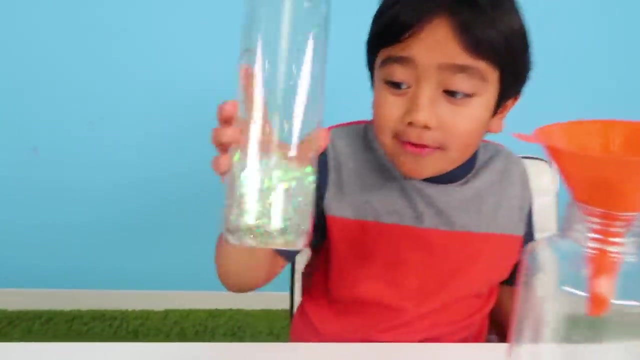 Okay, let's put an extra color of glitter in. Ooh, Okay, and now we're going to put some green Whoa. Okay, so my last sensory bottle is done. Okay, now. next we have to put water inside. 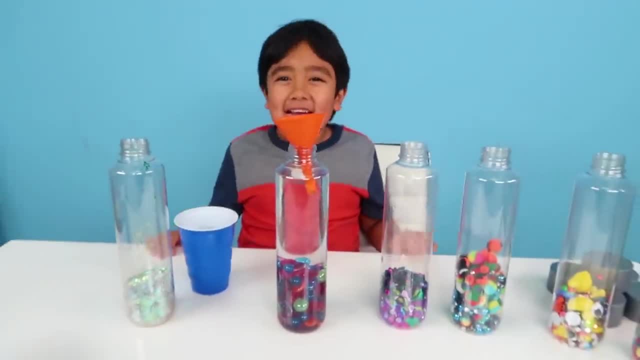 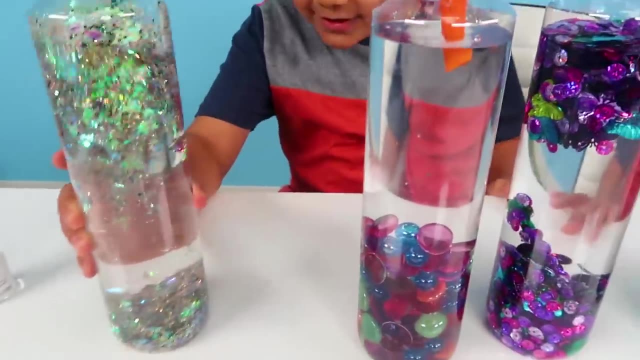 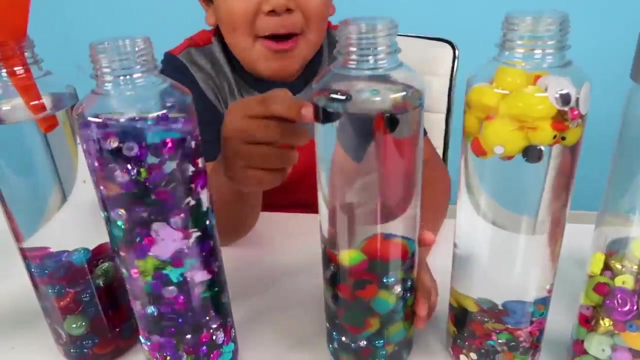 Ooh, Whoa, Yay, Let's do the other bottles. It's done. I filtered all the water. Ooh, And look at this, it's falling down. Whoa, Whoa, Oh, look, and Moe's on. 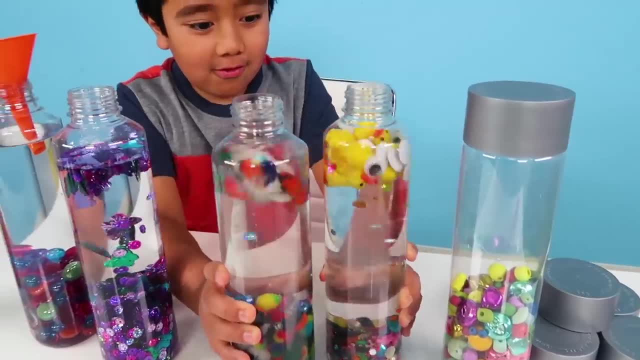 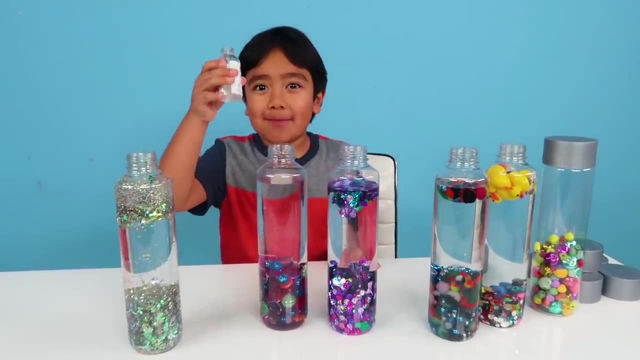 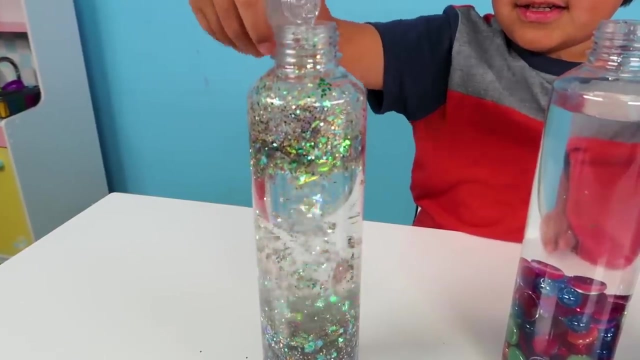 the top, Baby Moe and Big Moe. Ooh, I don't think I can make the duckies go down. Okay, the last step: You have to put glycerin to make it thicker. Okay, I think that's good. 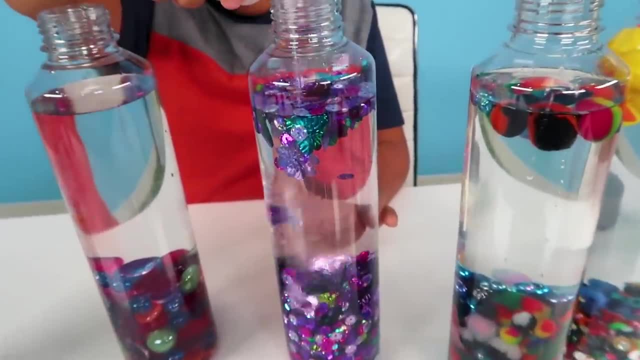 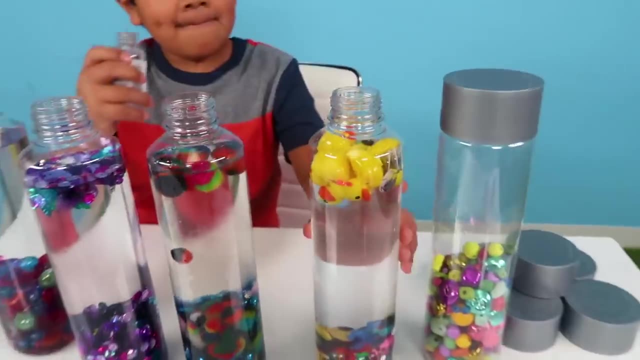 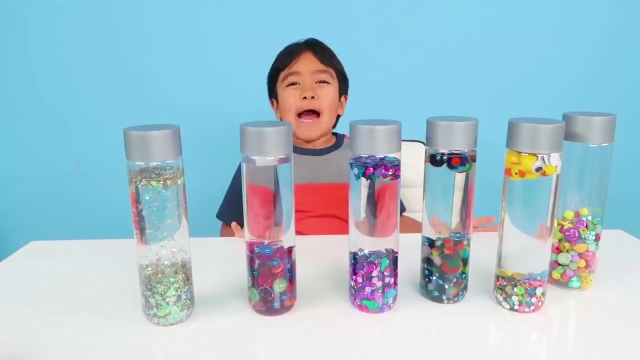 Okay, and then this one- I think that's good, And then this one, That's good, And one It's just going to fall on the duckies. Okay, that's good. Now it's time to mix it together and 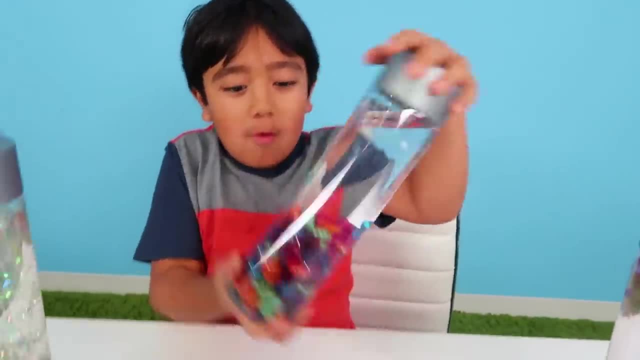 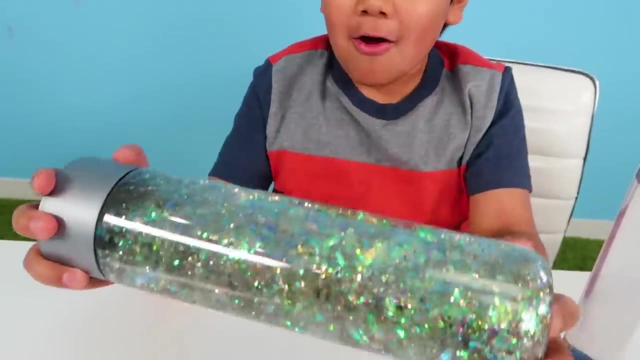 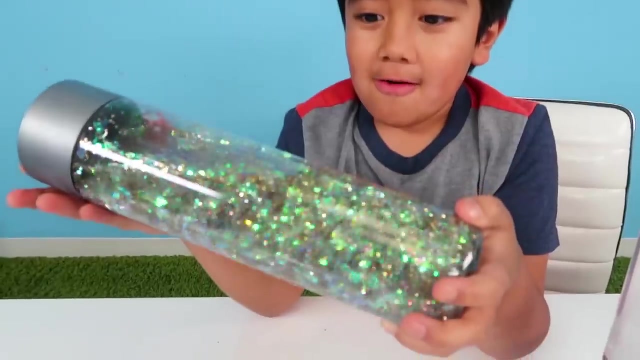 shake. Whoa, Whoa, Go, go, go, go, Whoa, That's so much glitter. Whoa, It's mixing the glitter in the water. Look, Whoa. And now we're going to do the sequence. 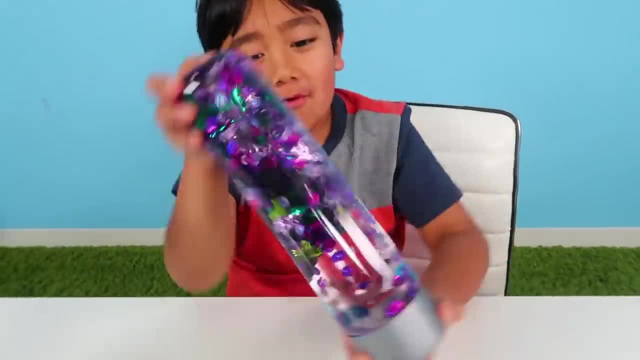 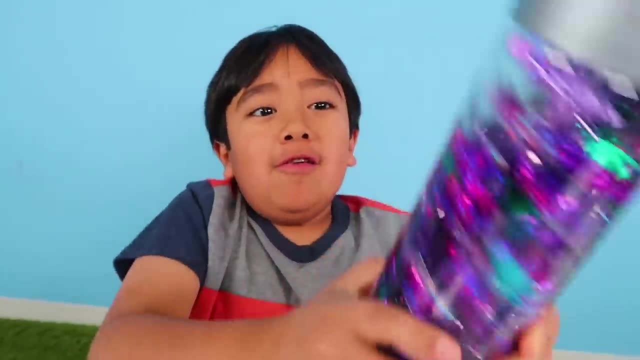 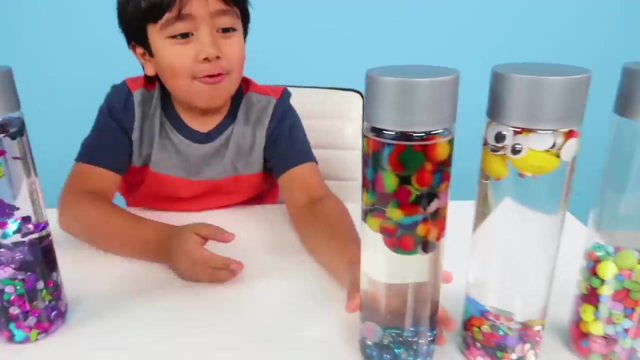 and sequence butterfly. What if the butterflies fly? Whoa What? It's like a tornado: Whoa, whoa, whoa. And this one with a bunch of moes. Oh, they're all separated, We're mixing them. 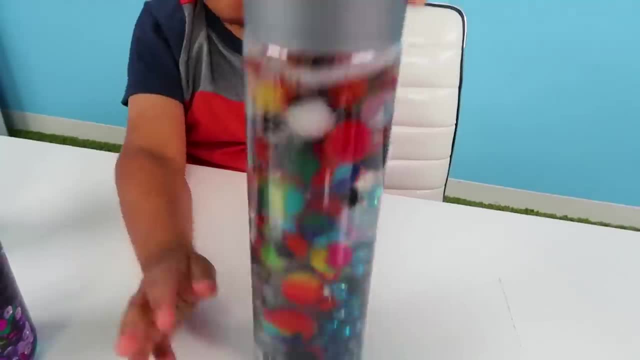 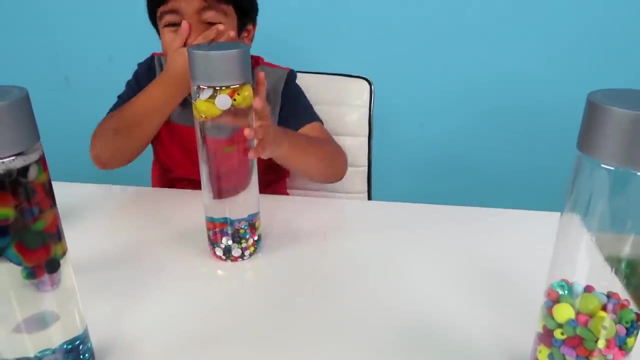 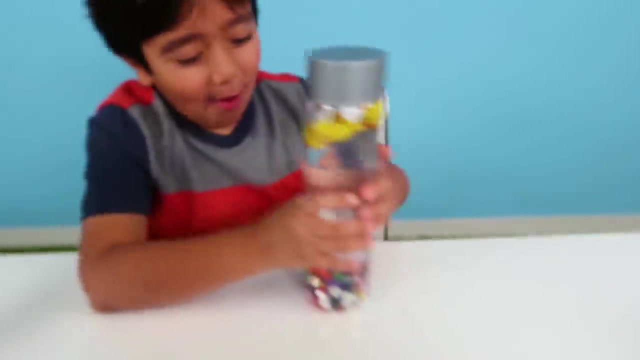 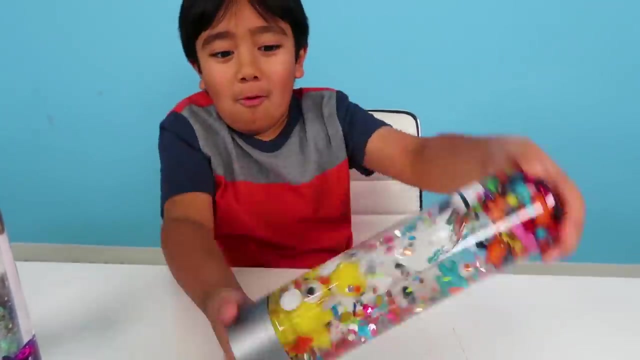 Whoa, Whoa, Whoa. They're separating again. Now let's do the rubber ducky one. See this body. It has a giant eye. It looks funny. Yeah, Keep switching sides. Whoa, Whoa, Whoa. 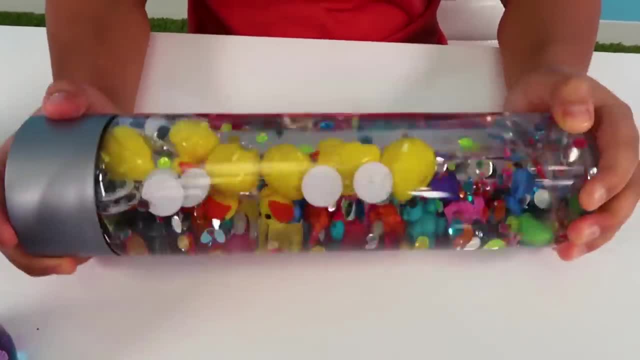 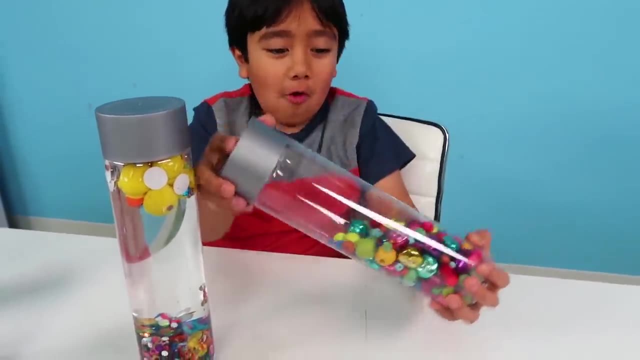 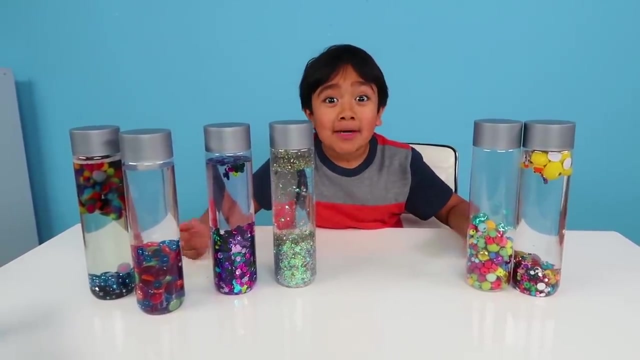 Shake, shake, shake. And now for this one, that we don't need any water for Whoa, Whoa. This is so cool. I'm going to bring it to Emma and Kate, my sisters. Let's go. Whoa, shaky powers. 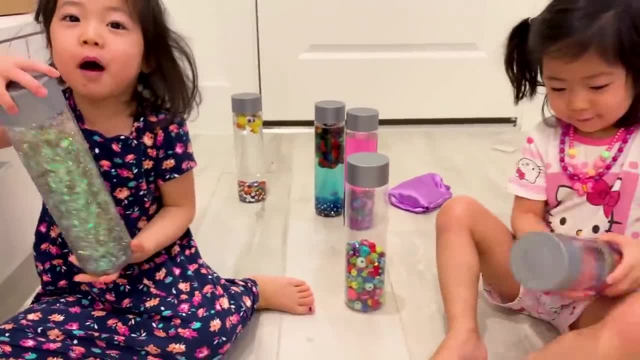 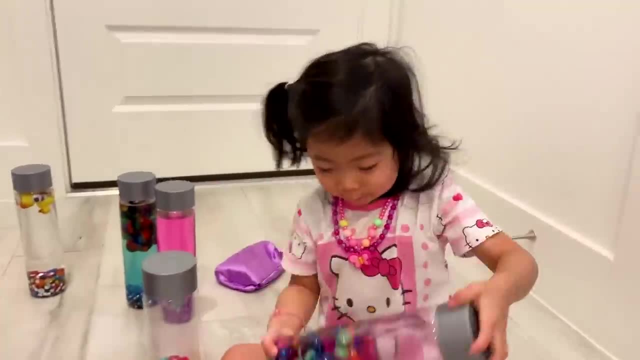 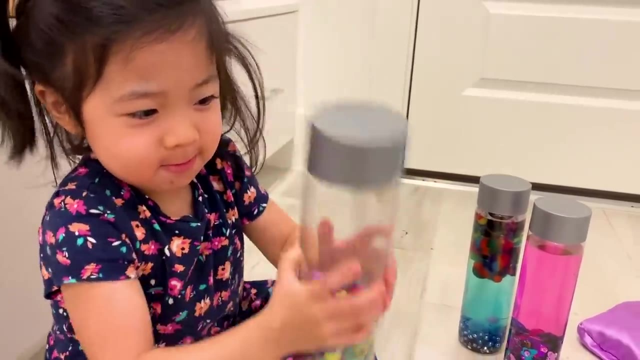 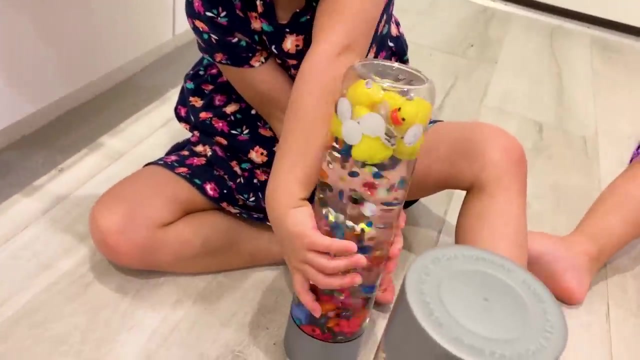 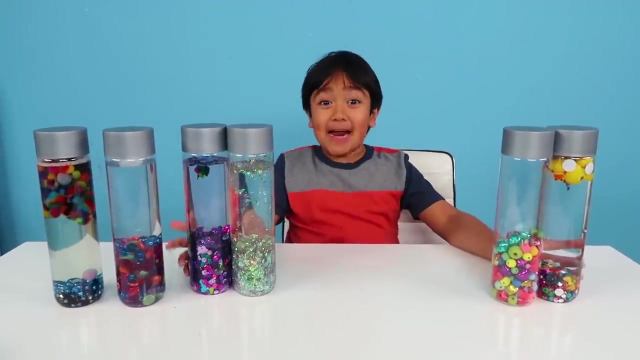 Yeah, Do you like it? Who bought it? Ryan made it. He made it for us. Yeah, Thank you Ryan. Thank you, Ryan. Ooh, Yay, It's very, very light. We're going to do the last step. 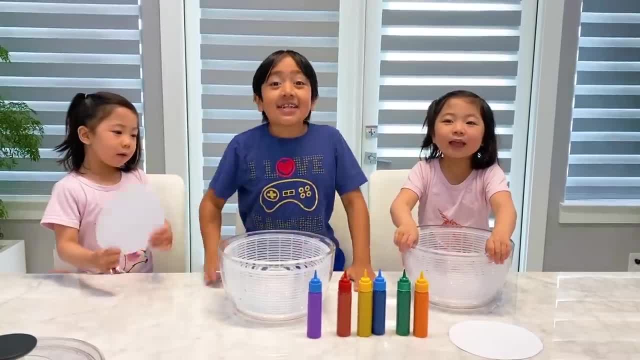 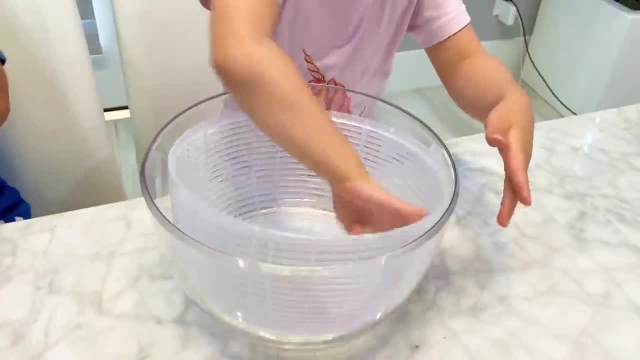 Thank you for watching our sensory bottle video. Hi guys, Today we're going to do the salad spinner art. Why? Because we're using a salad spinner and we're going to spin it. First you need a round circle paper. 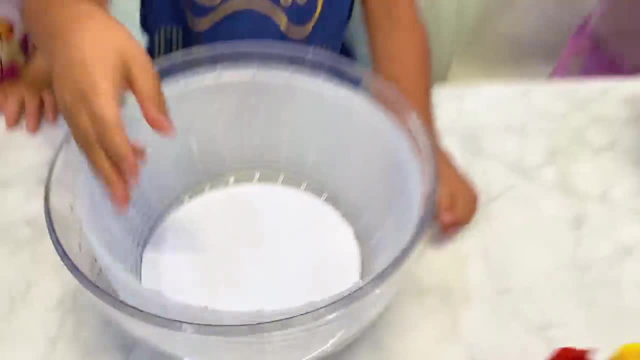 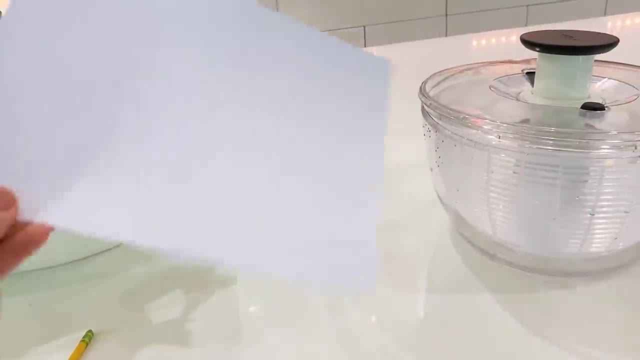 Put it in here. Put it inside, but don't forget to unhold it. So this is how you make a circle paper. All you need is some cardboard card paper, and then from the salad spinner you take this out, then you put it on your sheet of paper. 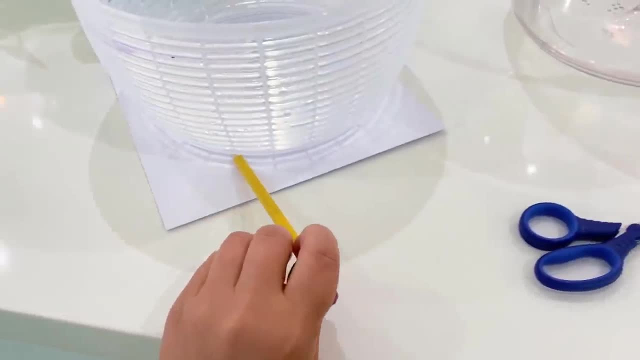 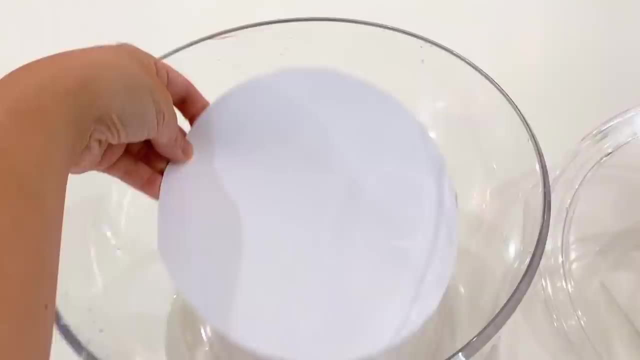 then you just trace a circle around it. Then, once you're done with the circle, then all you do is just cut it out. Once you cut it out, it looks like this And it's perfect to put in the bowl. Can I help? 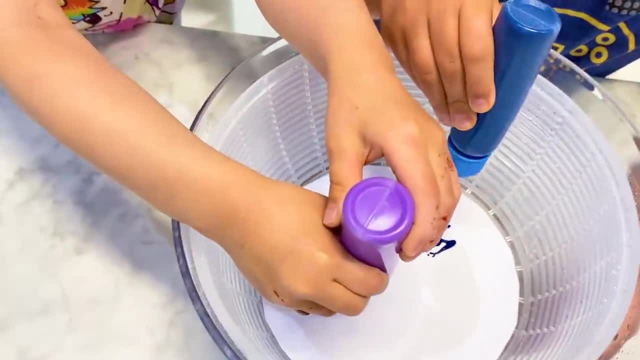 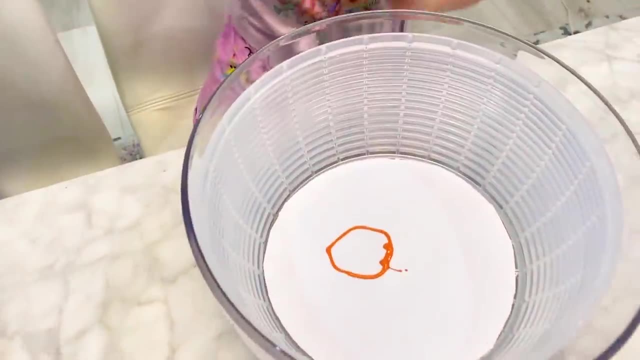 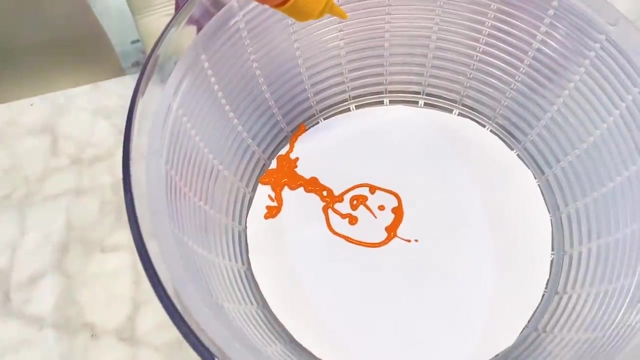 Yeah, of course, Kate, I'm going to draw, I'm going to draw somebody, You are See, this looks like somebody, right, You did it? Oh, I love it. Am I Oh, together It's. 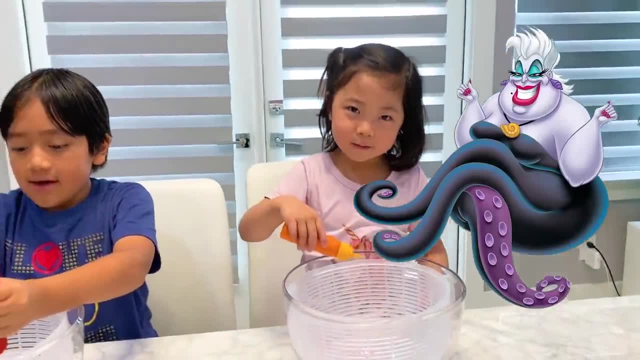 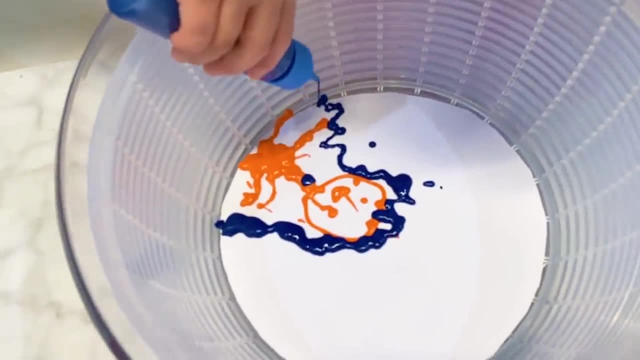 Oh I love it. It looks like a person, Emma, But not a person. It's Ursula. Oh, Ursula, Whoa, Do you want to try a different color? Oh, I love it, Emma. Oh, it's so cool guys. 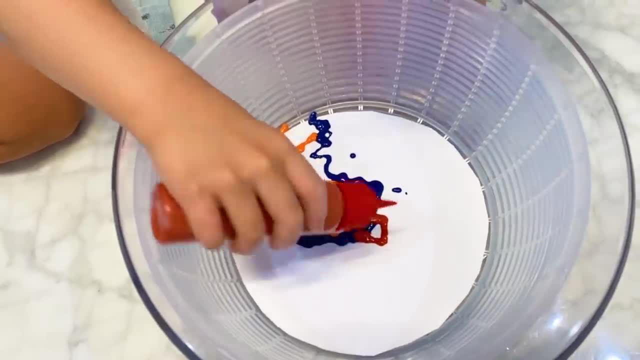 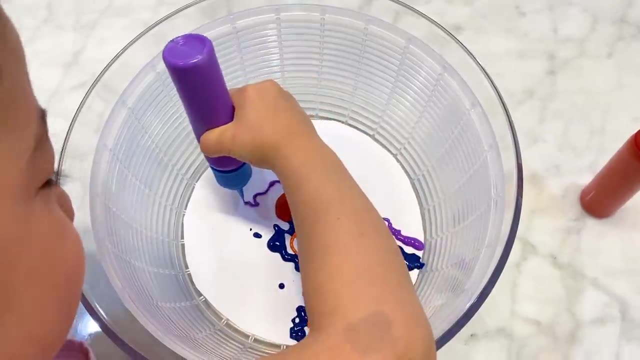 I need red. Oh, I love how Emma's drawing a painting in here before we spin, Love it. Whoa guys, that's a lot of paint. Look at this paint-ness. Oh, I like it, Love it. 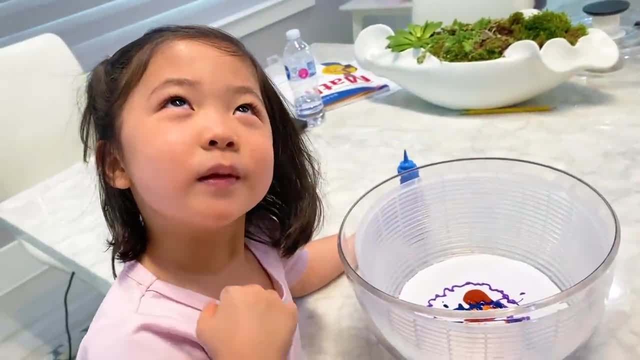 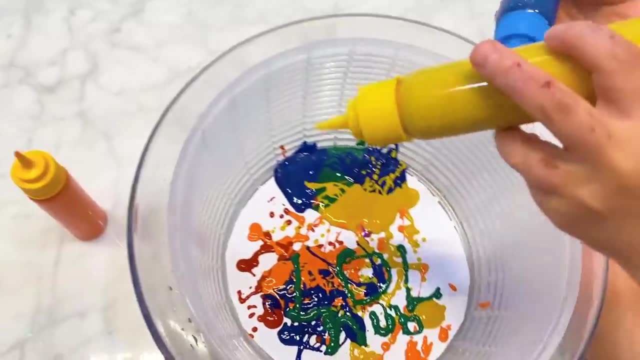 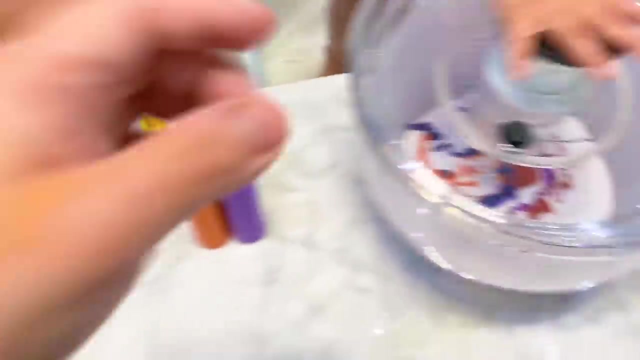 I don't know What is that? Her, Her life, Her hat? Nope, I already got a hat. Oh, I love it. Whoa you guys done now? Yeah, You gotta spin away guys Here, Emma, I'll help you. 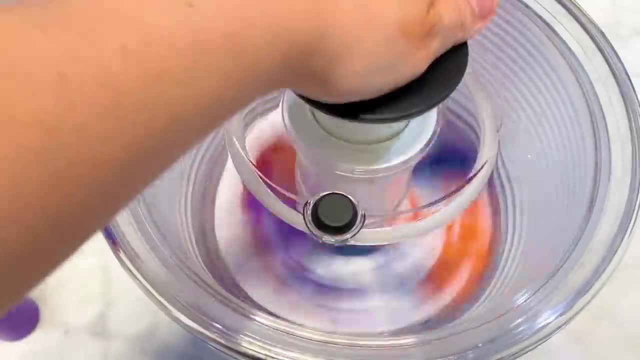 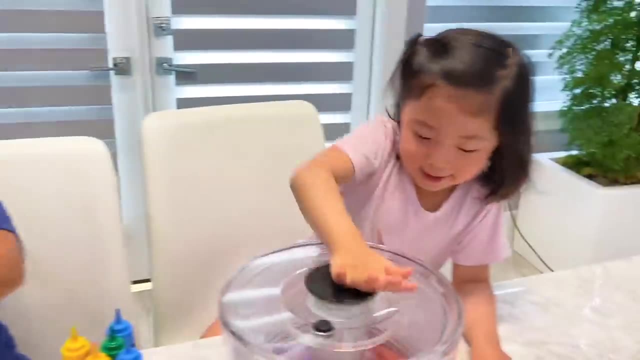 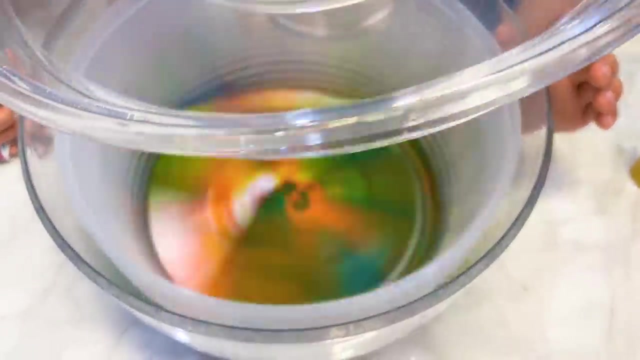 You gotta close it and then you gotta spin Like that. see, I'll try. Yeah, try it. There you go. Can I see it? I know Whoa guys. Let's see what it looks like Whoa. 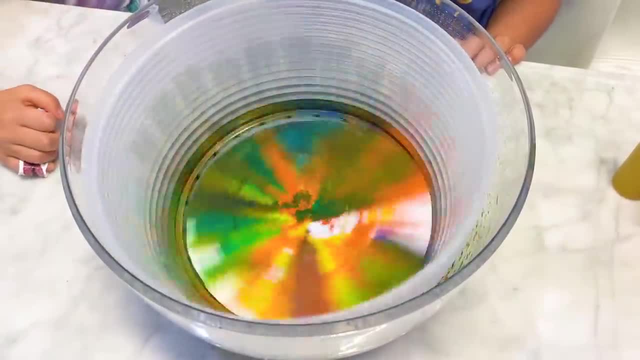 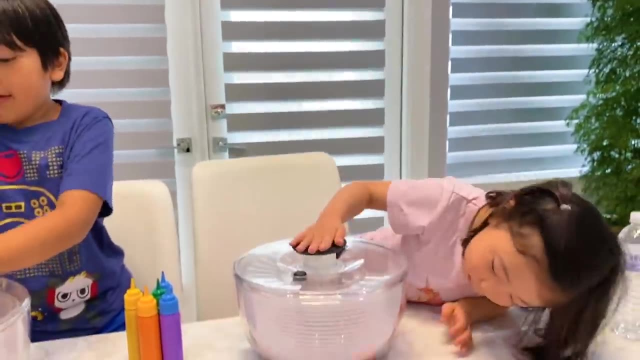 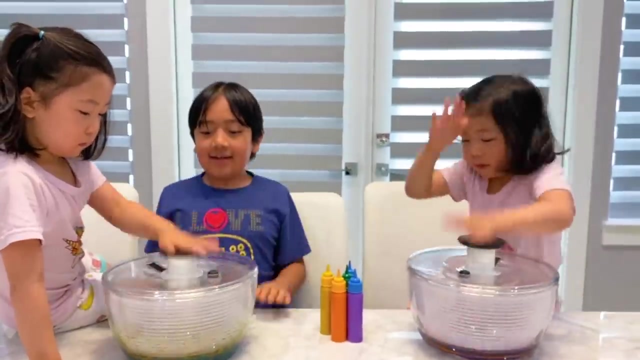 It's still spinning. It's like going crazy. Oh, it's dizzy. Whoa, Emma, you want to see yours? I don't see right here. Okay, Whoa, I think it's done. Let's see what Emma looks like. 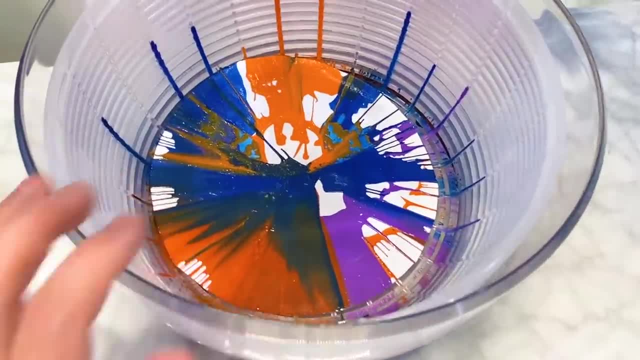 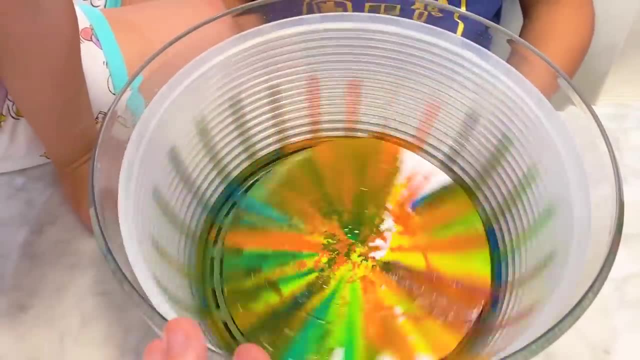 It's spinning. Whoa, it's like dizzy. I'll stop it for you. Whoa, it looks super cool. Let's see what Ryan looks like. Whoa, it's super dizzy. Be careful. Whoa, Yeah, it looks super cool guys. 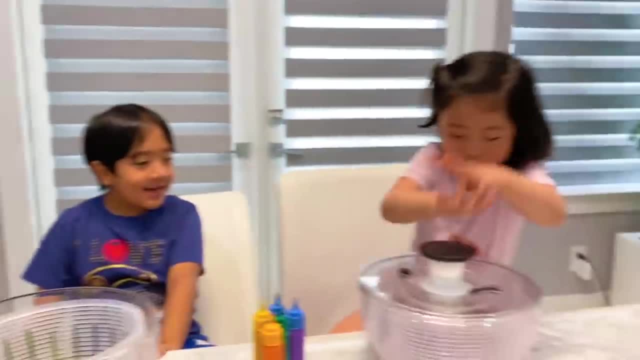 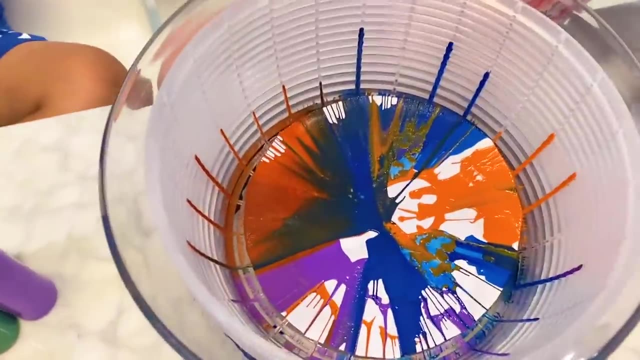 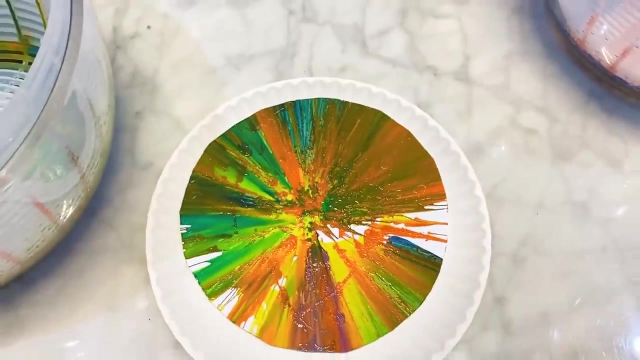 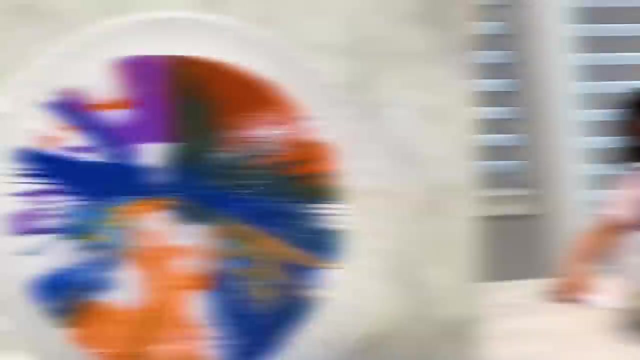 Good job. Of course, Emma's still going: Whoa, Yeah, Okay, when you're done, you just take out your beautiful painting. That's Ryan, That's right. And this is Kate And this is Emma's. So good guys, Perfect. 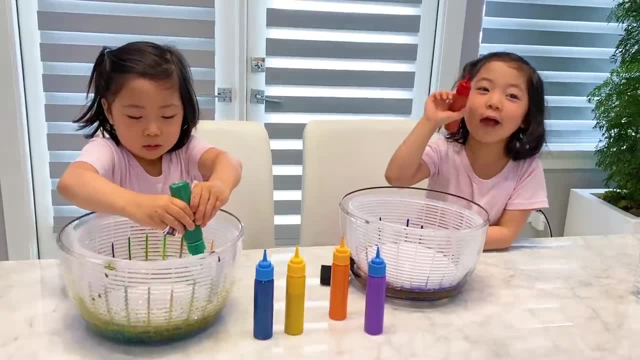 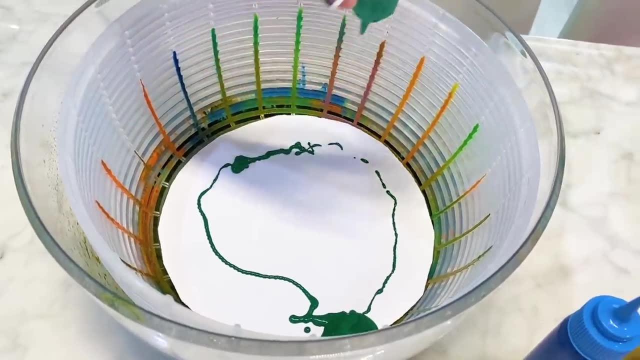 Okay, now Emma, Kate's going to try Put it in. I'm drawing a woman. Okay, anything you like, I'm going to show you guys a different technique. You can do anything you want. I'm drawing an animal. 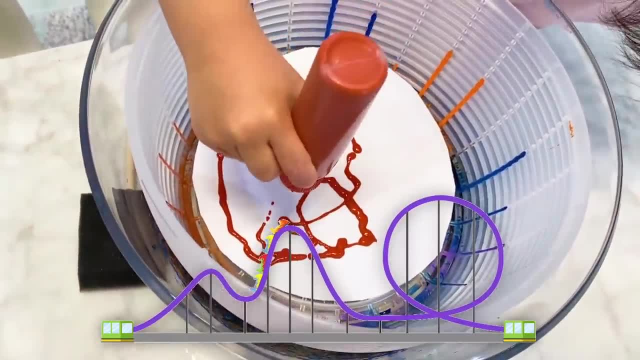 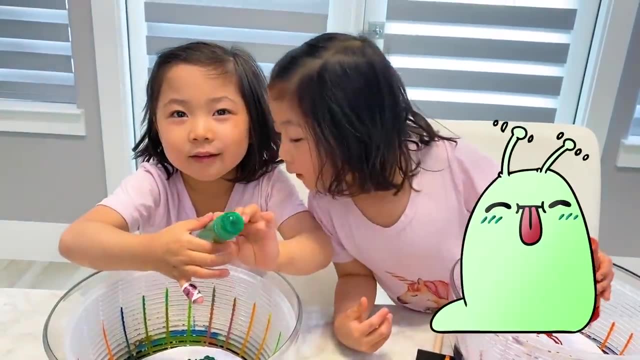 Can you guess what animal I'm drawing? A roller coaster, Oh, that looks so cool. Let's see what Kate's drawing. What animal do you guys think that is? Is that a slug? Yay, Oh, Emma, you're just going crazy. 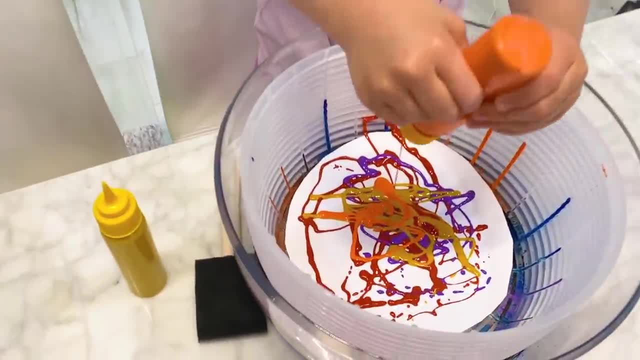 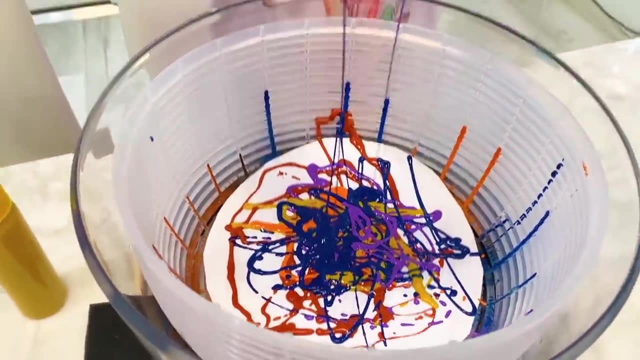 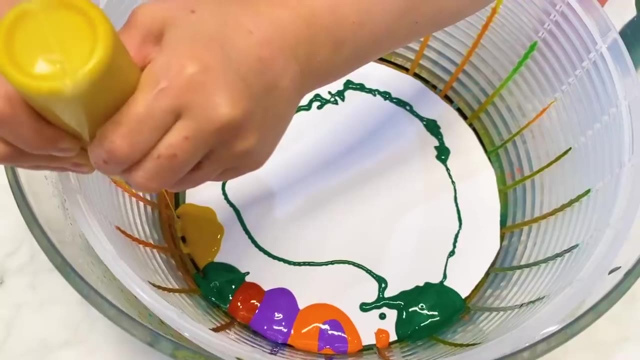 That's his food. Oh, the slug's food. Yeah, Whoa, Emma, I love it. Guys, look at this purple, I love that slime, I love that. Wow, Cool art. Look, Love it, I need some. 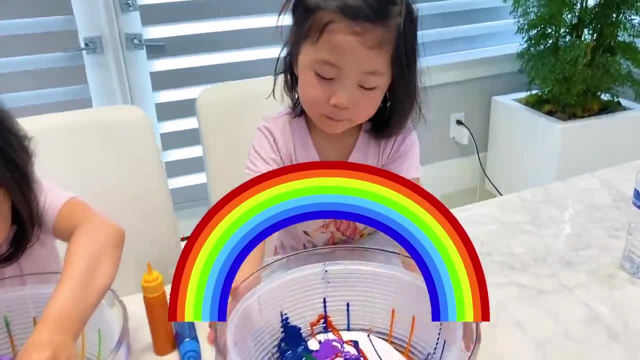 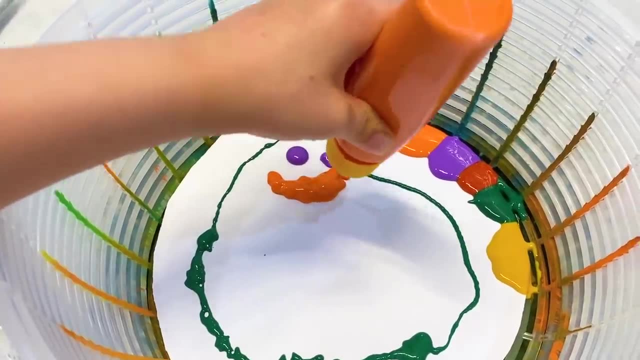 It's a lot, Emma, but it's going to be great. It's a rainbow. Oh, I see, I see a rainbow. I see the slug. Yeah, I see it. Oh, whoa, Kate, you guys see the slug there. 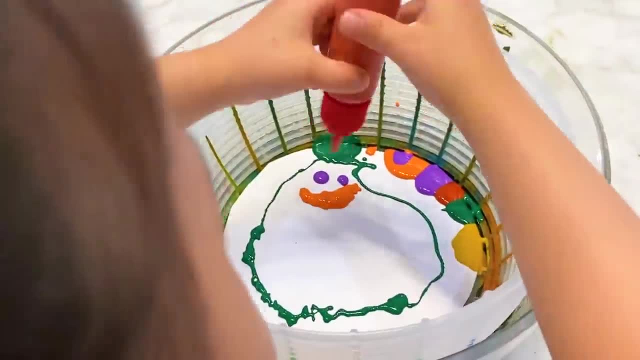 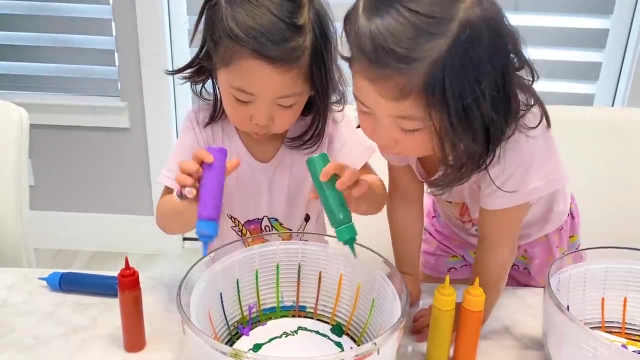 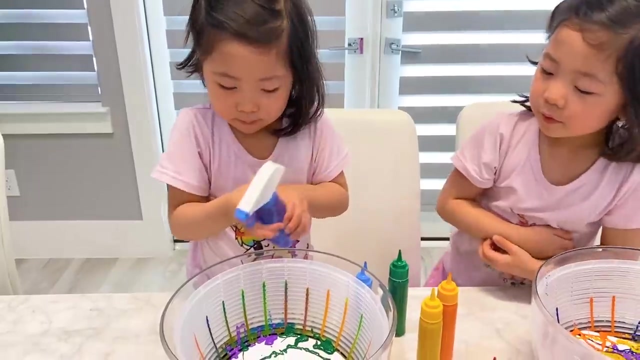 So cute, I love the mouth. Okay, now some red. Okay, what's the red for The nose? And a round one. this time Got it. So you're done, Done, Okay. Okay, we're going to try something different. 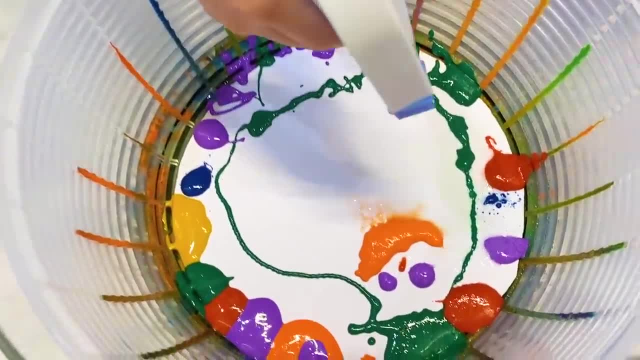 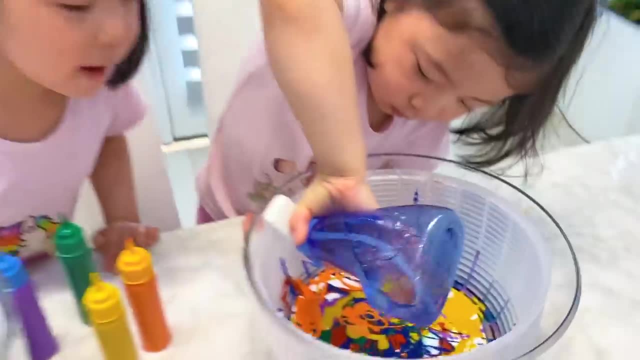 We're going to try to spray with water first to see what happens. Spray, spray away. It's just water. You guys see how it's wet a little bit. It's going to be great when you spin it. Whoa, there we go. 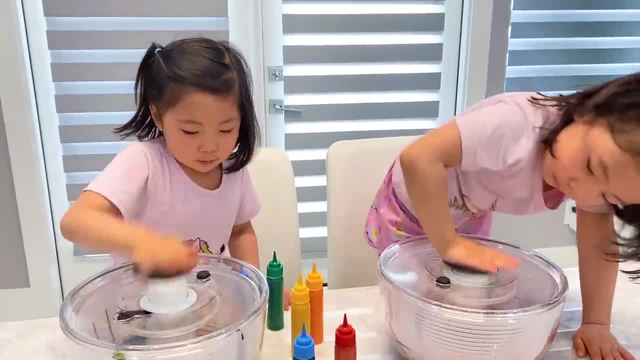 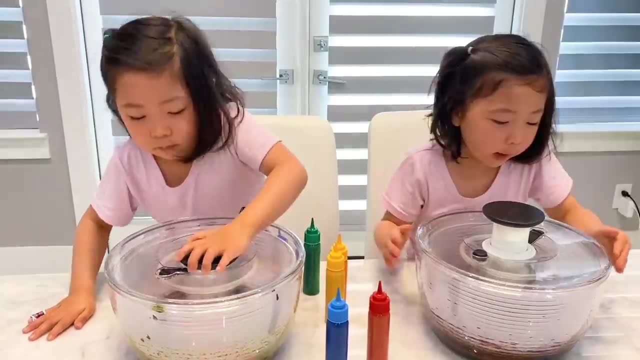 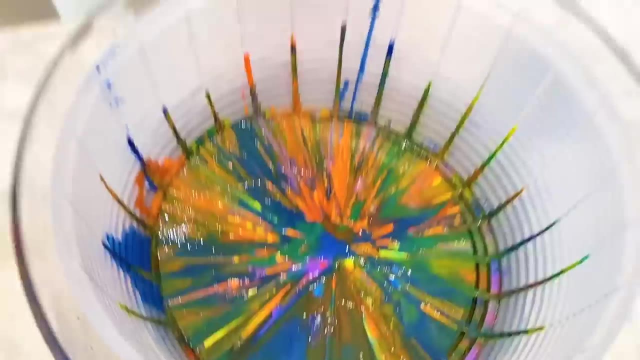 I'm going to try to spray. Looking great guys, Looking great Emma. Aw, that's sweet. Look at that one. Ready, You ready? Ready for mouth Ready? let's see what this is like. Whoa, that looks super cool, Emma. 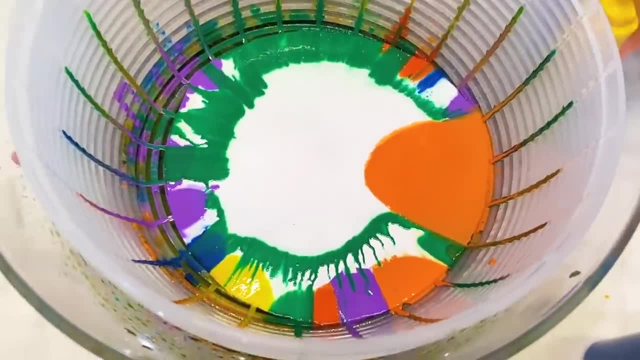 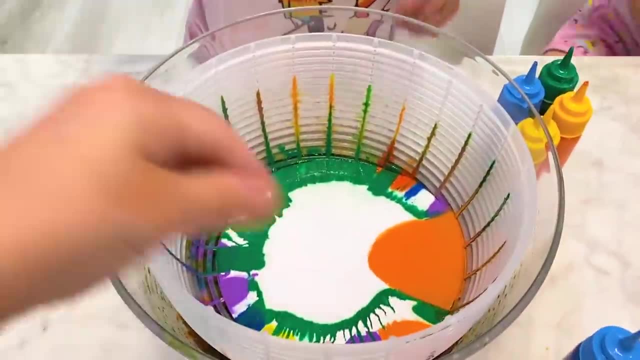 Whoa, that's so cool. You like mine too. All the colors spread on the outside. I like mine. Yours looks super cool. Here's what we're going to do, So we're going to use this and just spread it around. 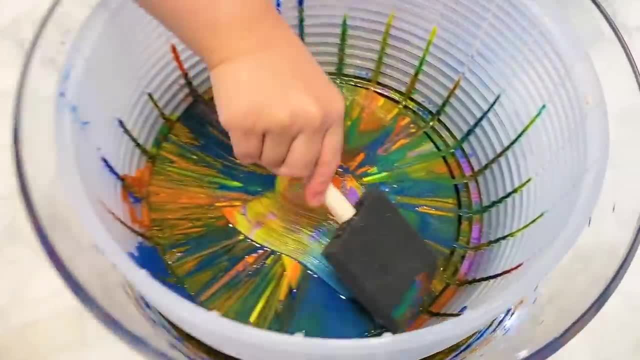 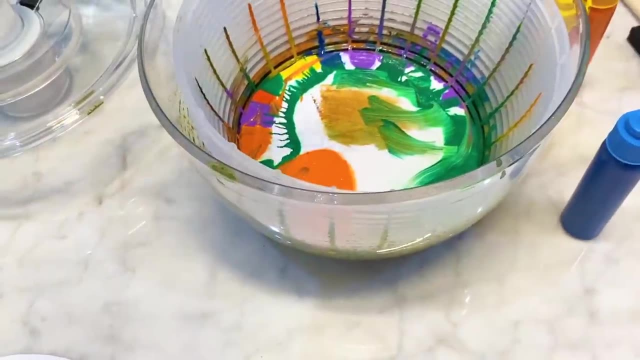 We're going to try to just spread all the colors around. Oh, it's turning colors, Yeah, like that. There you go. Maybe you want to add some more. Kate, You want to add some more colors? Let's see Here we still have some red. 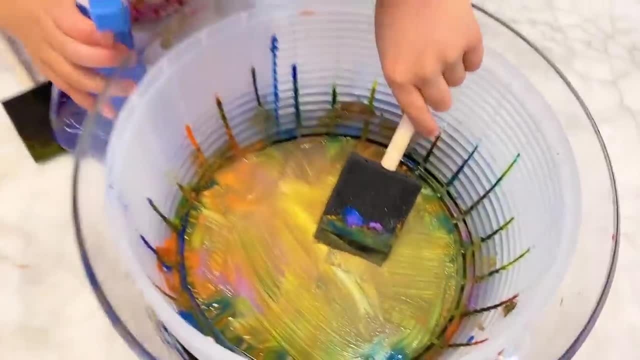 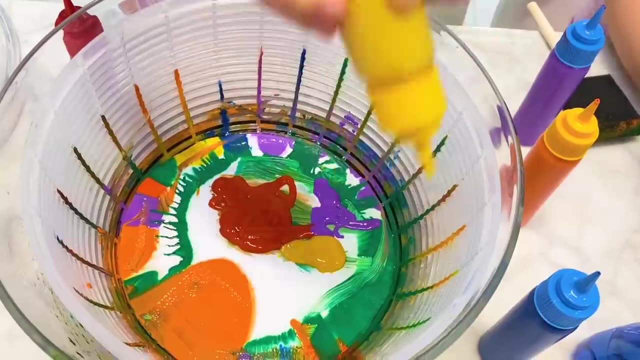 There you go, Just spray all around. Yeah, it looks great. You can add more color, Emma, if you want. Whatever you want to do, It's art. You cannot go wrong with art. Great Kate's going to add a little more water. 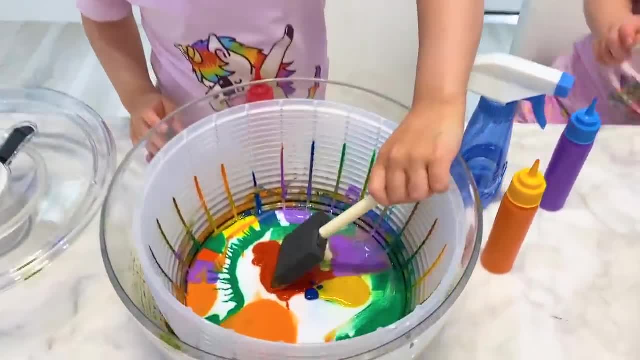 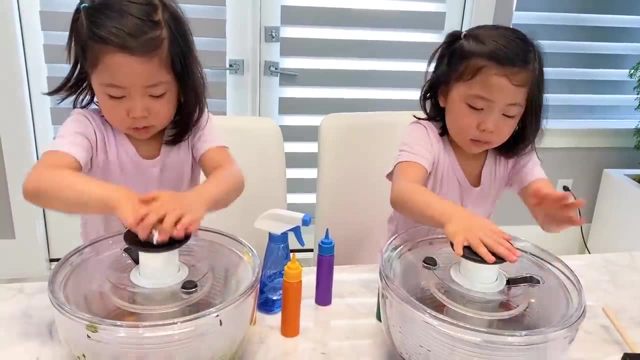 Then you want to spread some. You can do that too, if you like. Anything you want. We did a lot of water. Yours looks cool too, Emma. I'm going to bring the spinner back and spin away. See if there's any difference. 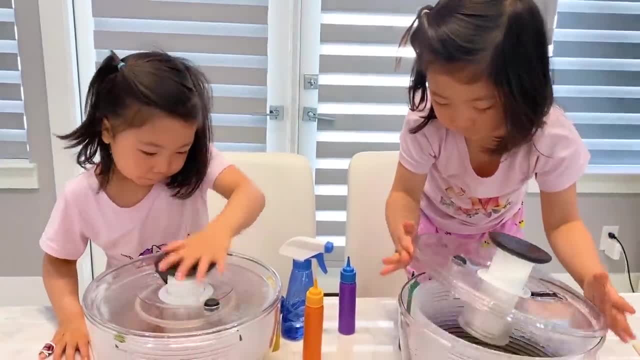 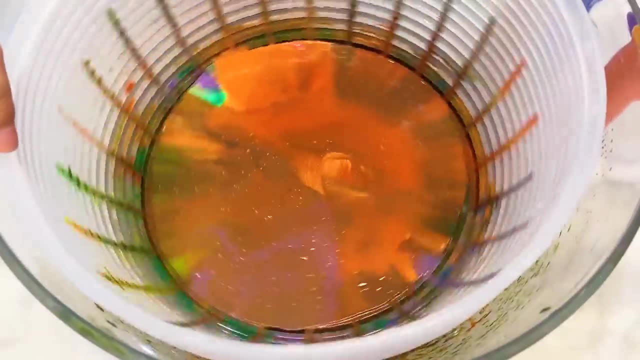 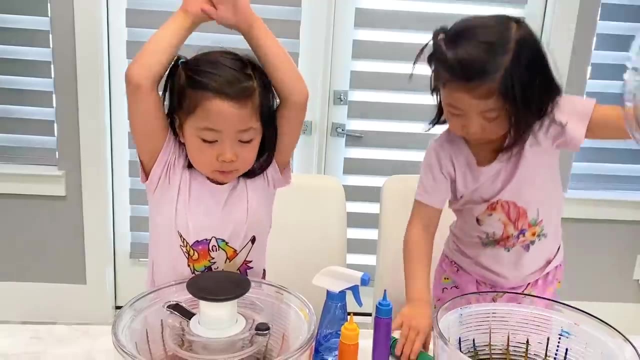 Are you going to see the colors? Yeah, Whoa, That's so cool, Love it, That's so cool. It looks like a marble sort of art. Very cool guys. You guys just like to spin. Good job, Emma. 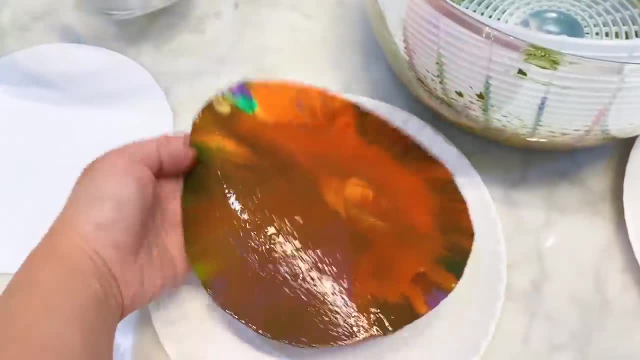 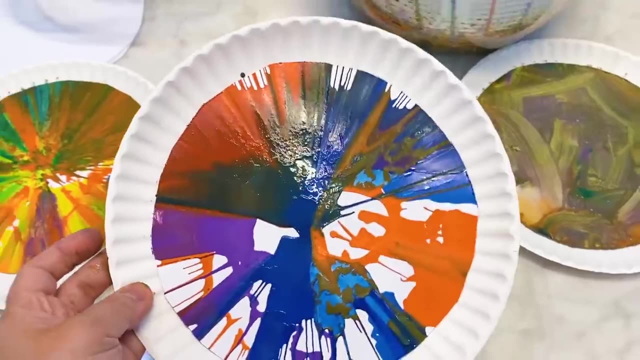 Great. Okay, when you're done, you just take out your art piece again. It looks really cool, Emma looks cool too. There it is. Take it out. So there it is. Then you just wait for it to dry. You're going to have beautiful, beautiful artwork. 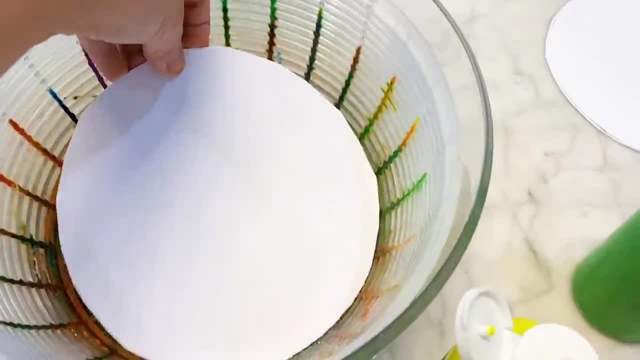 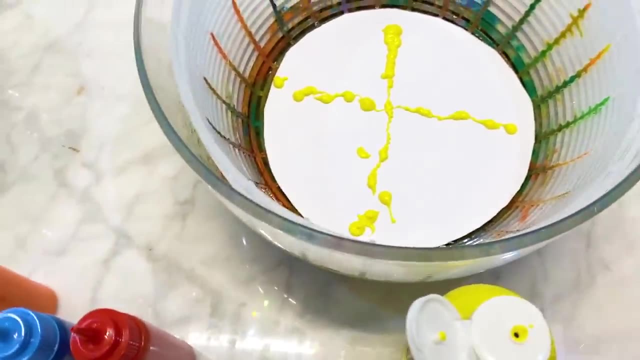 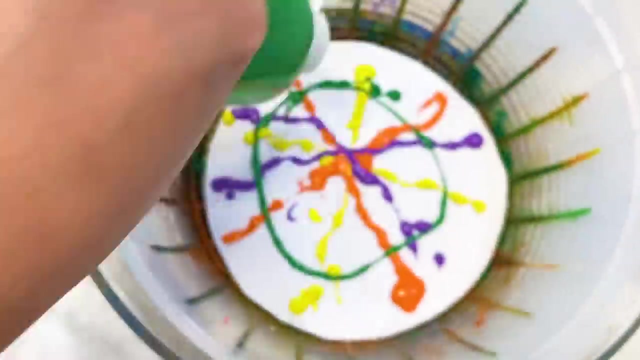 Hi, Okay, it looks so much fun. I think I want to try one too. What if I just do a star? I'm not very good at this, guys. Whoa, That's kind of cool. One more color. I think I'm just going to go circle all around. 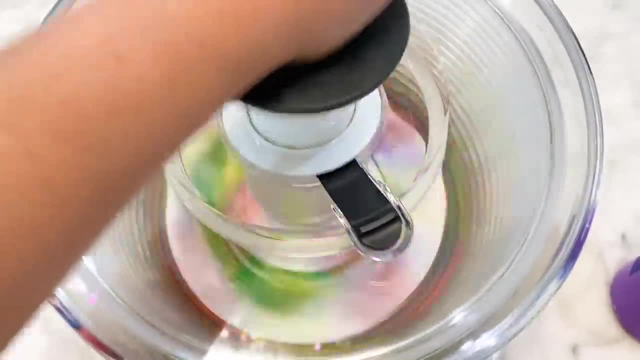 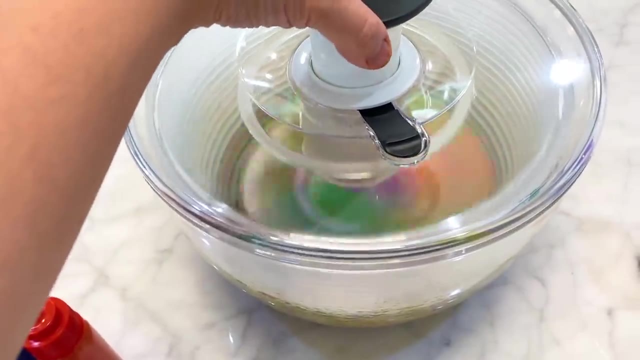 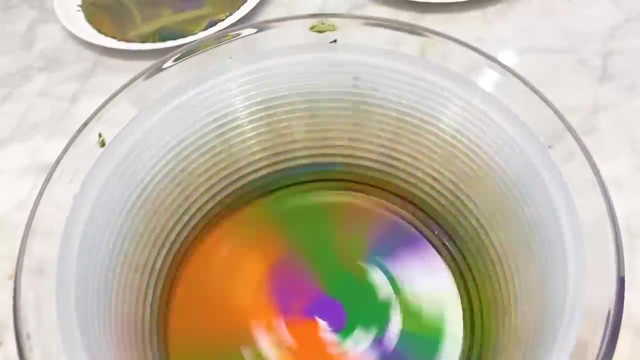 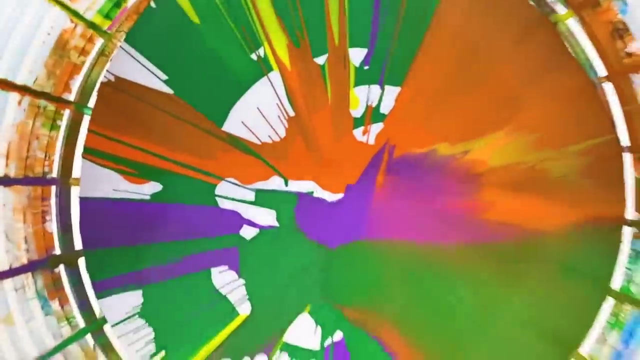 Spinning time. Whee, Let's see if it makes any difference. It looks super cool when it spins Any day now, Any day now. Whoa, Look at that. What do you guys think? Ooh, Thank you so much for watching. 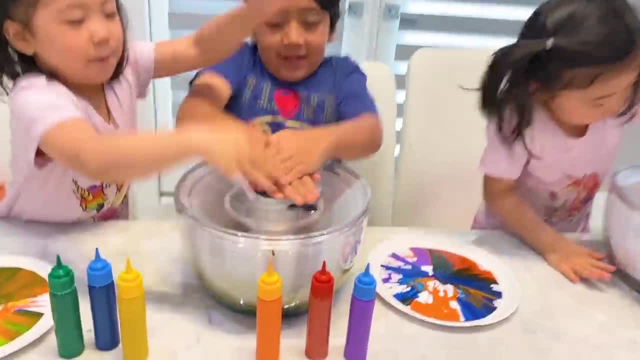 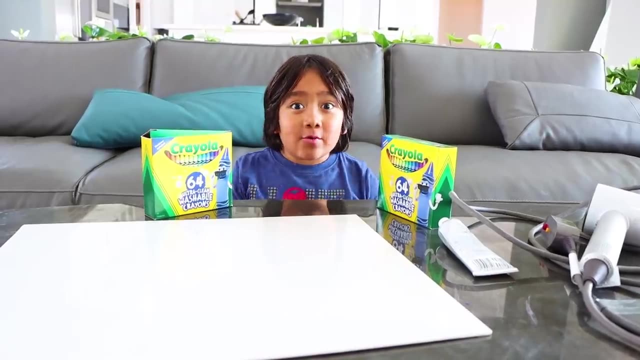 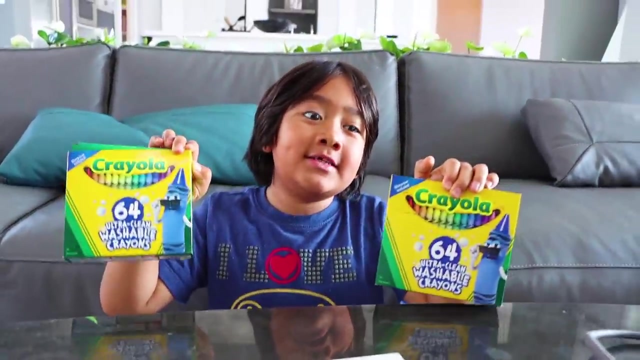 We're going to do more now. Bye, Put nothing inside, Bye. Hey guys, Today we're going to be melting crayons to make art. So first, obviously, you need some crayons And also you need something to put all the melted crayons on. 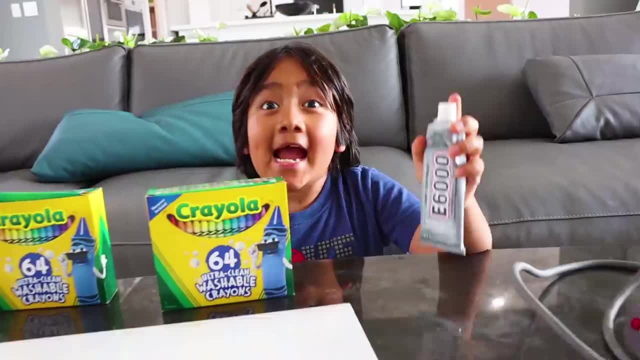 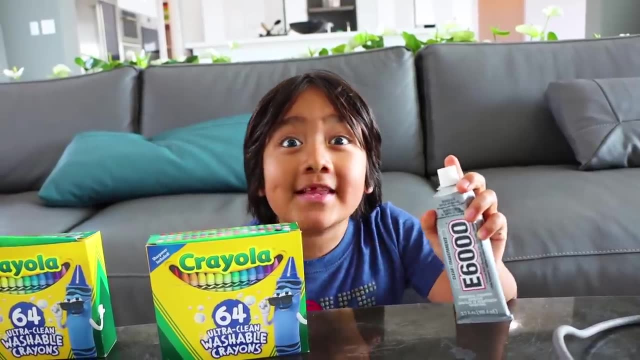 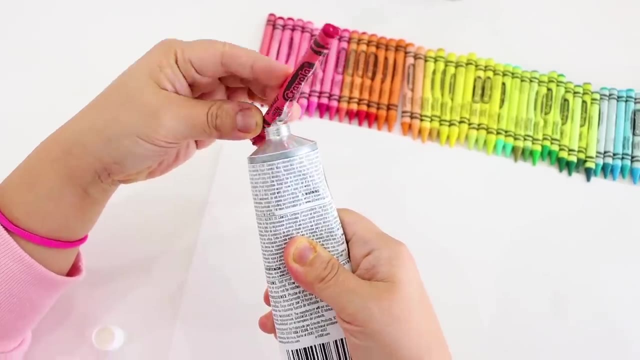 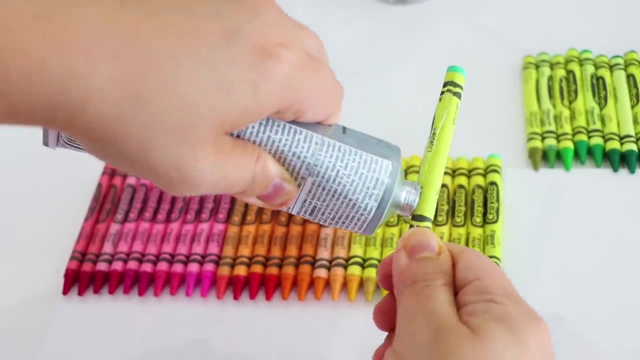 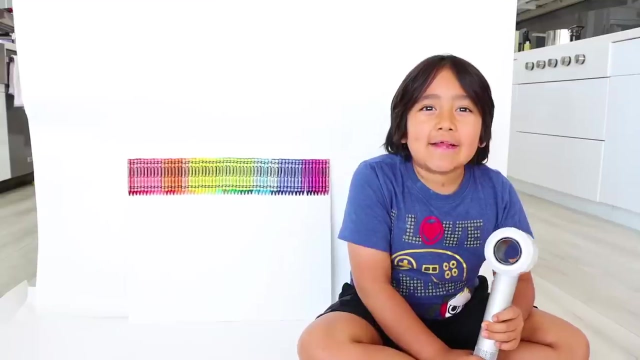 And a hair dryer And some glue. You can use hot glue or super glue, but make sure your parents use it. Okay, let's get started Now. let's melt the crayons with a blow dryer, But remember to protect your house. 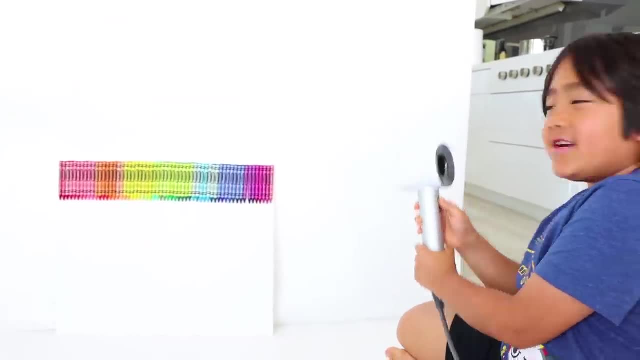 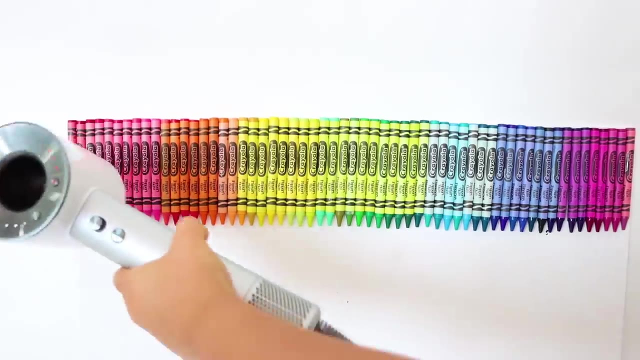 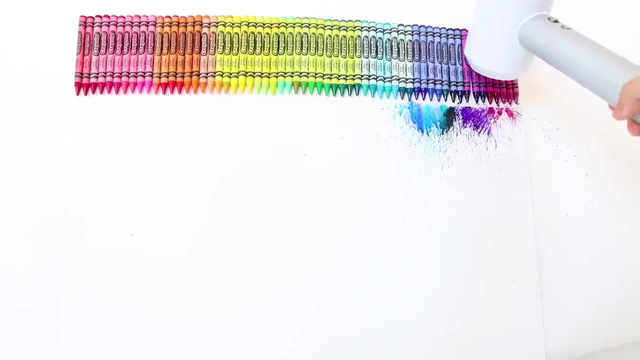 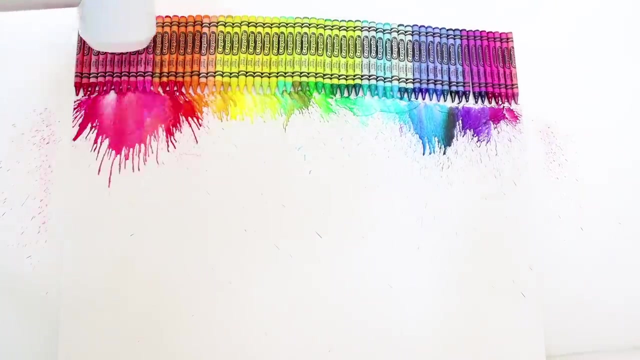 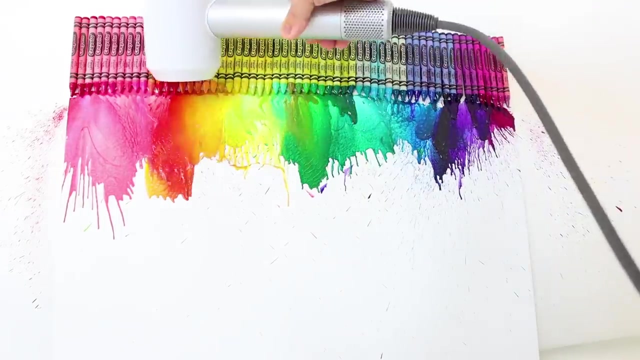 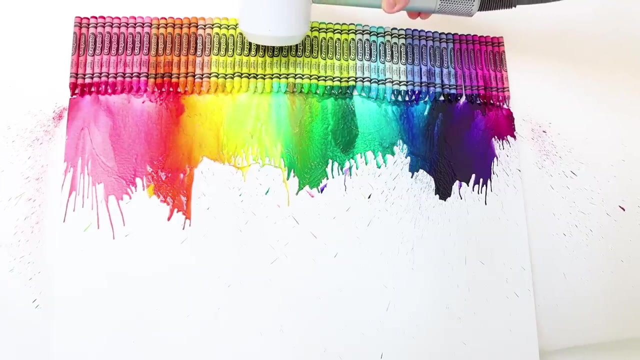 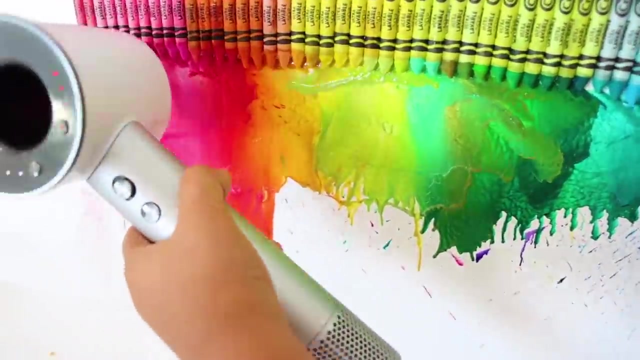 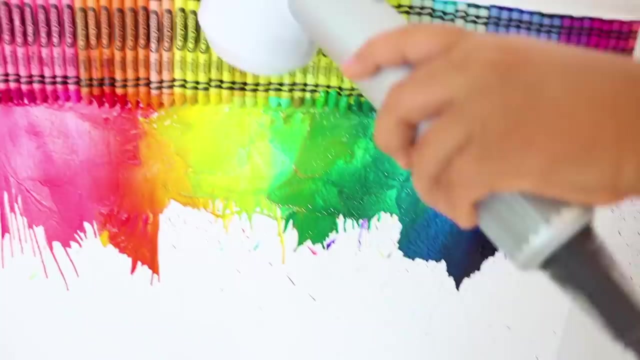 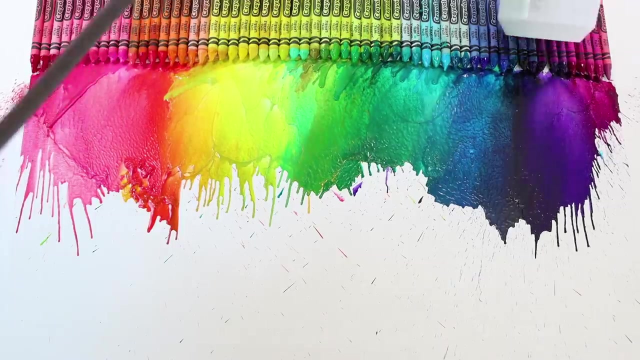 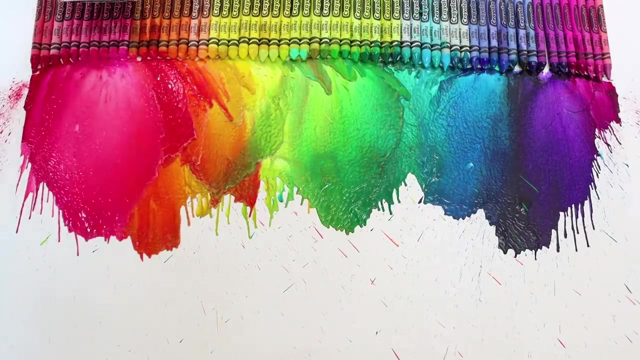 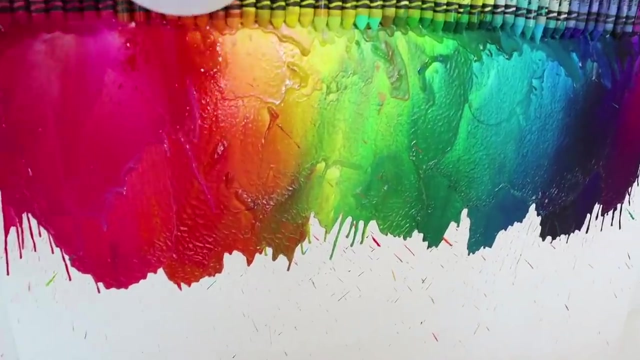 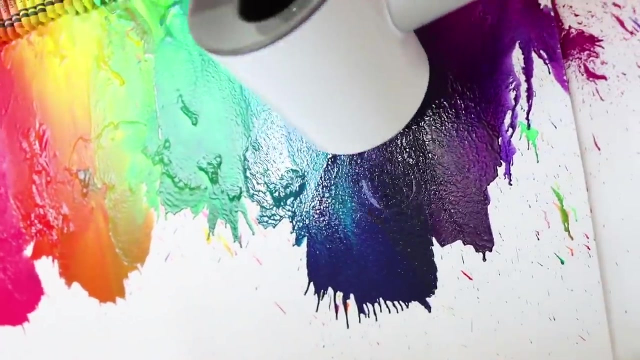 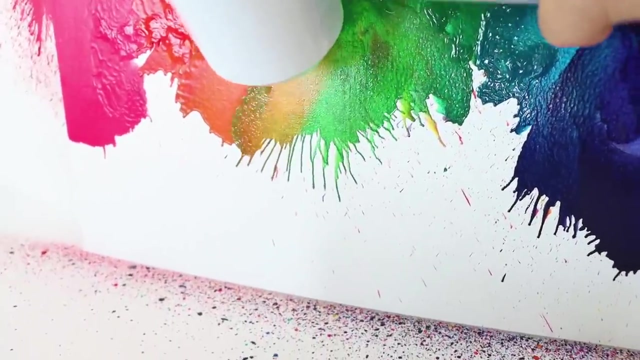 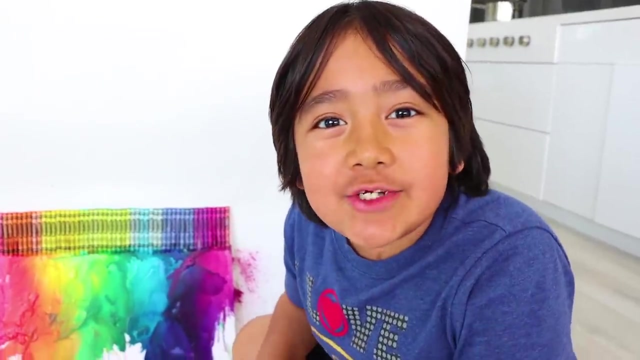 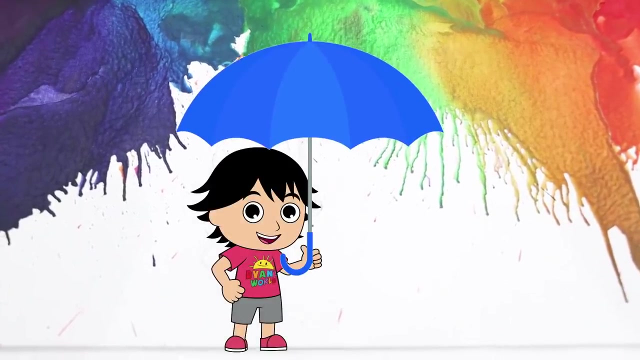 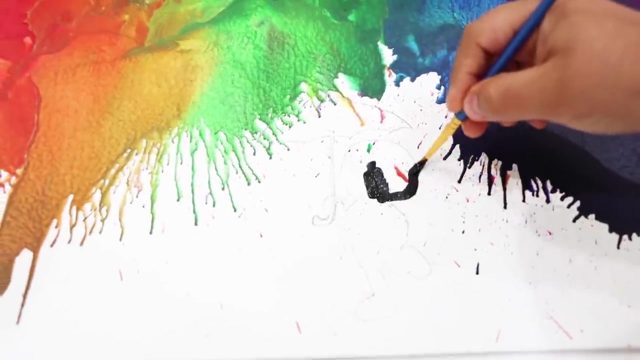 with some kind of paper. Three, two, one go. 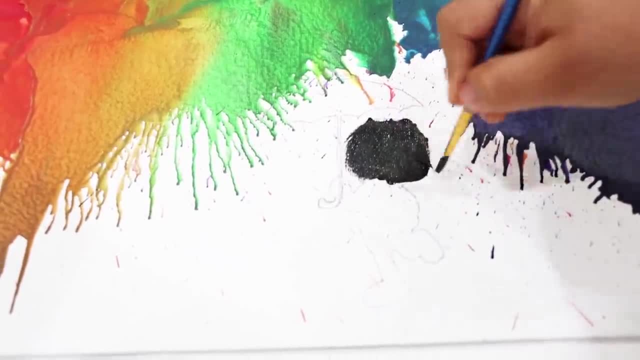 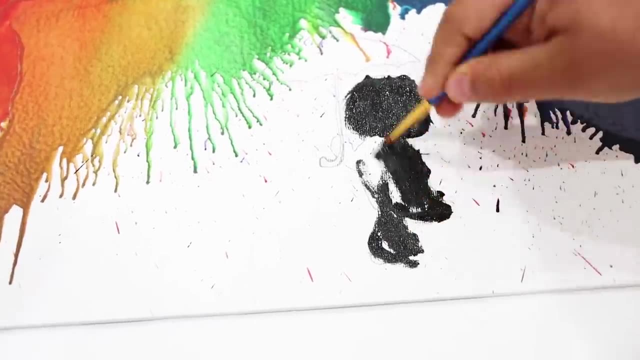 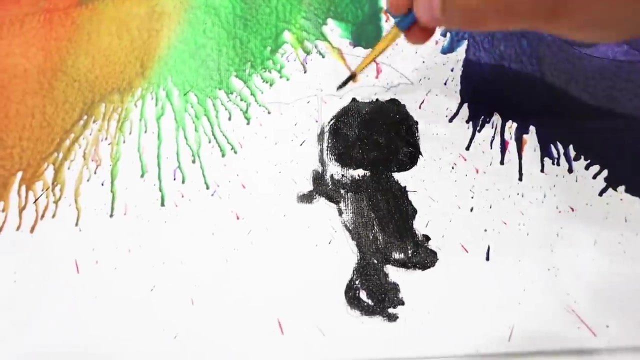 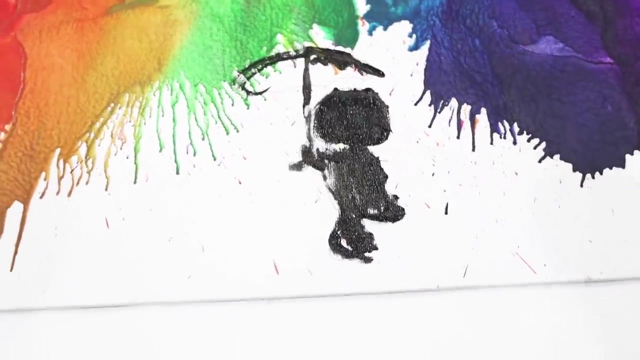 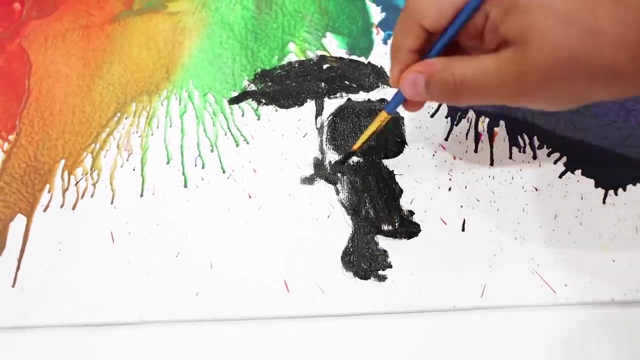 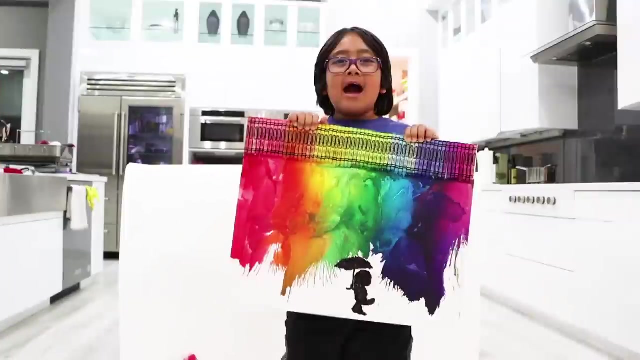 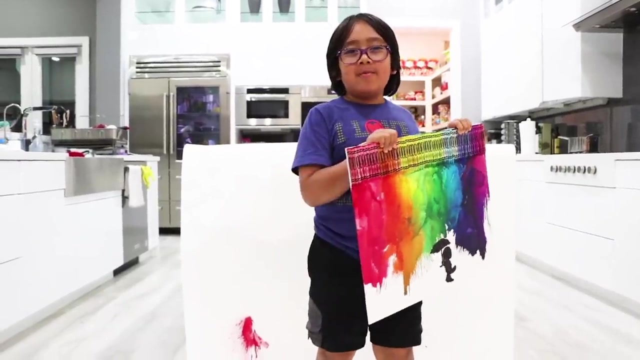 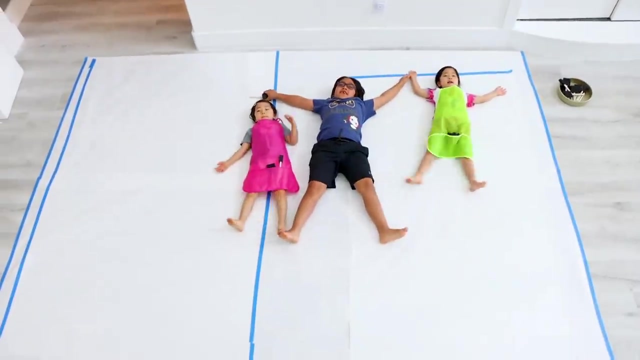 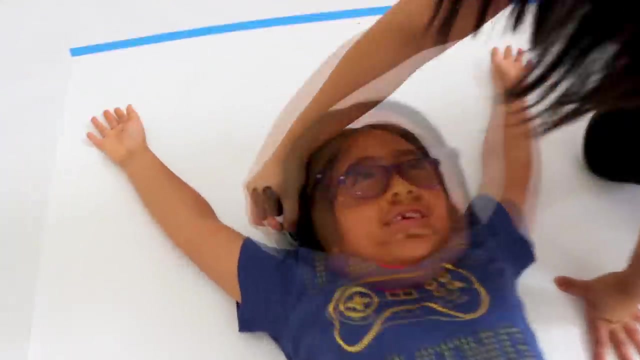 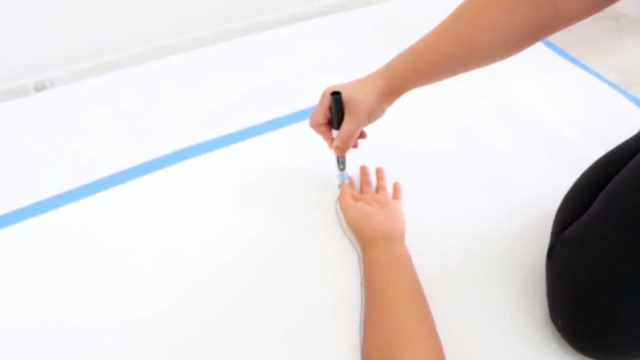 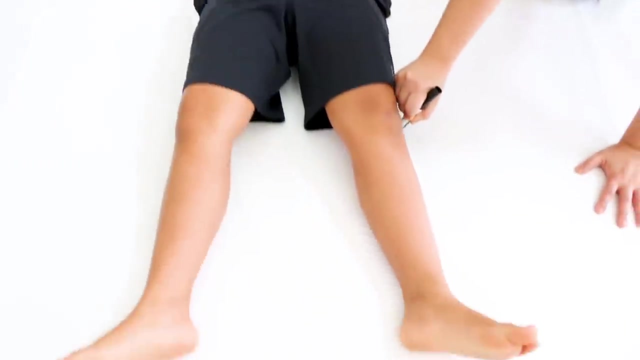 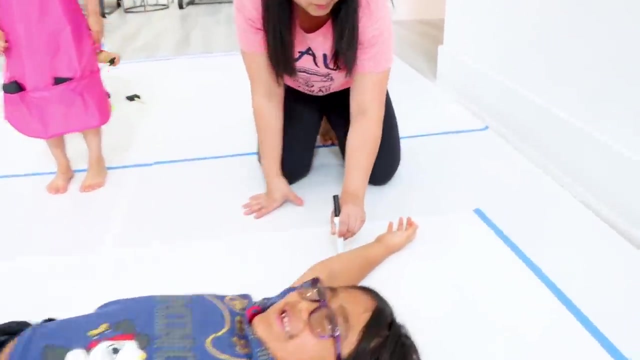 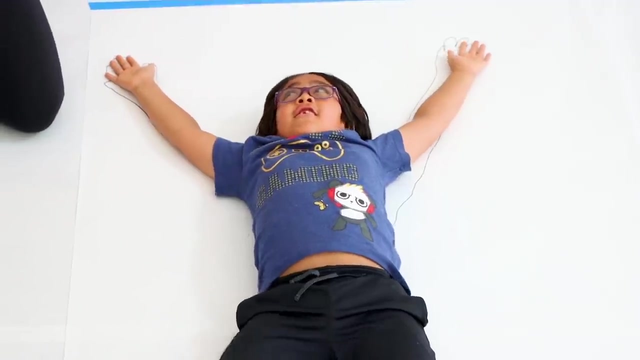 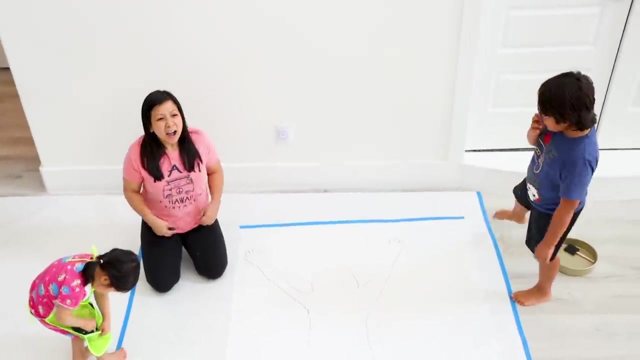 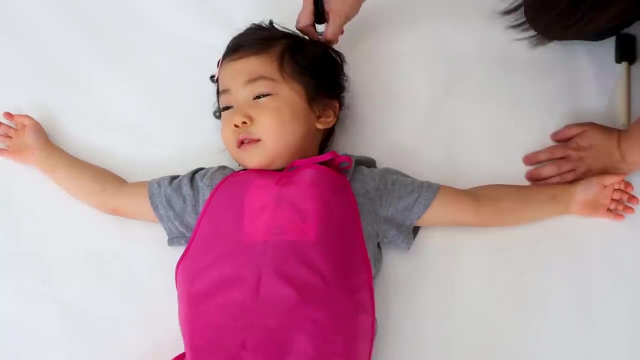 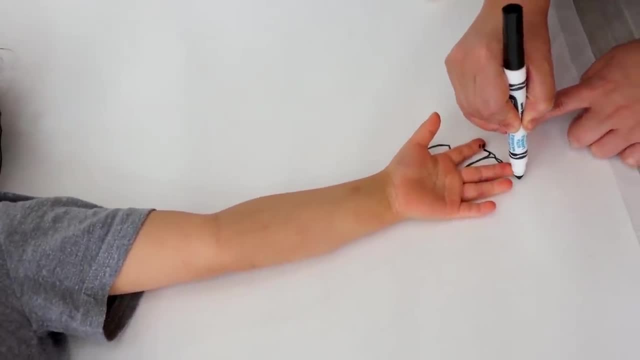 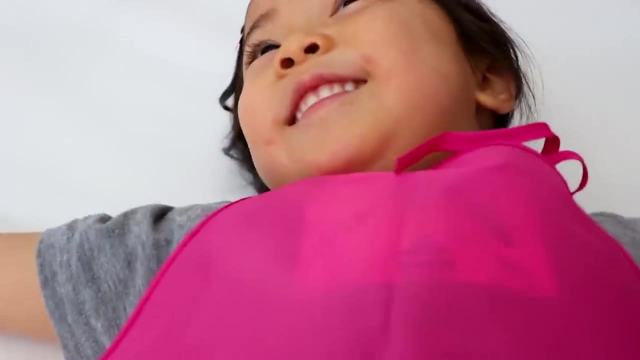 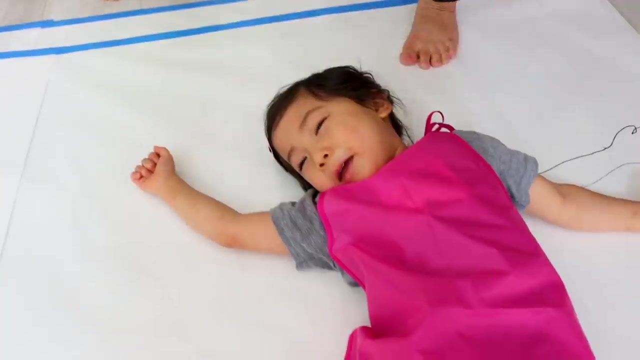 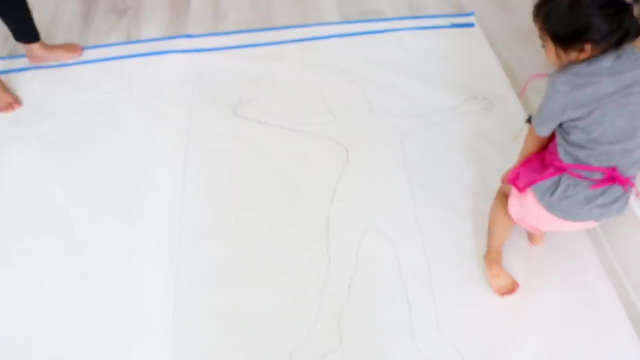 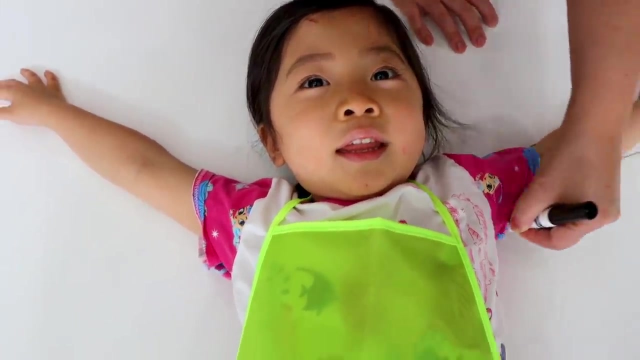 Wow, Emma, you ready? Yeah, It's Emma's turn, And Emma's just staring at somewhere. Hi, Emma, I'm going down, Woohoo, And Ryan's also tickling too, so it's double tickling. 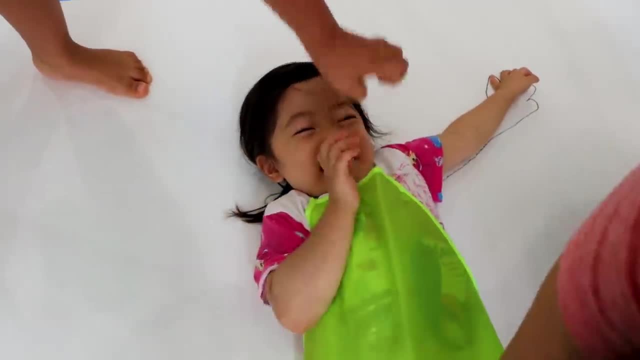 All right, Emma's done. Yay, Let me see, let me see, let me see. Oh, whoa, Yours is probably the best, and very slim. Okay, now that we traced our outlines, it's time to paint. 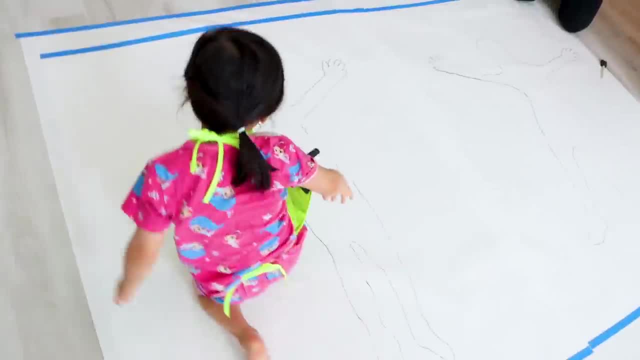 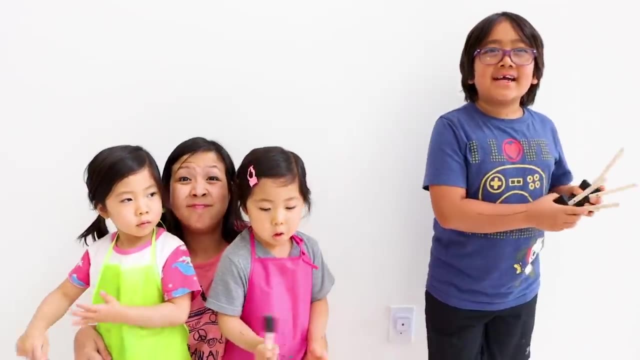 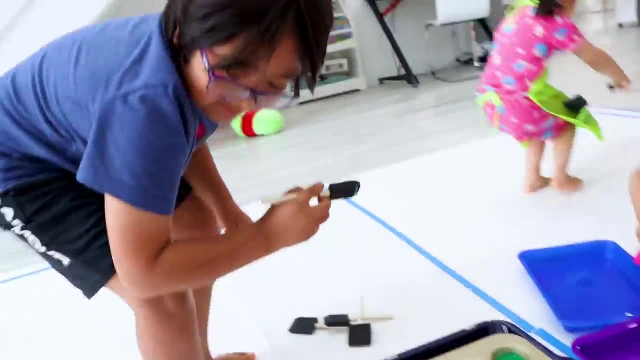 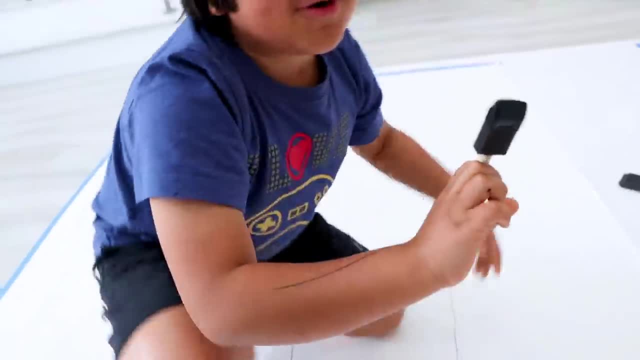 Anywhere you want, Anywhere you want. I'm trying to Okay, you want the body, You want a picture. I'm trying to draw, like the neck part thingy, The neck part Shirts, Like no, like this part. 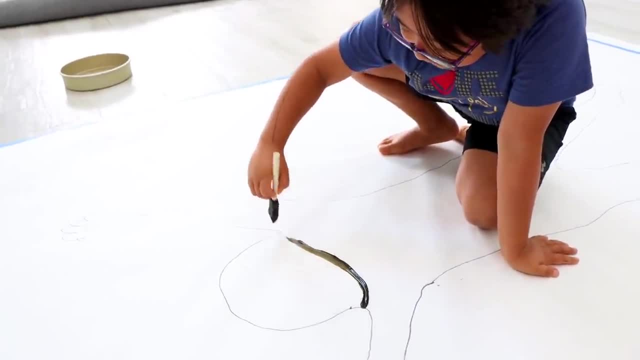 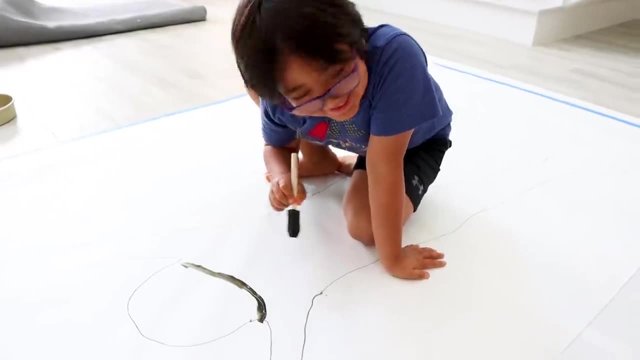 Oh, okay, Yeah, yeah sure. Uh, what, Uh huh? Oh okay, Giant smiley face. What do we? Okay, so Kate is starting from her feet right. Finish, Emma, it's okay. 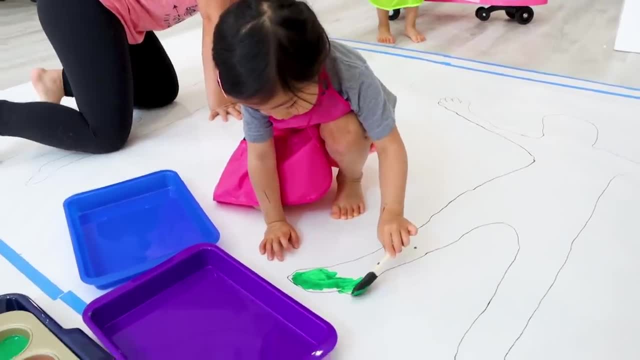 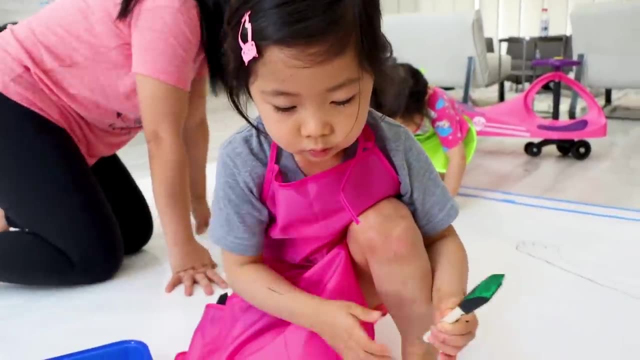 Do you have a camera? Yeah, Yeah, Yeah Yeah. Do you have like a green shoes or something? Okay, Nice, And Kate's really good at art. Once she's focused, she can't even hear me, Right, Kate? 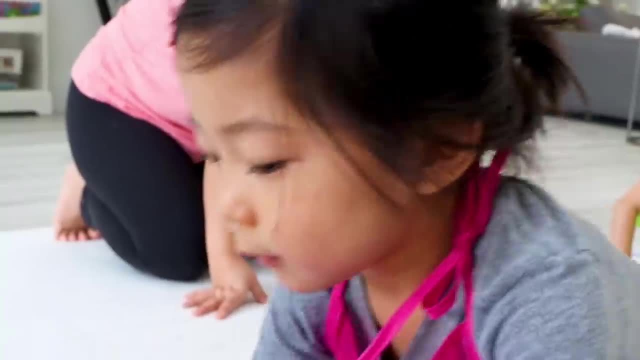 Right, Kate, I think she heard that one. I think she heard that. Good job, Kate. Like a green foot, All right, mommy's going around everybody and just helping each one of them. Okay, yeah, Anybody need help, let me know okay. 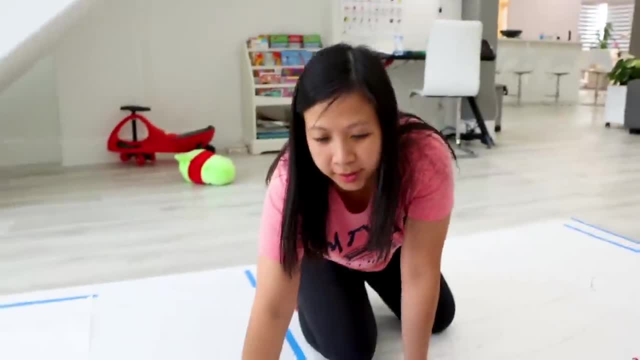 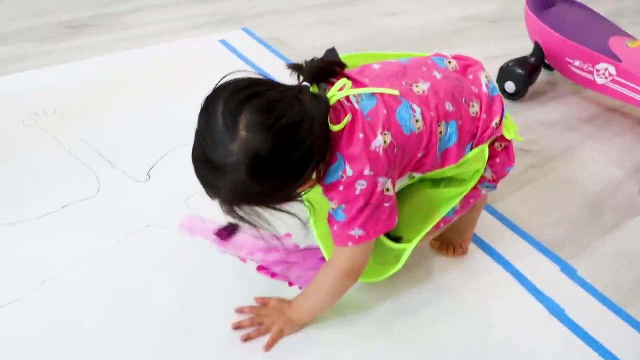 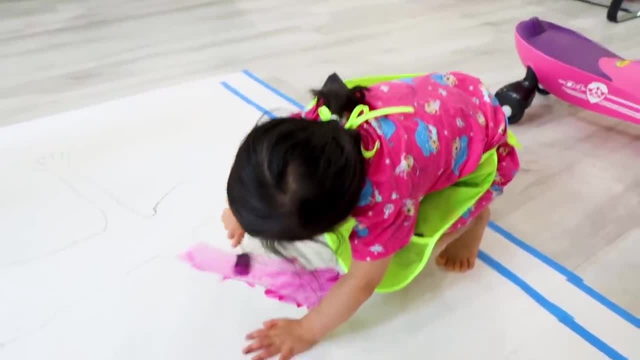 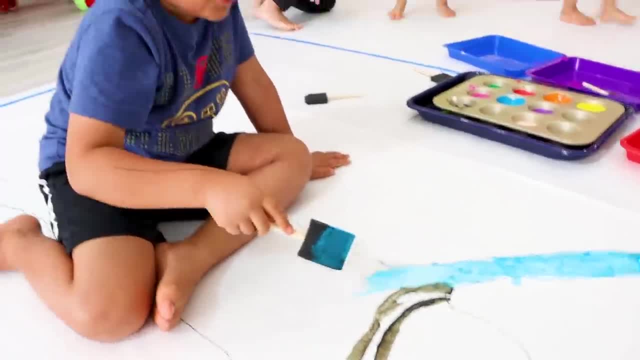 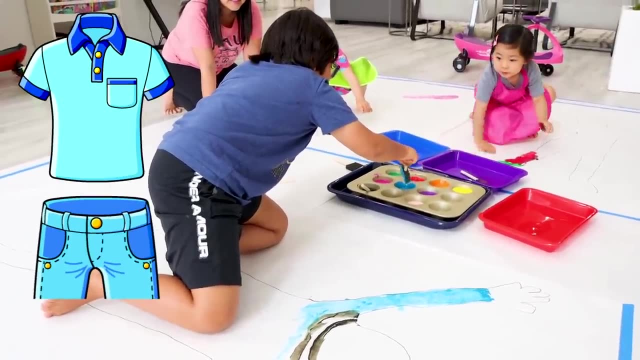 I like it. It's a long shirt And I do not like long shirts, so I don't know why I put a long shirt. That's right. If you guys noticed, Ryan always loves to wear a t-shirt and shorts, Nothing else. 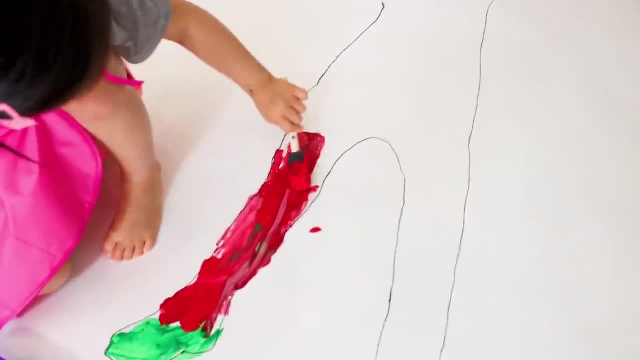 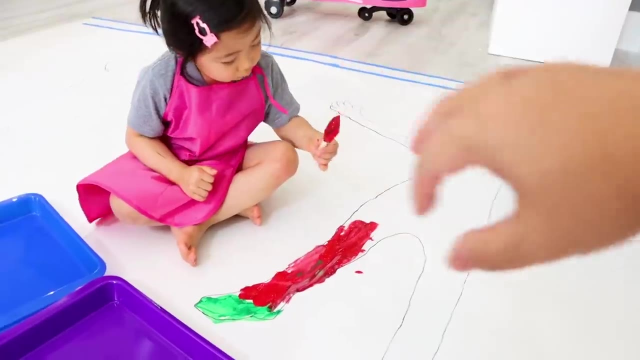 Even in the wintertime, Ryan still wears a t-shirt. Oh wow, Okay, Good job. Red pants- Nice, I like it. Okay, Good job, You were painting within the line. Good job, Emma is She's more dynamic? 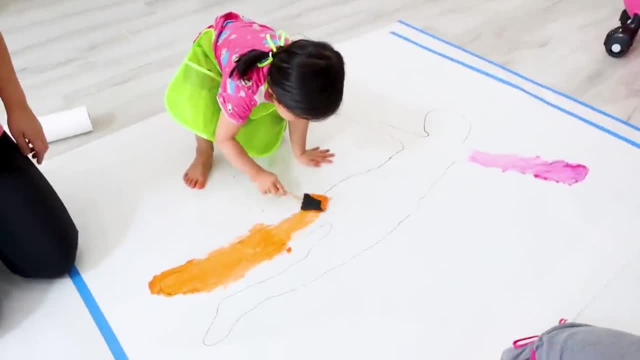 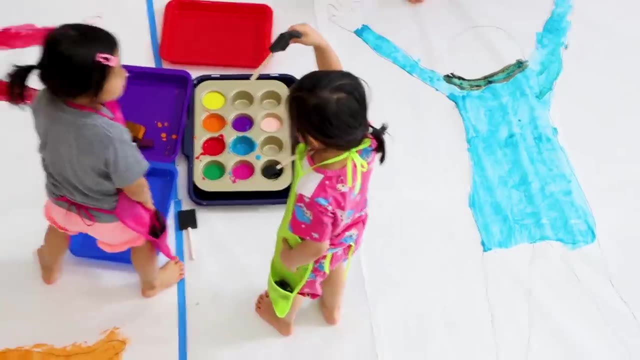 Yeah Right, She's all about big scale. Good job, Emma, She's doing great, And Ryan too. What do you want me to do, Ryan? You draw fast. Look at that. I don't know if you guys noticed, but they all selected different colors for their body. 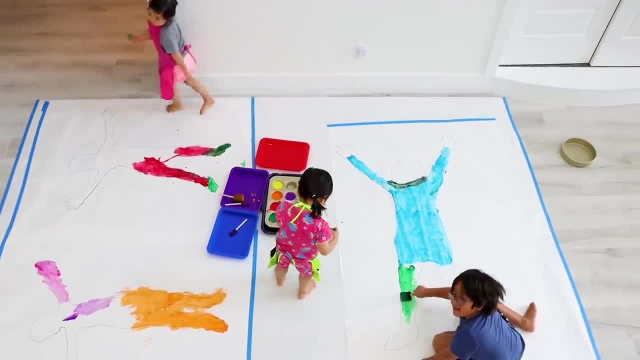 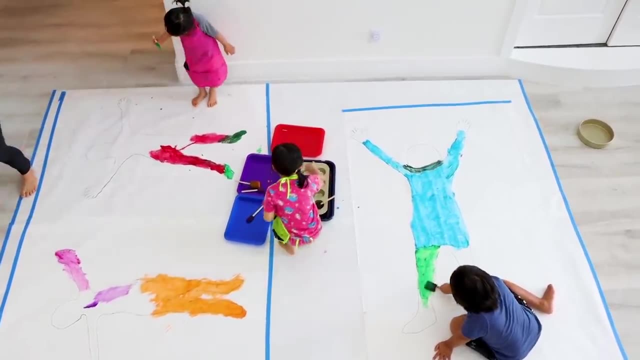 part. How's it going, guys? Good Good, Where's Daddy Up there. Up there, Hi Emma, How are you? You're so far. You know, Ryan, yours kind of look like a Astronaut. 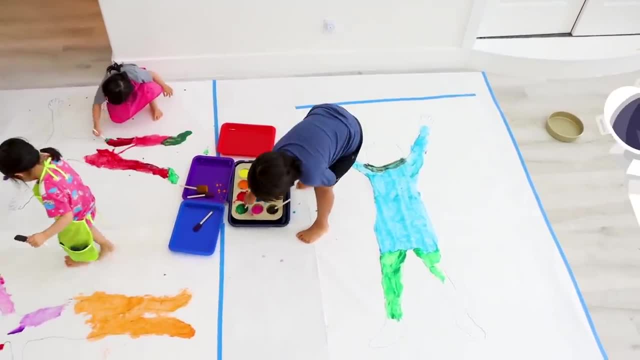 Astronaut. Yeah, It's like a helmet: Your head, Mommy. I made long pants and I made a t-shirt, T-shirt. Oh yeah, I made a long t-shirt. Good job, I've drawn all of them. 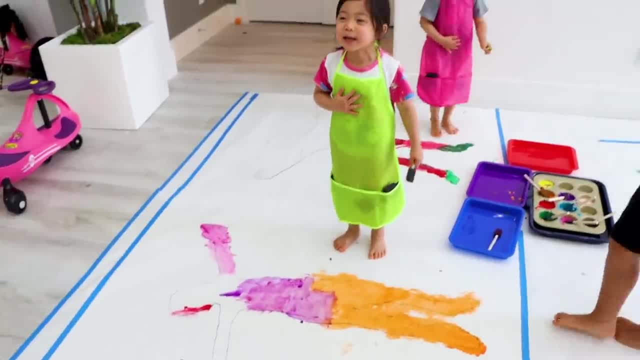 Oh see, You're done with the pants. Oh wow, I'm making art masterpiece right here. So Ryan is working on the most important part: face. Is it going to be a hat? No, No, No, No. 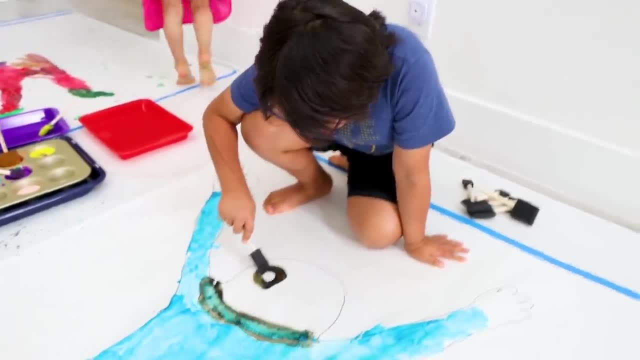 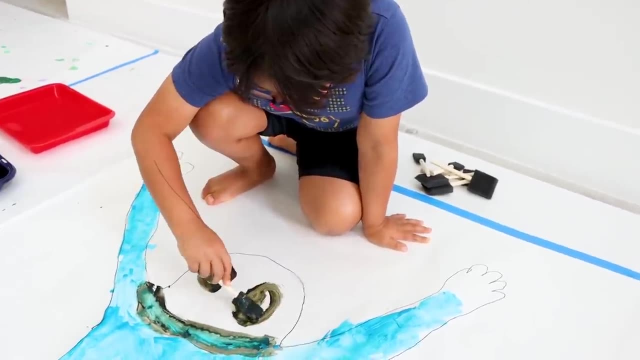 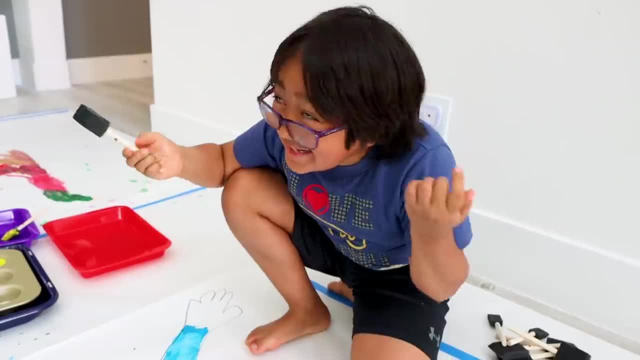 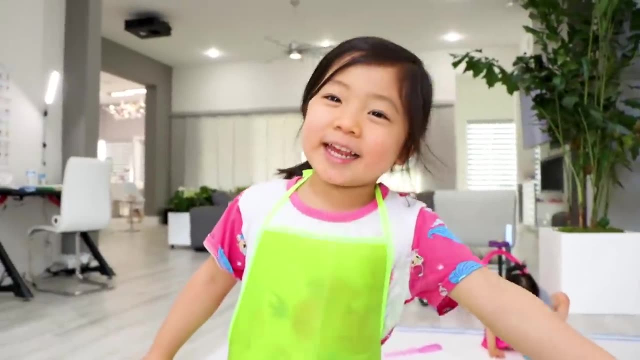 Aha, What, what do you mean? What are you talking about? Alien- Whoa, that's a big eye Daddy, Daddy, daddy, That like alien. Yeah, Ios The alien on my face. He does look like a alien a little bit. 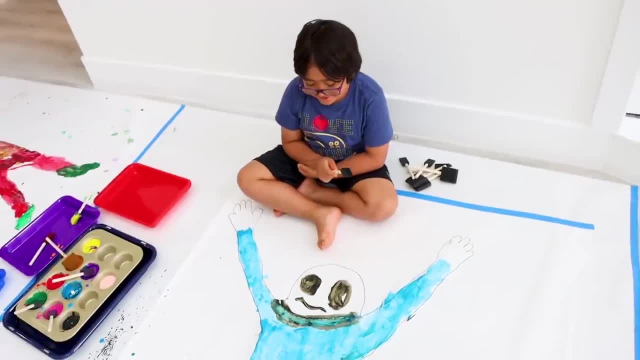 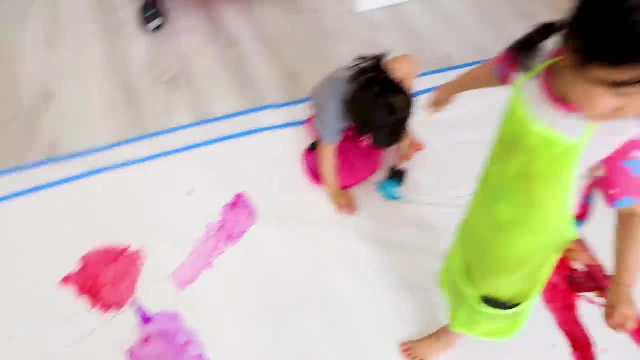 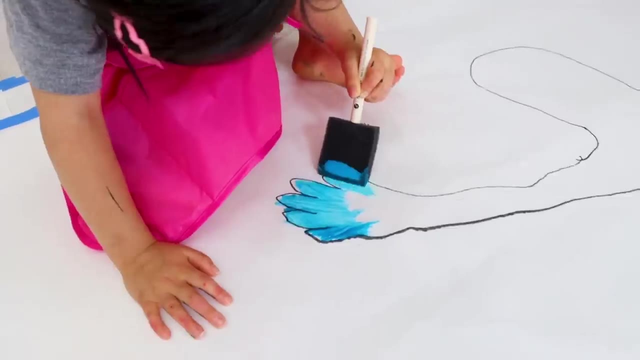 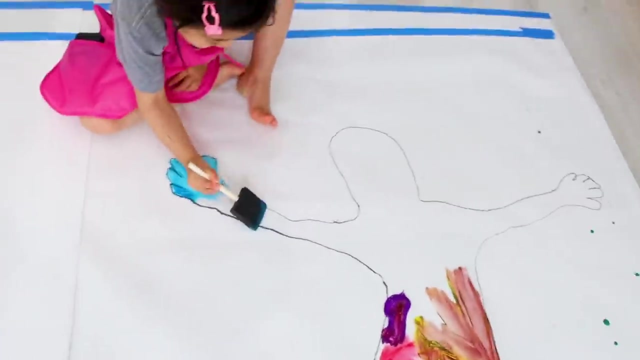 Yes, And big eyes, Oh, that's cute. What about yours? Your face is red. It is Interesting Kate's so attention to detail. look at that. Even though Emma and Kate are twins, the way they draw is completely different. look at that. This is Emma's and this is Kate. 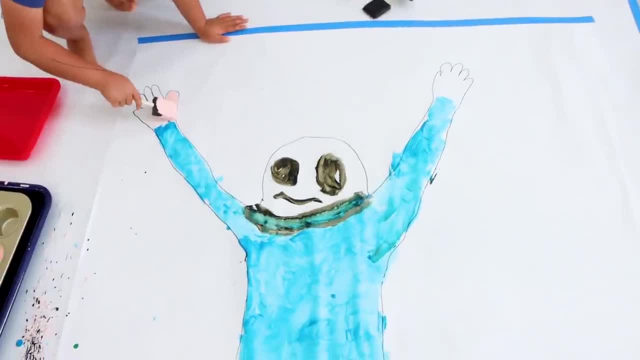 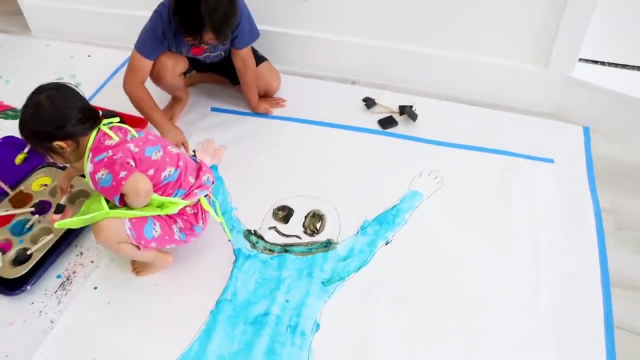 Can you guys tell the difference? You know, he kind of looks like that. that that youtuber, Ryan, Look like a marshmallow. You know who I'm talking about? that the head is marshmallow, DJ marshmallow- No, you don't know. you have a full-on skin over him. 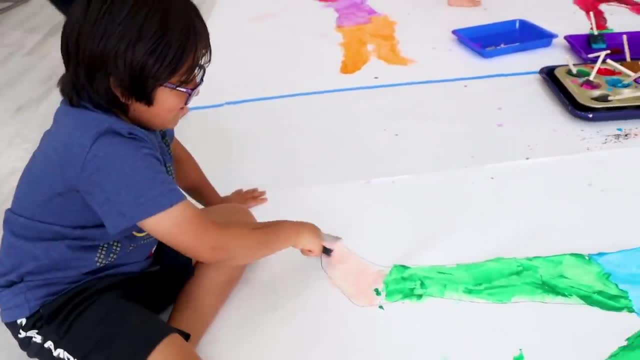 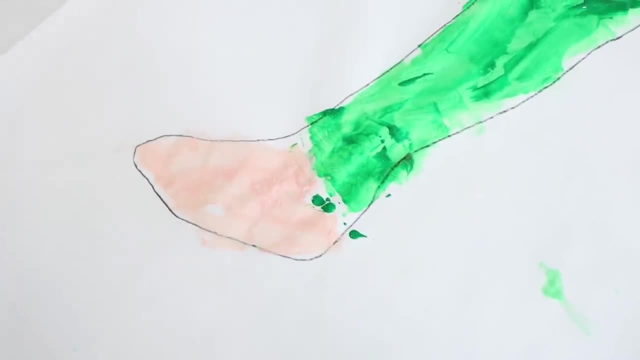 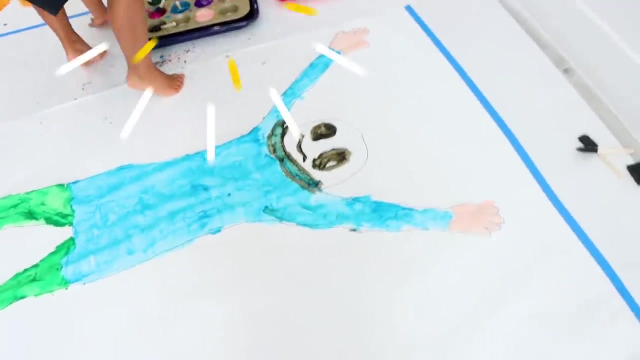 But you don't wear any shoes. No, okay, All right, Maybe you're staying at home. Look, there's green blobs right here. What do I do? It's okay. Whoa, whoa, whoa. you almost tripped. Ooh, that was close. Don't forget the hair too. 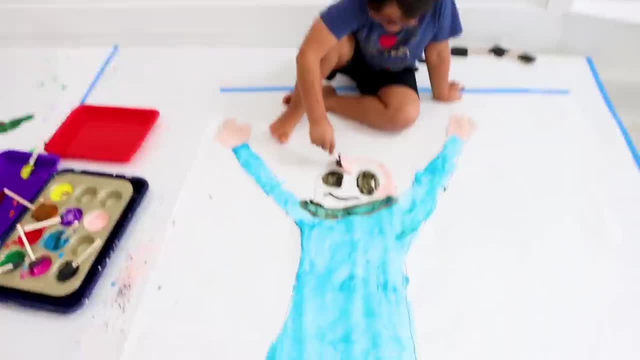 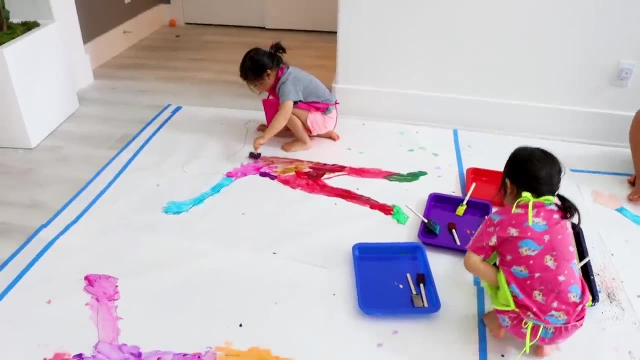 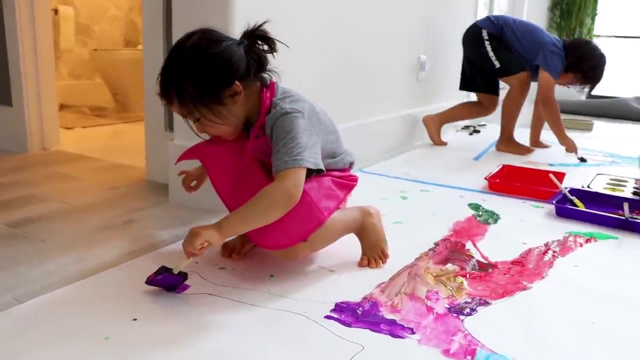 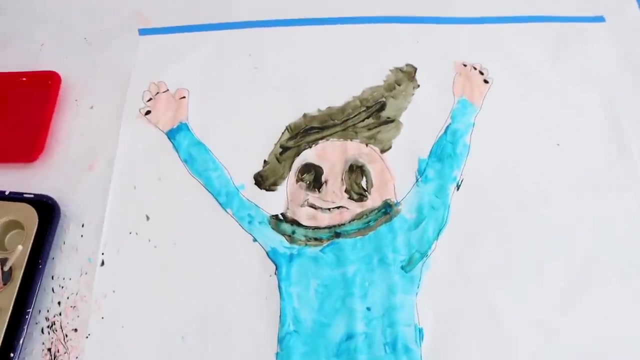 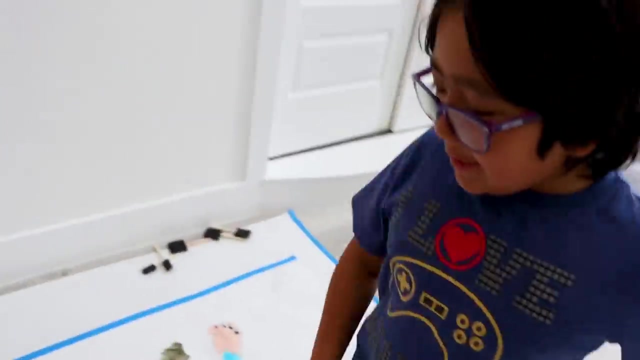 I Mean, if you want to, if you want to, who only This kind of looks cute, Cute? Oh, look at the face, and they're so focused. Okay, You like my hair? Oh, Round hair. Look at that, We're going one side. Okay, you have long hair like that, very spiky. 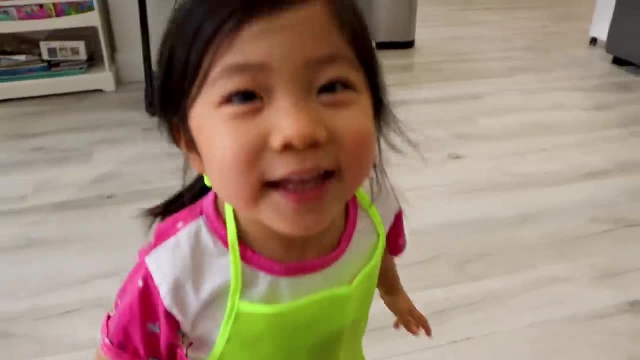 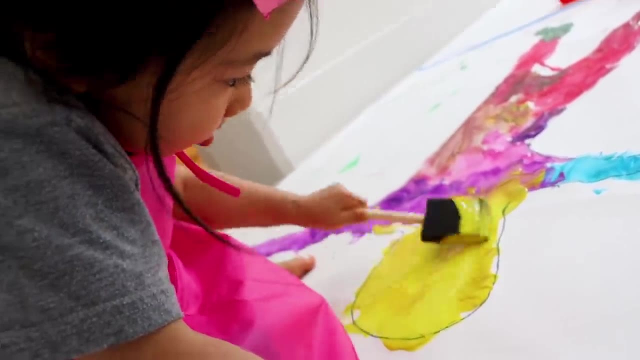 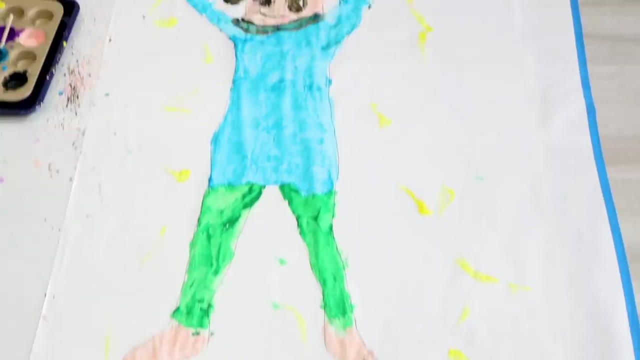 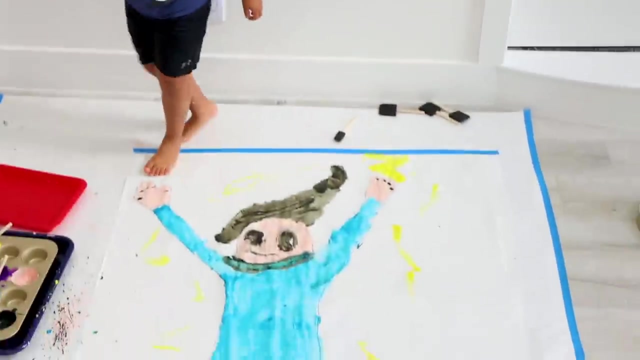 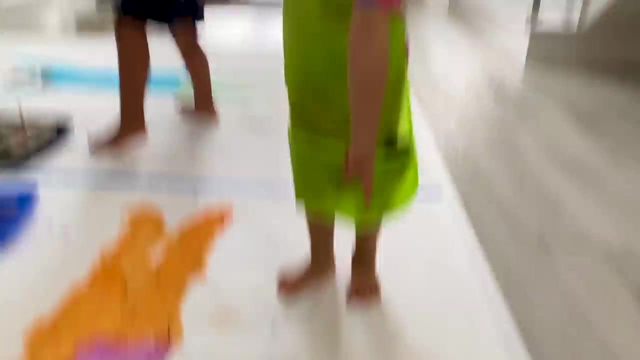 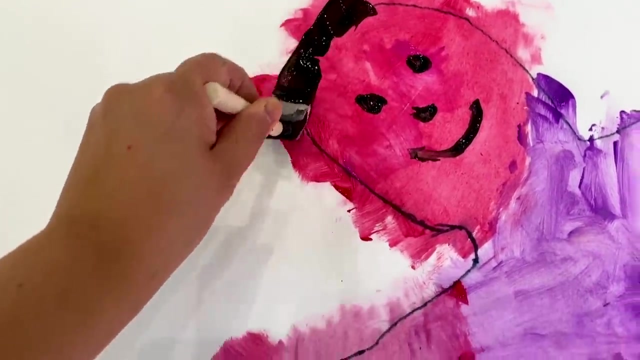 Okay, What Not done? Wow, Check Ryan's art. What is that? He's throwing something around like a yellow stuff. What is that? Oh, it's electricity itself. Whoa, so he has a super power, electricity power. Beautiful Emma's hair, Long hair, Emma. Wow, so long. 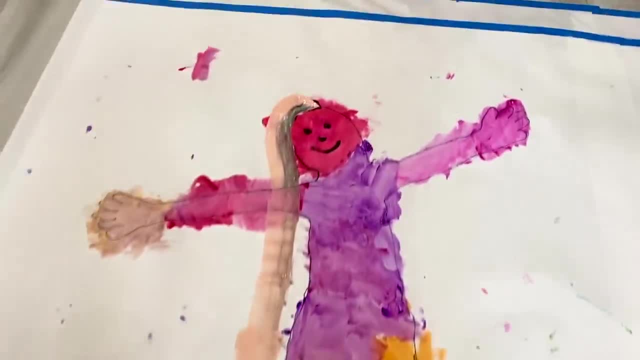 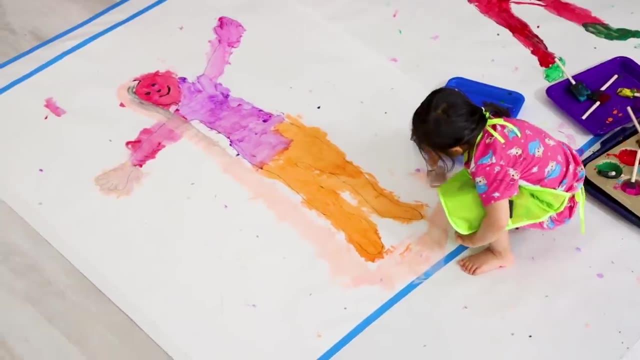 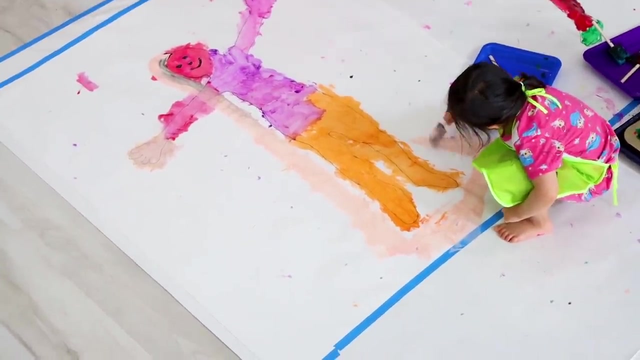 You're pretty. you look at this. Wow, Hi Kate. Wow, Look at Kate, That's beautiful. Whoa, look at Emma's hair- and she's not even done yet going all around. Look at Rapunzel. Okay, guys, I'm done now. 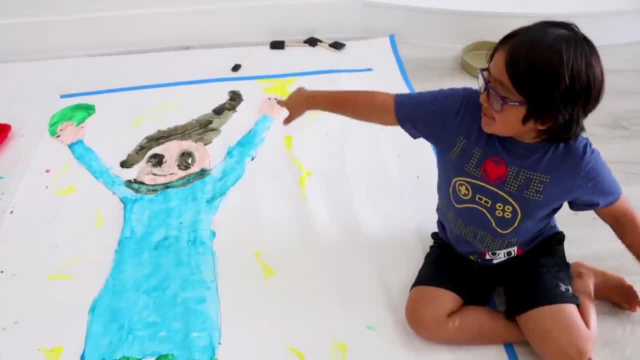 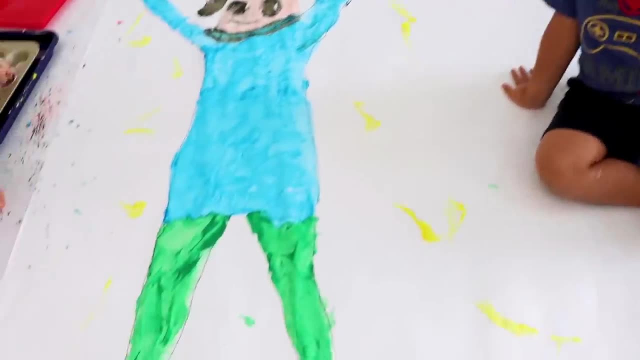 What do you guys think? That's supposed to be a lightning thing and that's supposed to be a plasma ball thingy. Oh, he's holding a plasma ball, Yeah, Nice. Good job, Ryan. Yeah, I'm making my hair super long. 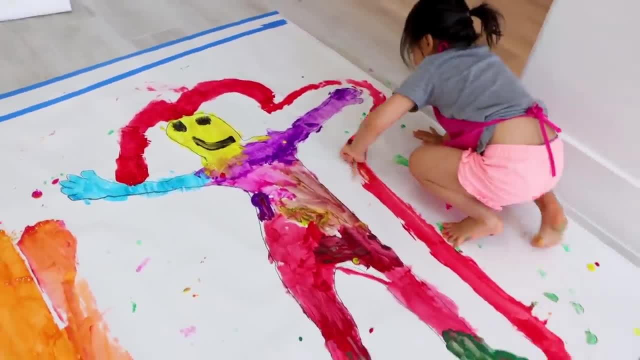 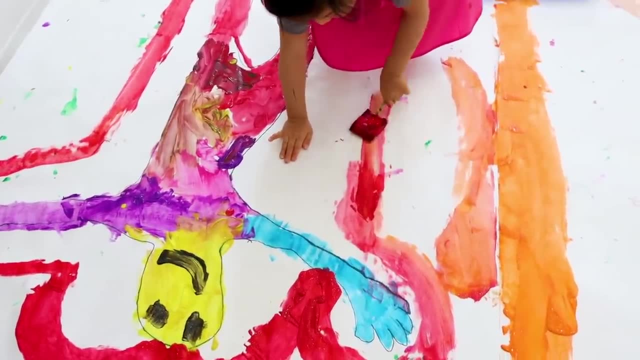 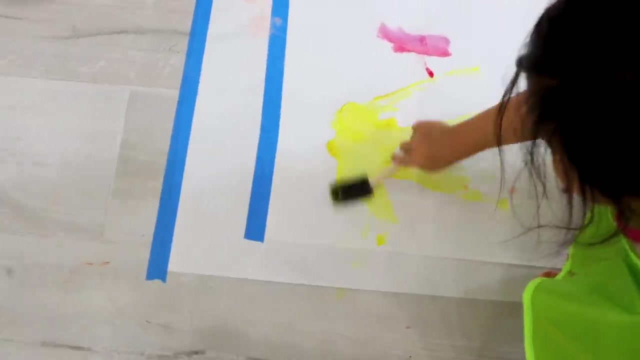 Oh, wow, okay, That's super long red hair. I love it. I'm going to put it in my freezer. It's beautiful. What are you making now? Emma Sun, Sun. Do you guys see Emma's sun? 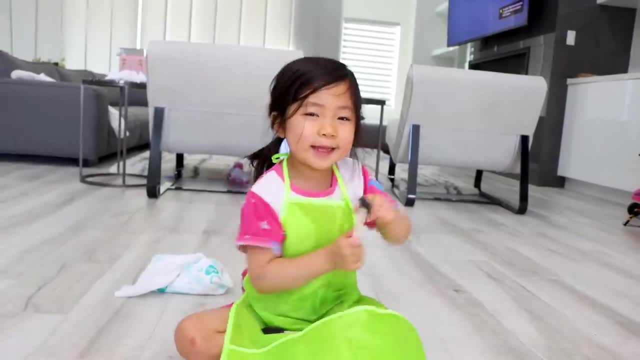 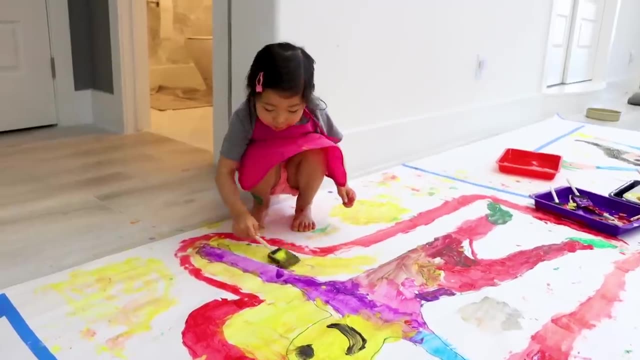 Good job, Emma. I'm done, You're done. Yes, Okay, so this is Emma's finished picture with the sun: Beautiful, I'm still working. Oh, wow, yeah, She's going to paint everything yellow, I think. 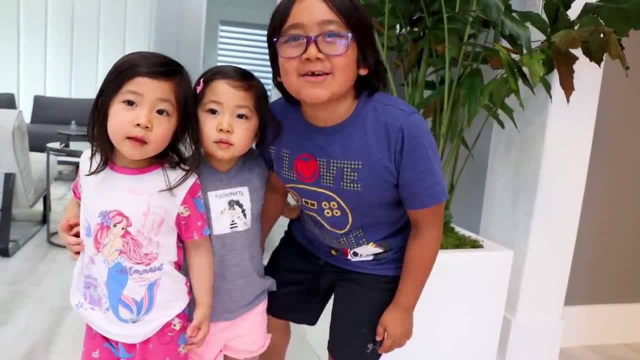 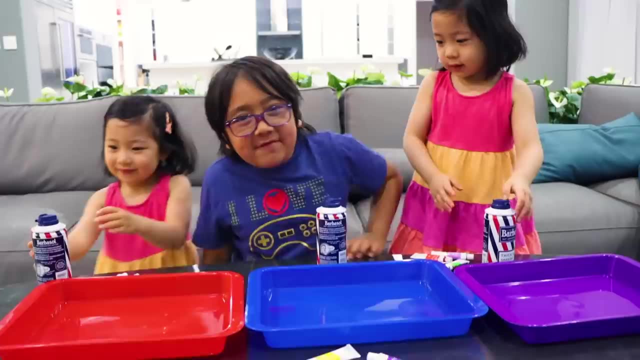 Beautiful. Okay, guys, thank you for watching our painting ourself video. Bye, Bye. Today we're doing shaving cream art First up, shaving cream, of course. Okay, let's put the shaving cream. I got it now, Mommy. 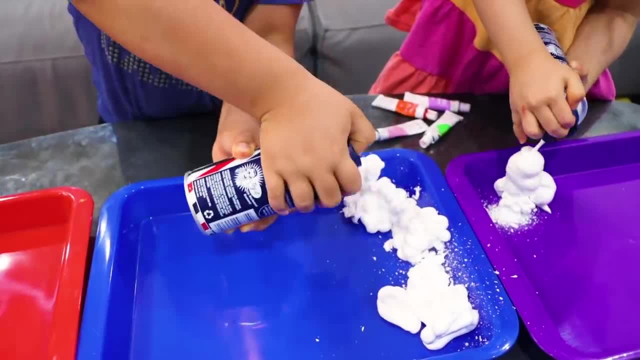 I got it. Whoa Emma, Look at Emma. Whoa, Ryan's doing it. Good job, Emma. Mommy, it's coming out. Yeah, you're doing great, Kate, You're doing great, You're doing great. 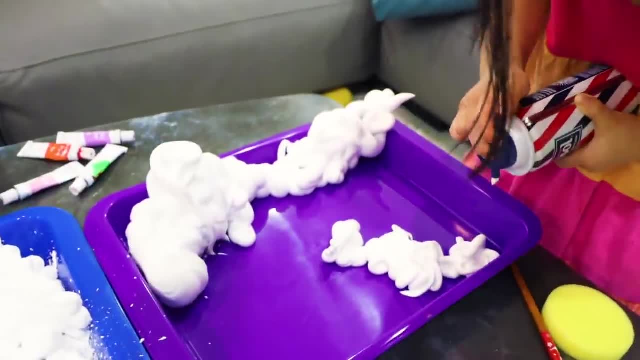 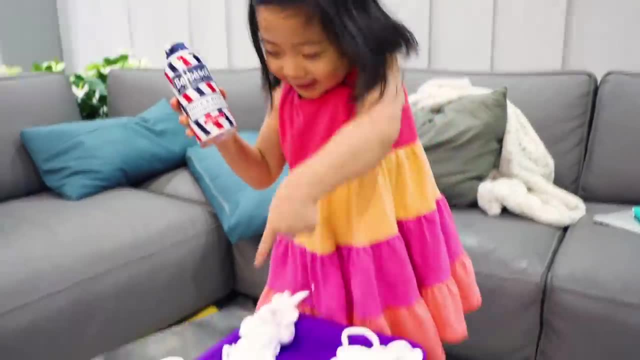 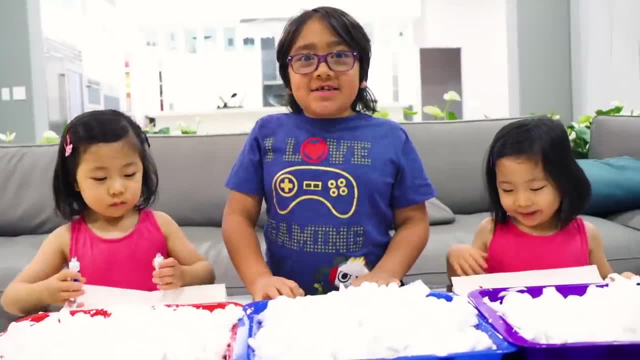 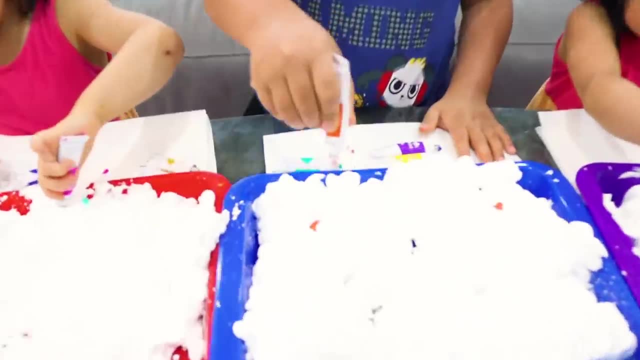 I want this one now. So next, use paint or food coloring and put it all around the shaving cream like that. Mm-hmm, We're using paint, but you can use food coloring, And if you don't have a tray like this, you can just use like a baking tray. 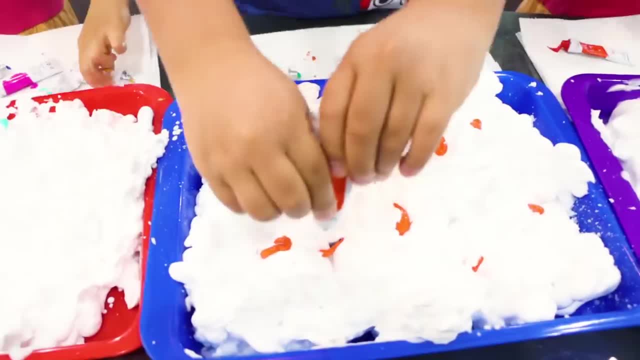 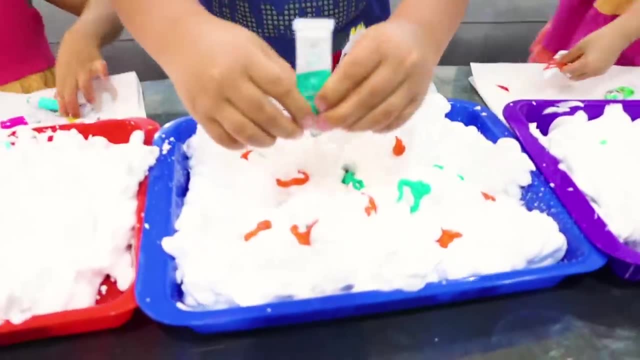 Okay, there you go. We're using a lot of paint from this acrylic paint set. Yeah, you can also use food coloring too. I told you I'm pretty like a bubble, like a magic wand. Okay, I'm done. 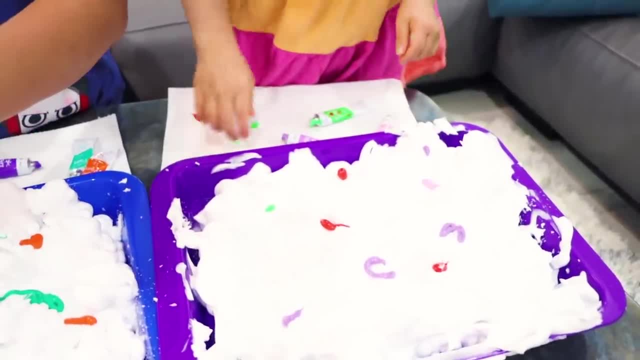 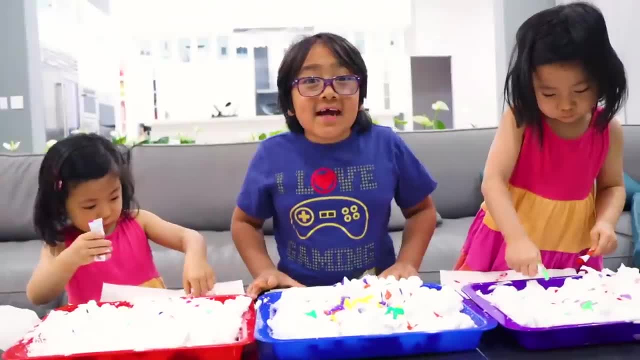 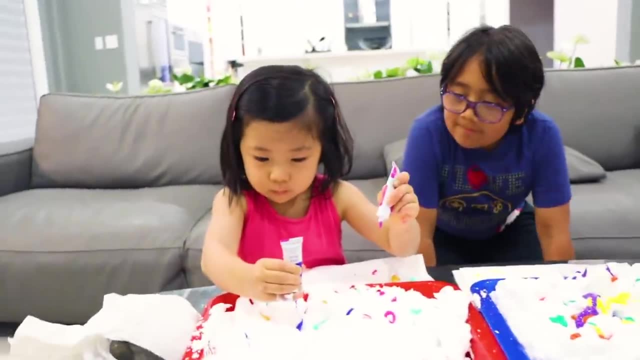 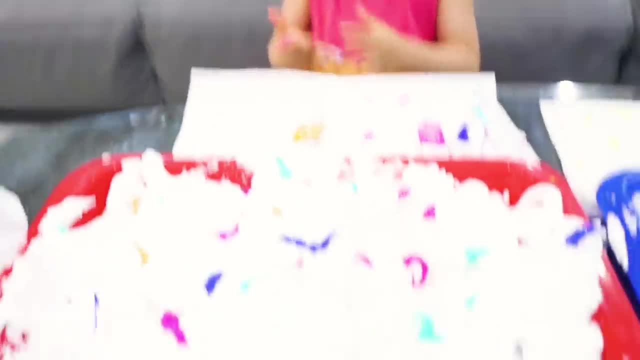 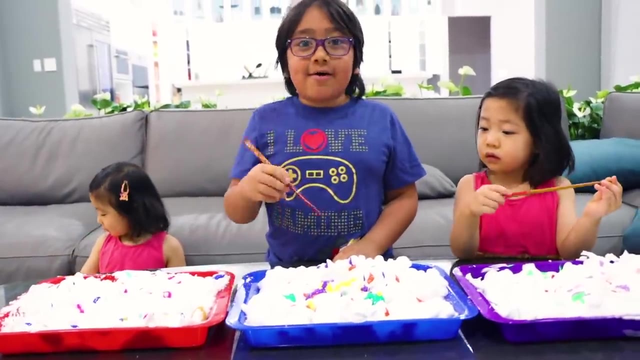 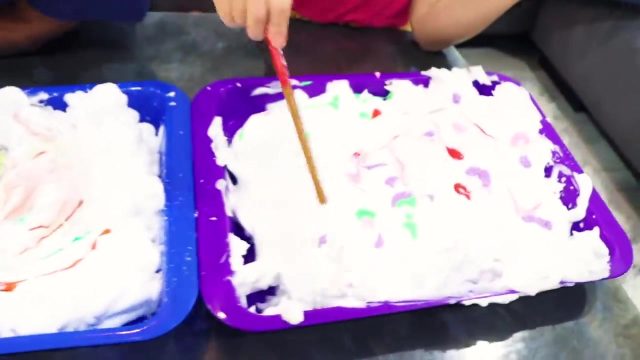 Let it drop. Okay, daddy, done It's pretty K Okay. so next you need a stick, chopstick or straw to mix it all up. Whoa, whoa. Good job K. So many colors together. 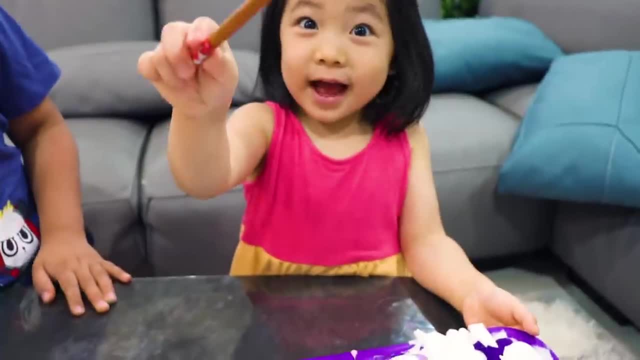 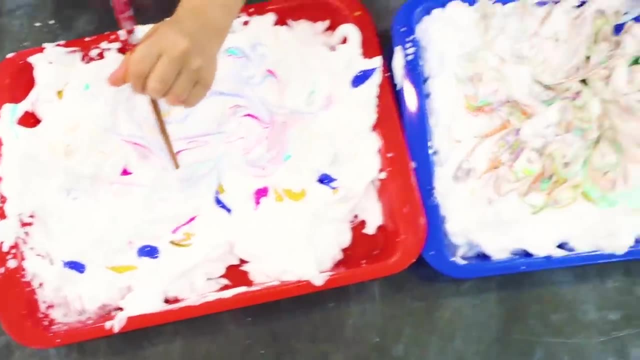 Yeah, No color's better. Looking great guys. Wow. Looking good Kate, Mm-hmm. Looking good Ryan Mine Looks like Christmas Mine's obviously super good, Good job. And then Kate's almost done. 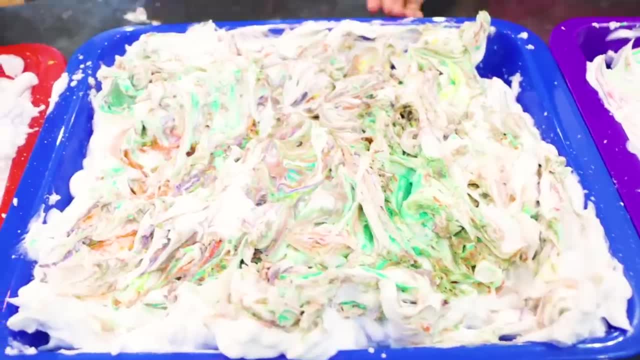 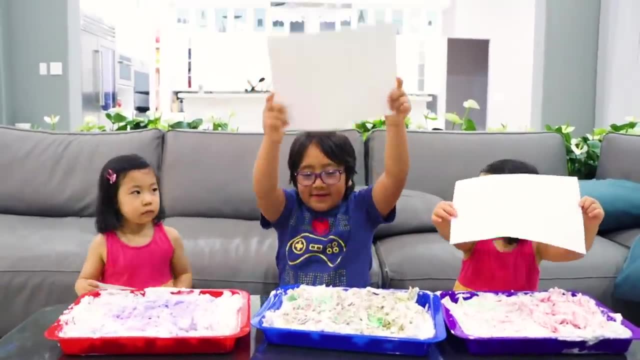 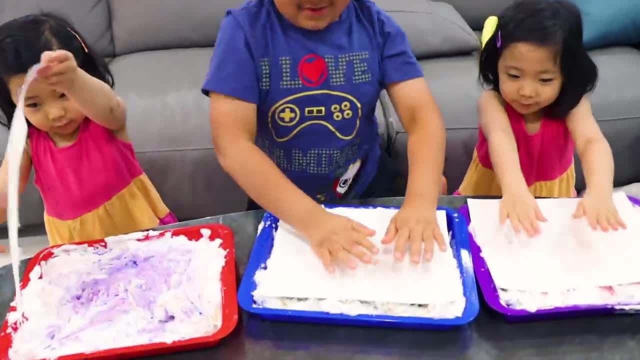 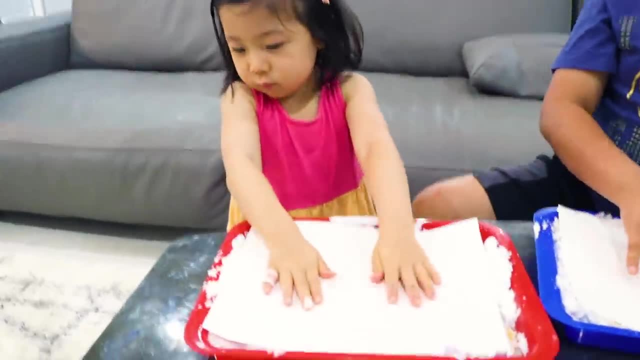 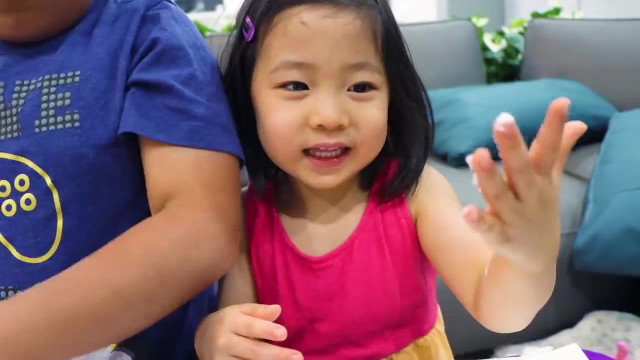 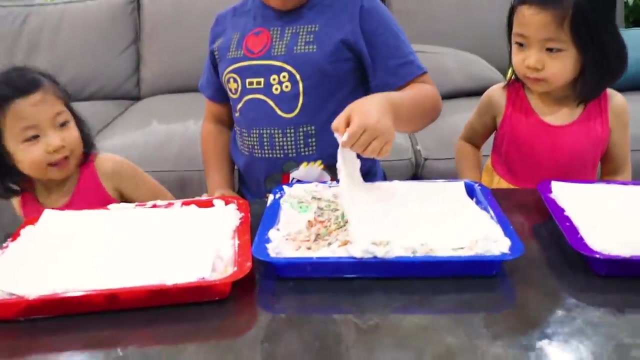 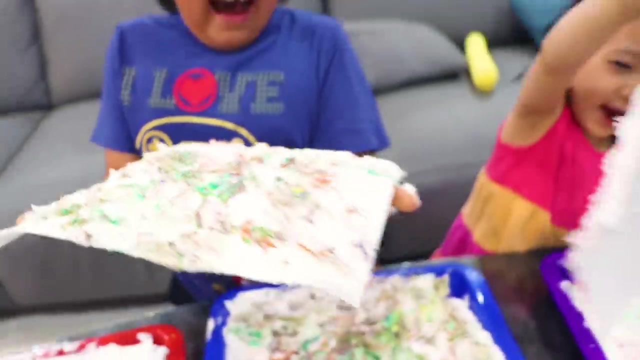 Okay, Okay, Okay, Okay, Okay, It's okay. it's just shaving cream. We can take it off, Uh-oh, Uh-oh. Next let's review our painting. Whoa, So this is Kate. This is Ryan. 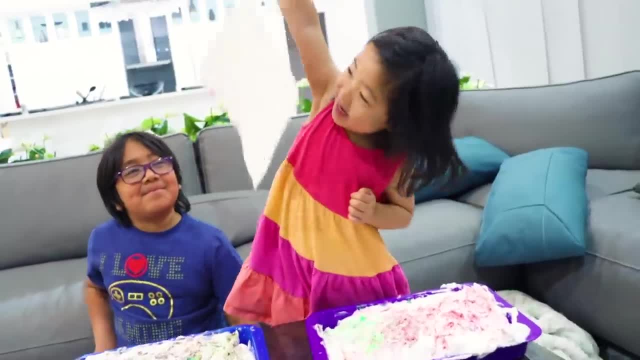 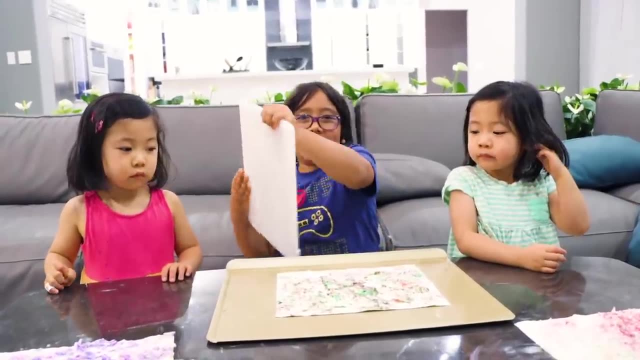 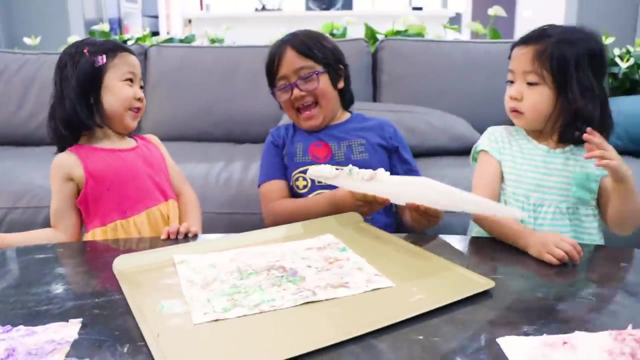 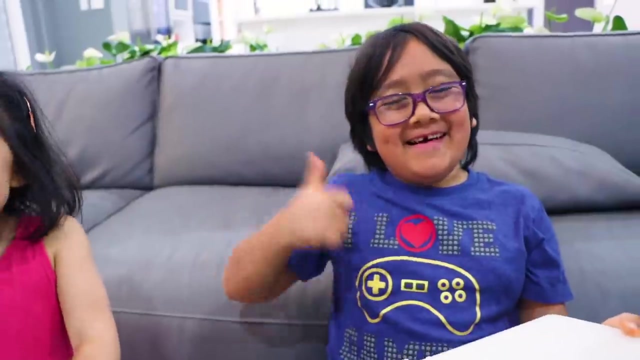 You very good and emma ryan saved it good job. okay, next let's shave off the shaving cream. there you go, just scrape it off. this looks beautiful. it's pretty good job. yeah, thumbs up from kate. yes, beautiful, every art is pretty. so that's ryan's art. there looks really good. 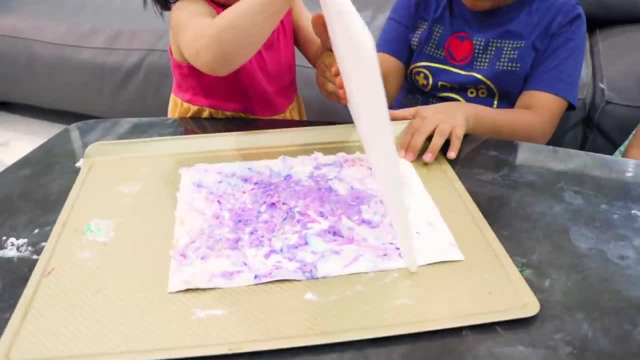 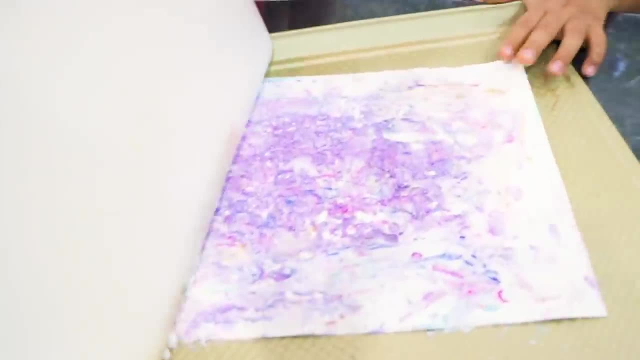 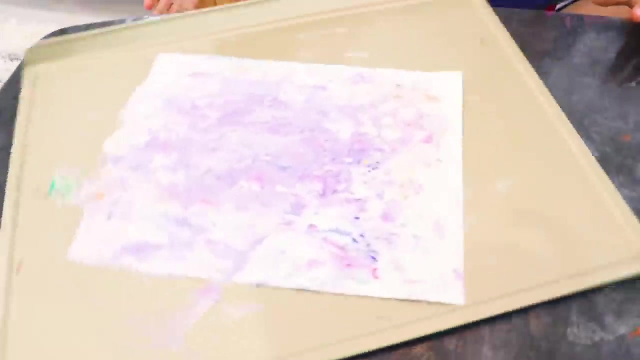 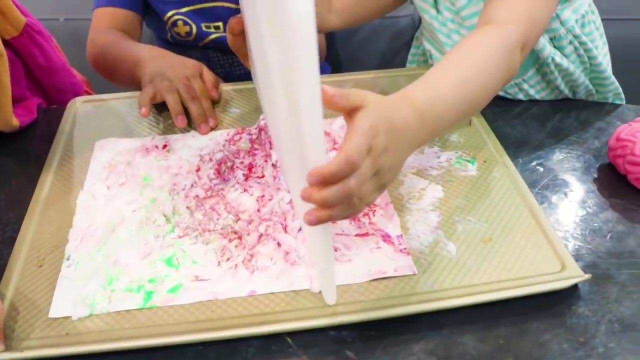 it's my turn. okay, ryan's gonna help easier with a ruler, but we couldn't find one, so not scraping there you go. beautiful, wow, that's pretty, yeah, pretty, okay, it's emma's turn. again would be very helpful with the ruler. we're doing great. 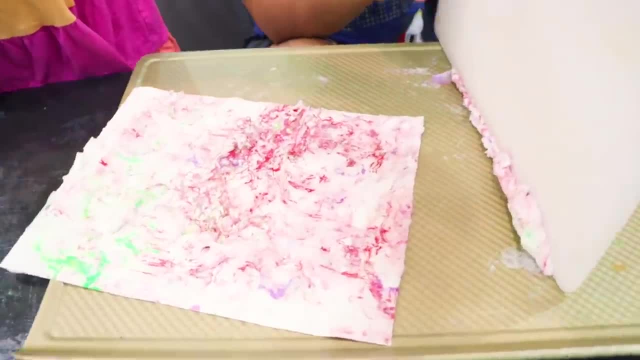 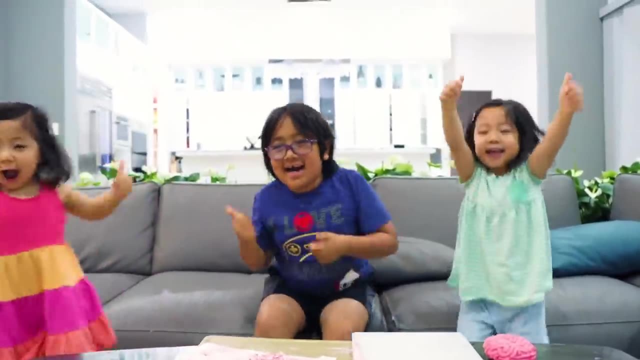 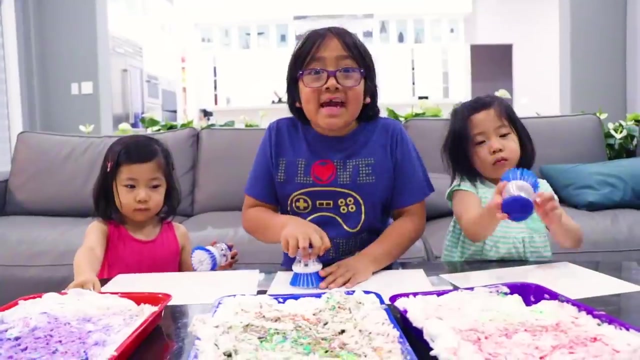 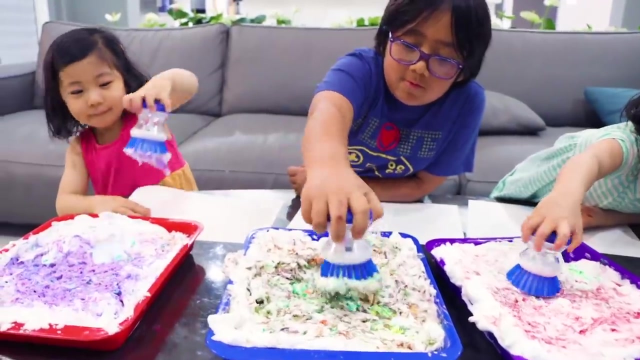 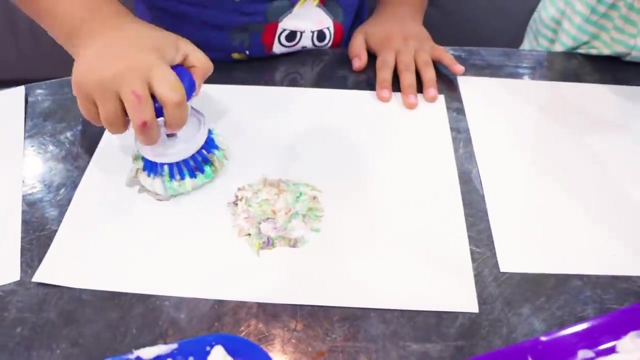 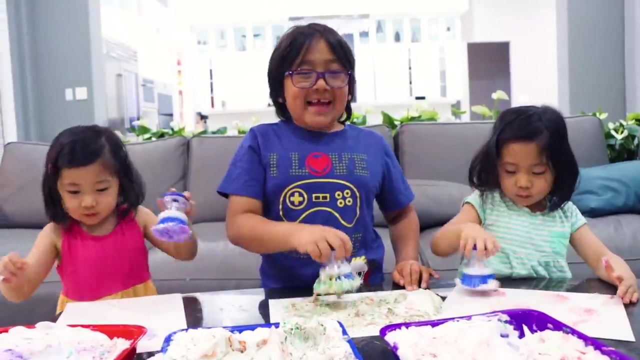 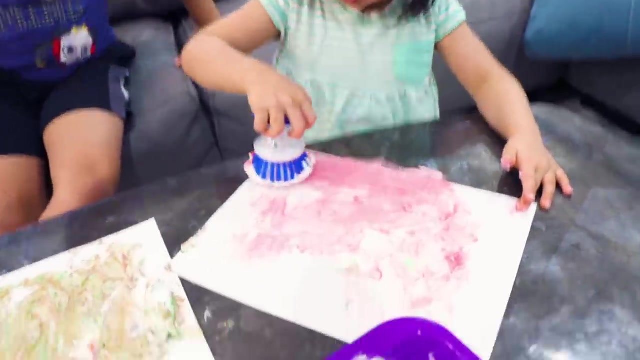 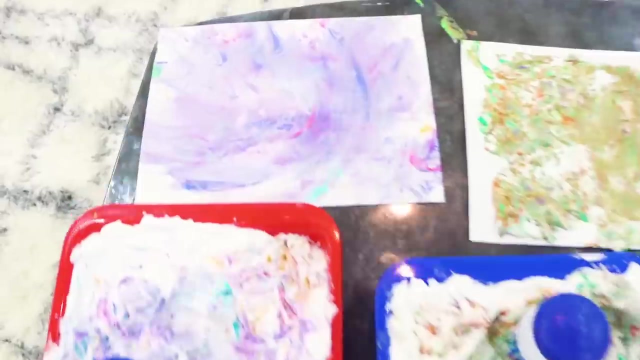 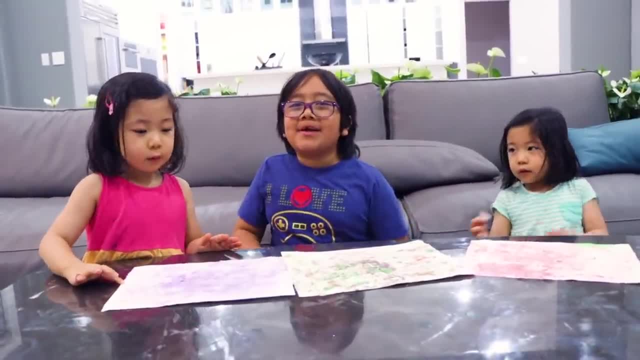 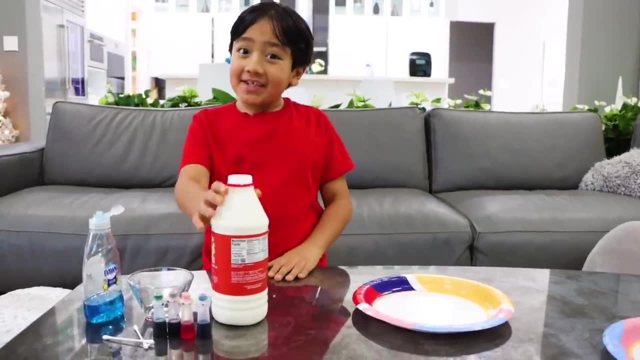 like our shaving cream art. We'll see you next time in another video. Hey guys, today we're doing the milk and soap experiment and a little bit of food coloring, So obviously you'll need some milk, some soap and food coloring. 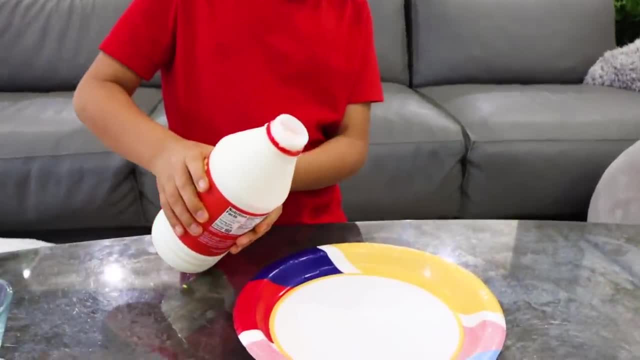 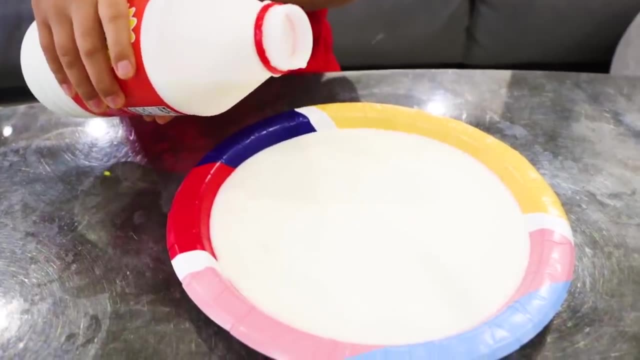 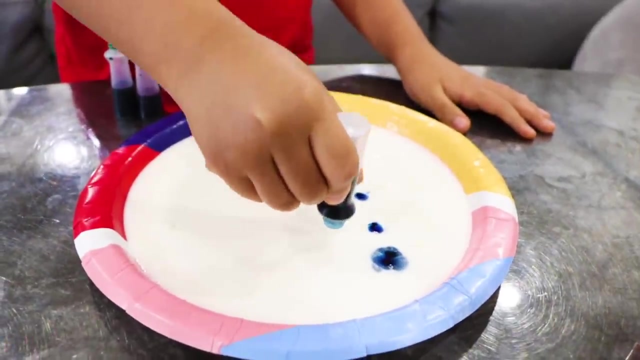 Whole milk works best. So you have a plate and then you pour the milk into the plate. up to about here. Then put your soap into the container. Next, be creative and put some food coloring all over. I'm trying to write high with blue.